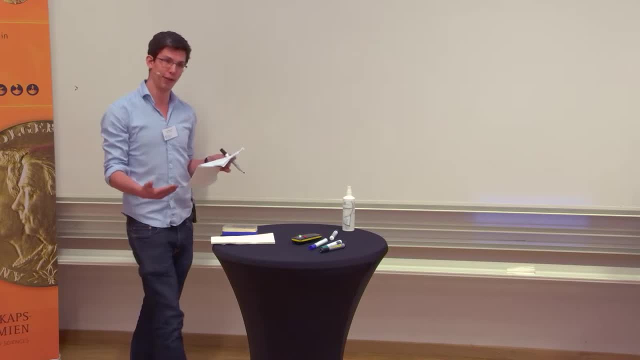 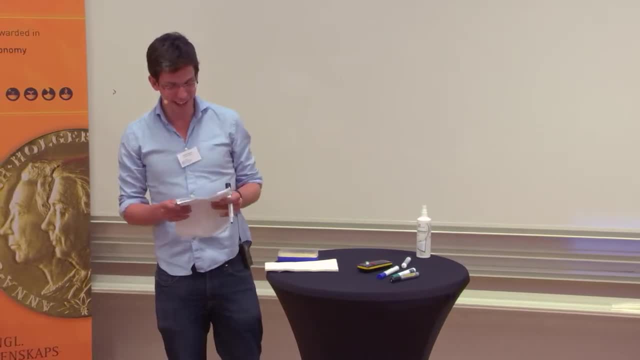 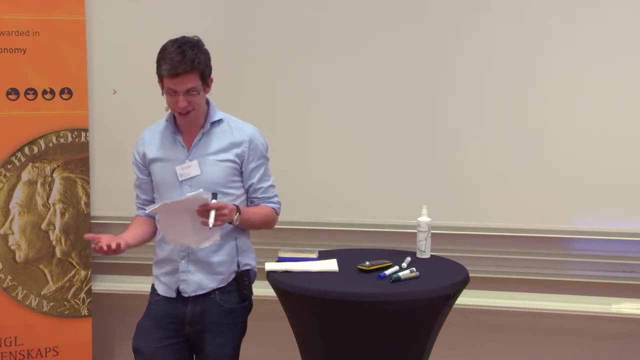 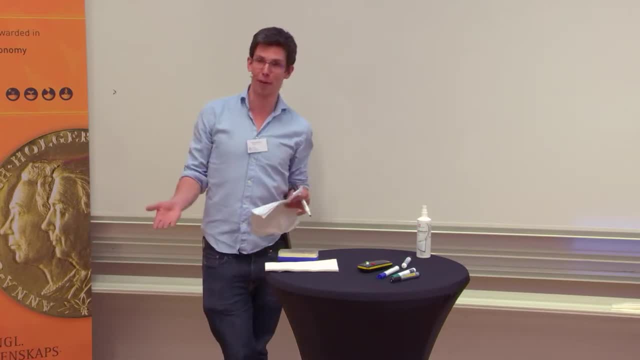 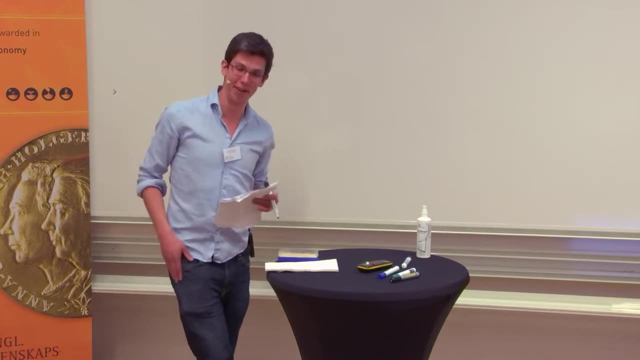 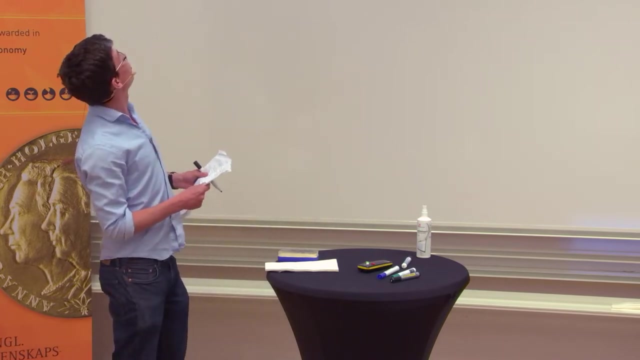 and they always refer to me, to him, to me- as the fun one. So I'm sure my parents are very pleased that you've won the prize as the fun one. Okay, so I would like to talk about Primes and Athmeta, Progressions and Civs. 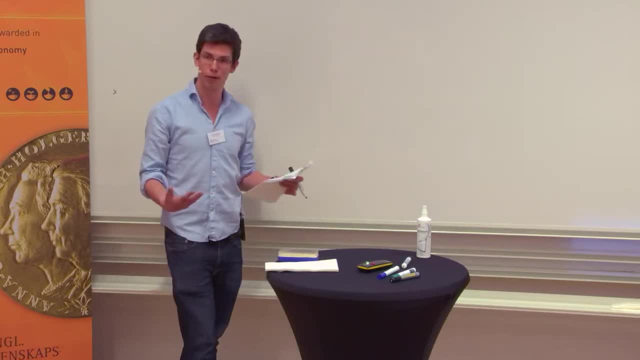 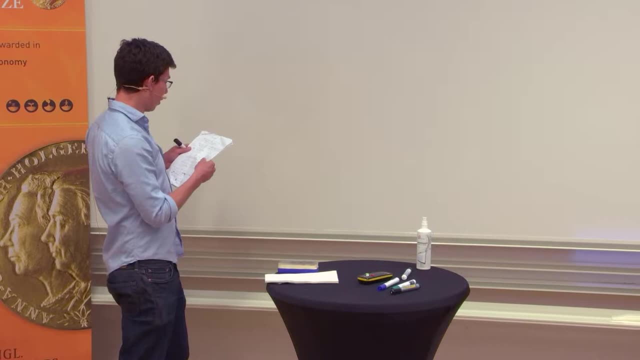 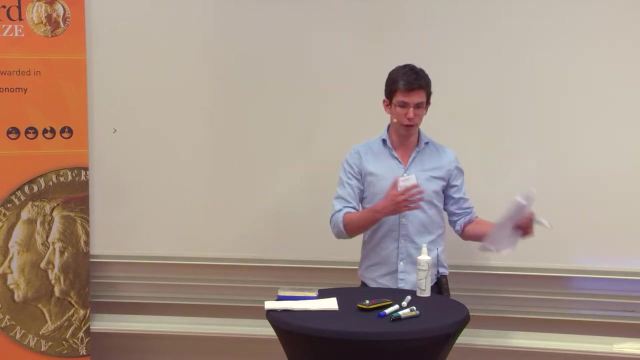 Just as a general thing, this is intended to be a colloquium-style talk, so I'm hoping that this is accessible, but please do ask questions if things aren't clear, And I'd like to not try and be at all comprehensive in terms of talking about Enrico Bombeiro's work. 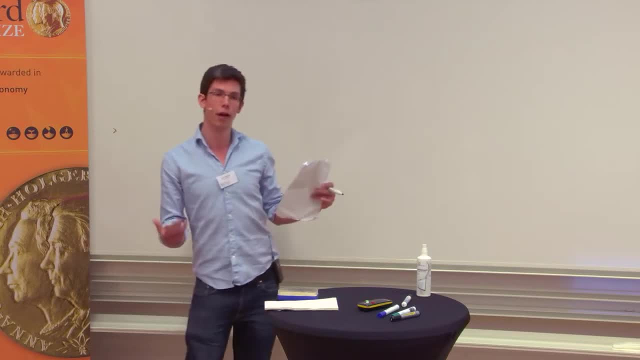 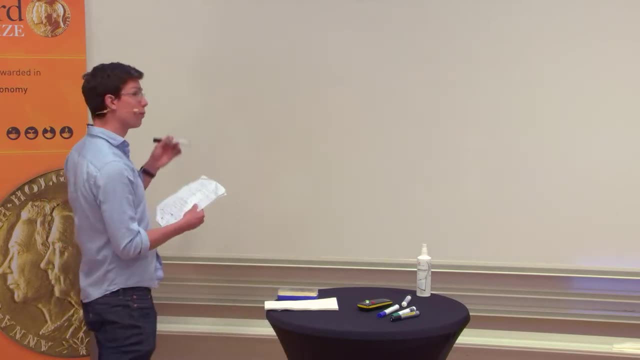 but maybe just focus on a couple of his favorite results and how they fit into my research and how they relate to me. So it's a slightly personal take and some of Enrico's work is what I'd like to focus on today, But maybe I'll start off with the Riemann Hypothesis. 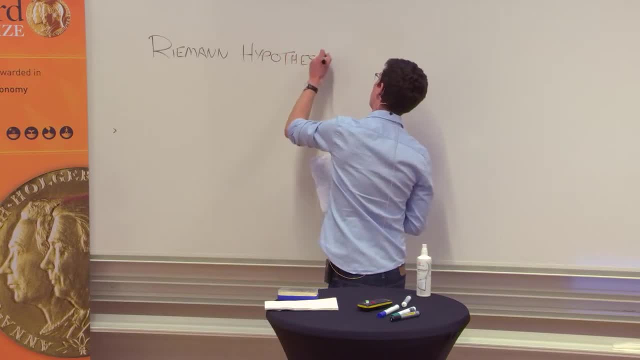 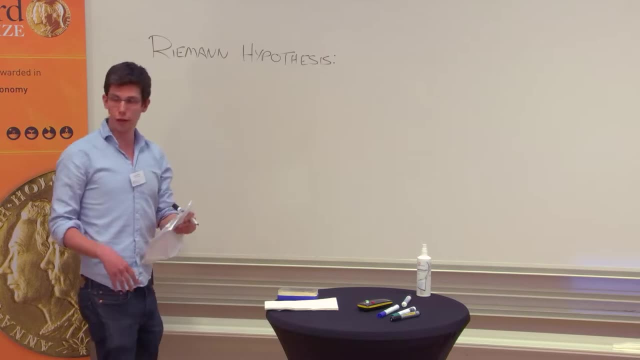 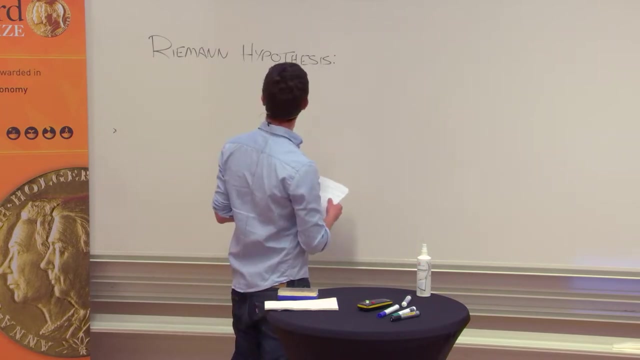 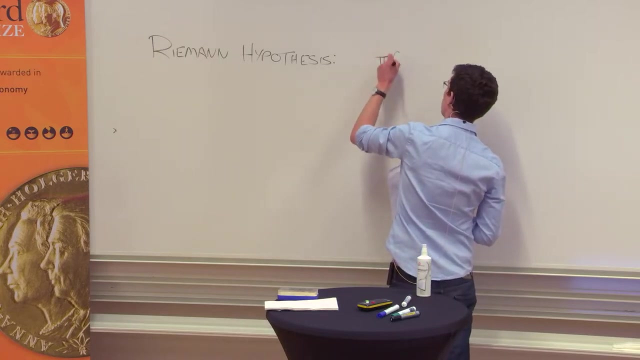 So we've already seen this a little bit in Enrico's talk. So this is normally stated as the non-trivial zeros of the Riemann zeta function all lie on this special line, with real part equal to one-half, But maybe a slightly more low-level way. 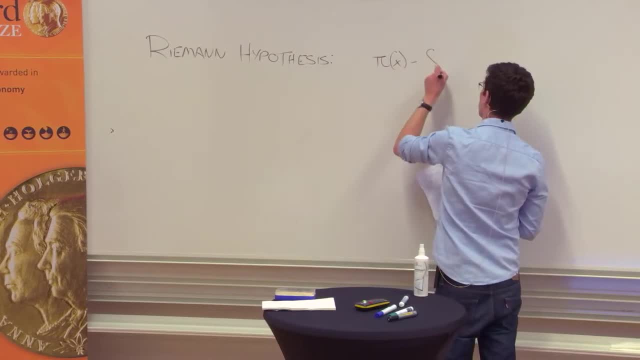 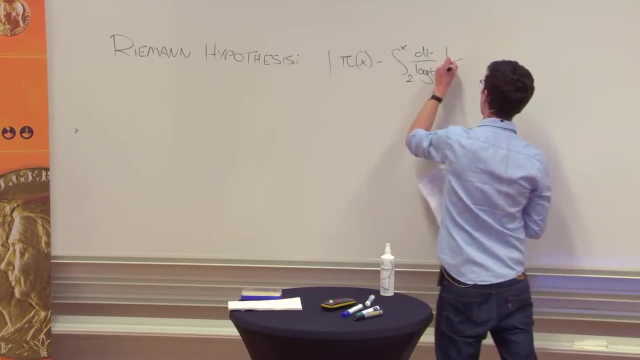 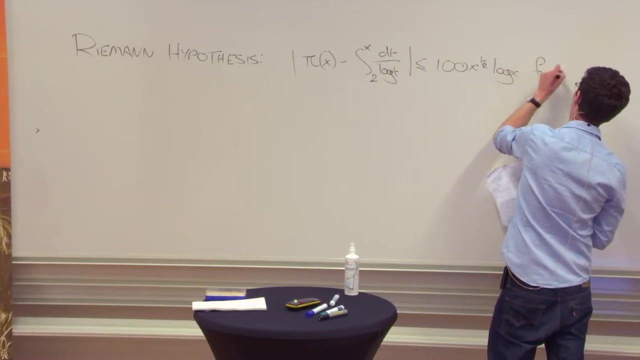 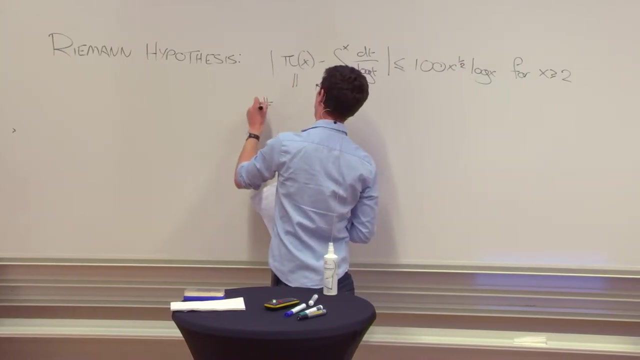 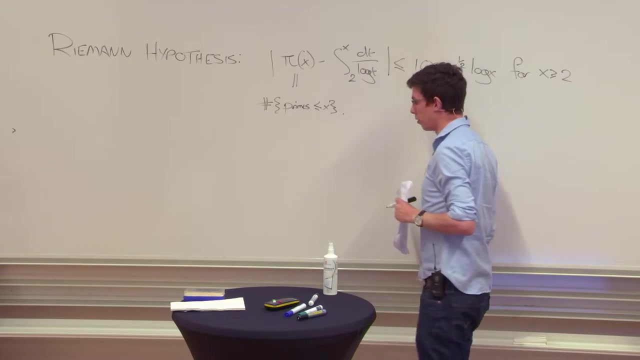 of stating the Riemann Hypothesis is just as an inequality, Where here, what I've written as pi of x is just the number of primes which are less than or equal to x. So this is a completely equivalent form of the Riemann Hypothesis. 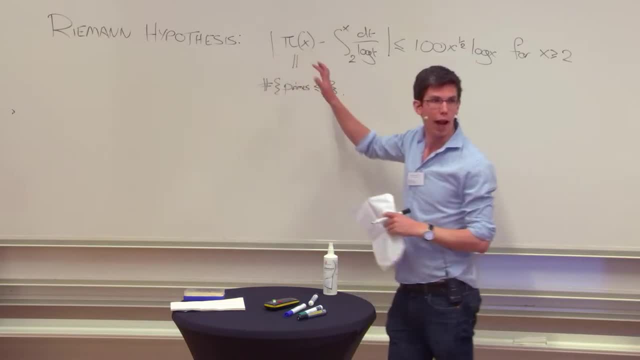 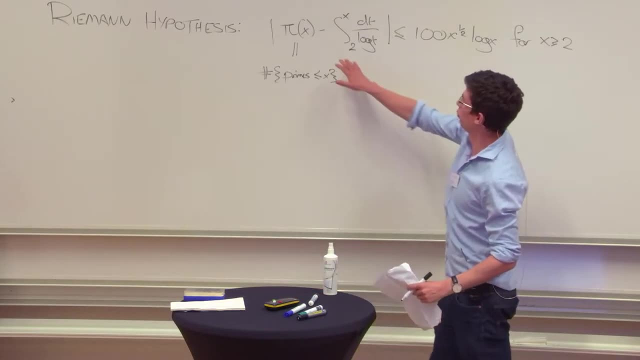 and there's this complicated object which, as an analytic number theorist, we are very interested in understanding: the number of primes up to x. And what this says is that the number of primes up to x is very well approximated by some simple, smooth analytic function. 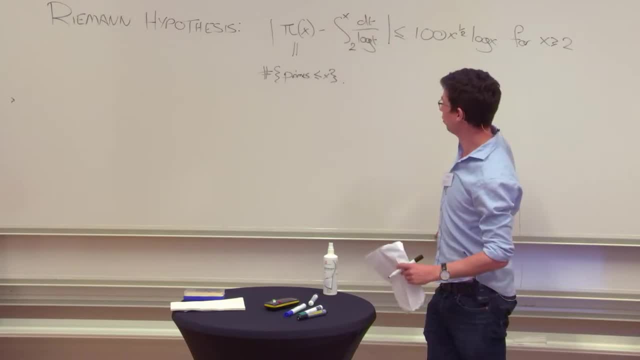 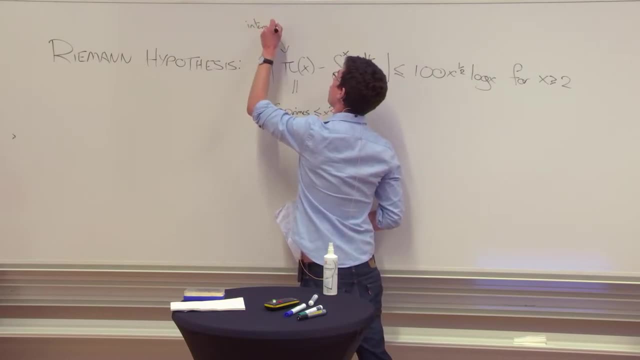 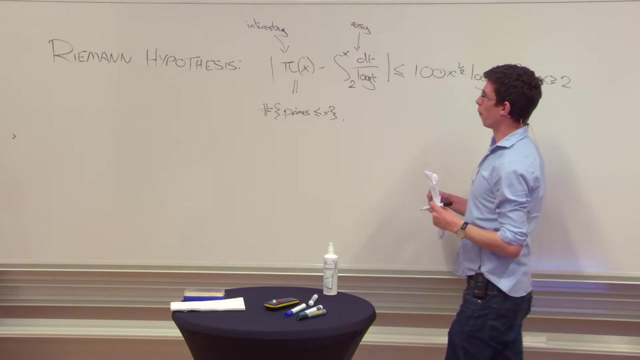 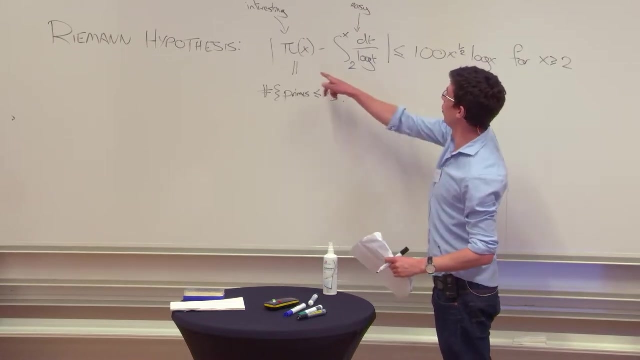 which we should think of as being this: integral is easy. So maybe this is interesting, but complicated. This is kind of easy and well understood, But obviously this is a step function that jumps by one whenever x gets to a prime number, so it's certainly not equal to some nice, easy, smooth analytic function. 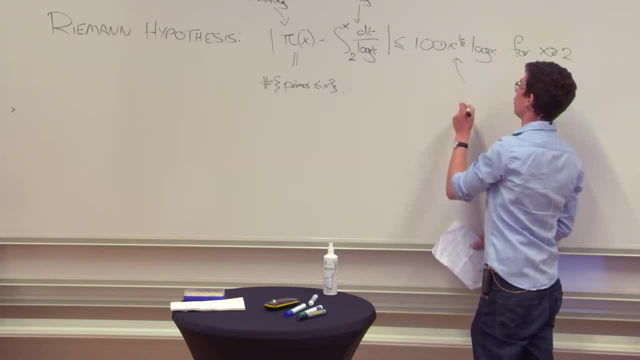 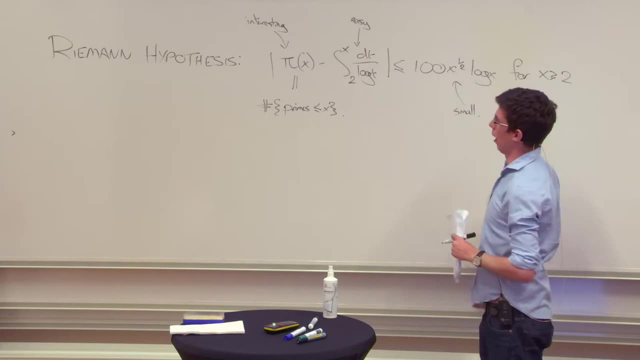 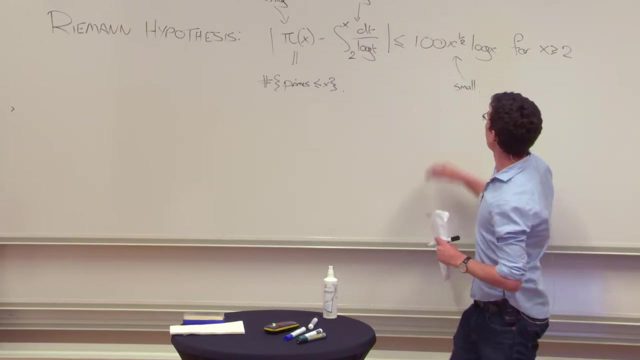 So it's only equal to this, up to some error, And the Riemann Hypothesis is stating that the error in this approximation is very small. So when x is very large, this approximation will have size about x over log x and this error term will have size slightly bigger than the square root of x. 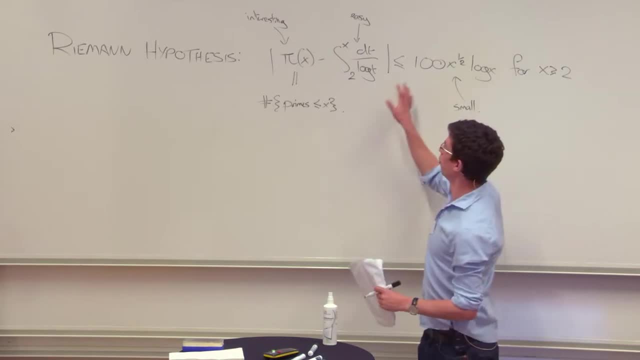 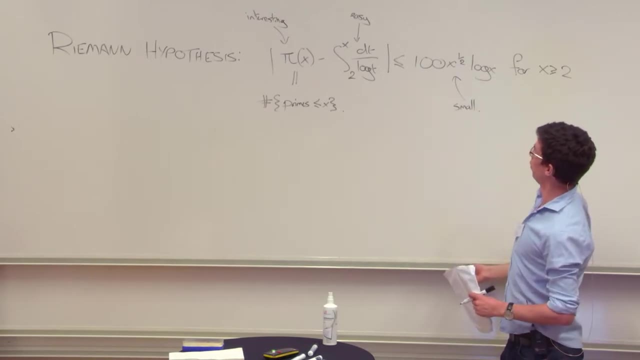 And so it will be of size roughly the square root of the main term, And so this is going to have maybe half the digits of the main term approximation. so this is really somehow a very good approximation. The constant 100 here is completely unimportant. 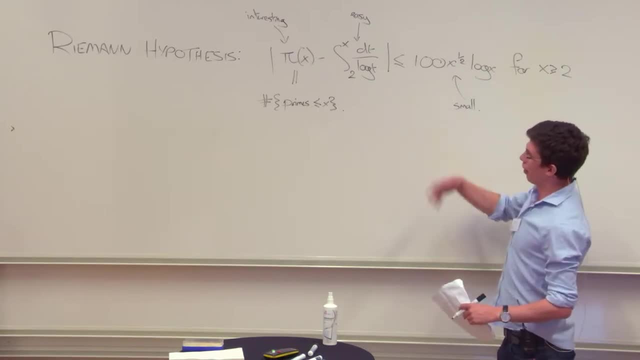 It's just some constant, although there's a lot of structure going on here, and so there's this sort of fun fact that there's a self-improving constant. So if you prove this with a constant 1000, you can also then replace it with a constant 100.. 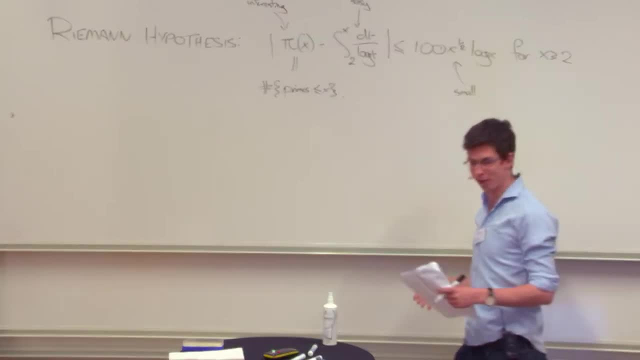 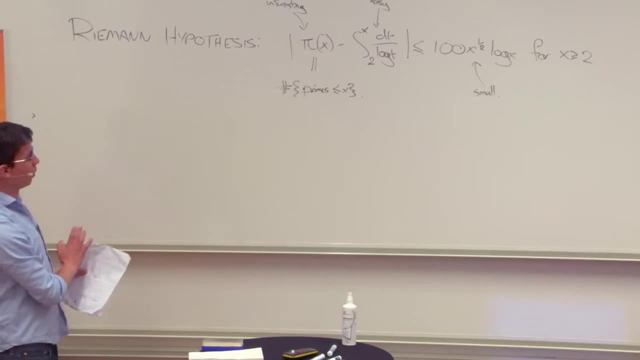 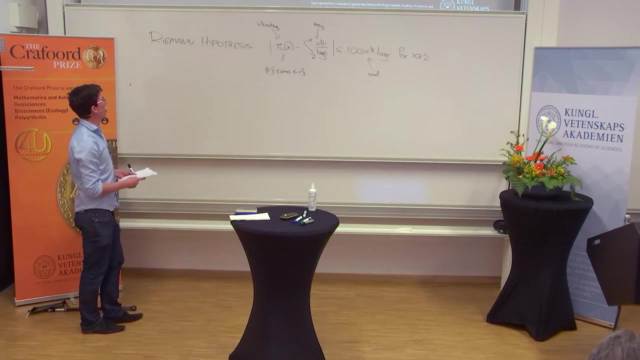 And in fact you can replace 100 with some smaller constant that depends on the zeros. Okay, So this is the Riemann Hypothesis. You get a million dollars if you solve it. It's often dubbed the most important open problem in mathematics. 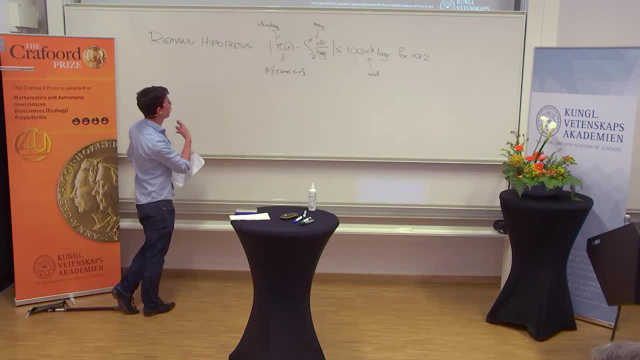 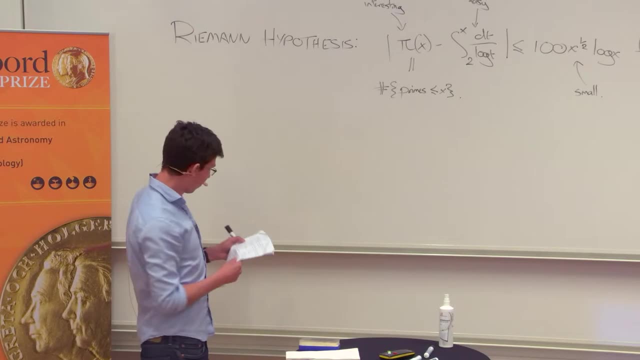 But often for lots of consequences for prime numbers. it turns out that a slight generalization of the Riemann Hypothesis is the sort of really key thing for further applications, And so maybe I'll call this rh and then grh will be the generalized Riemann Hypothesis. 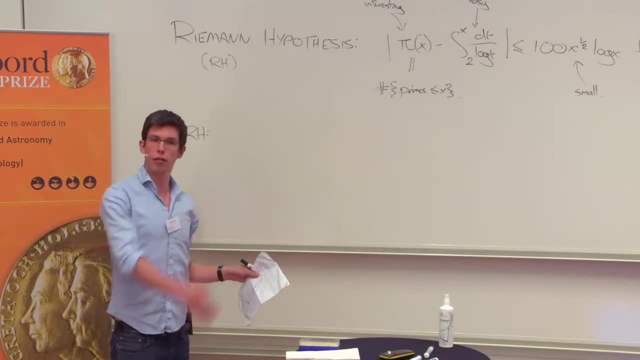 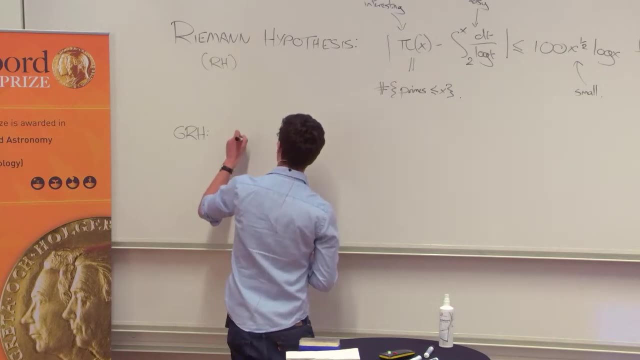 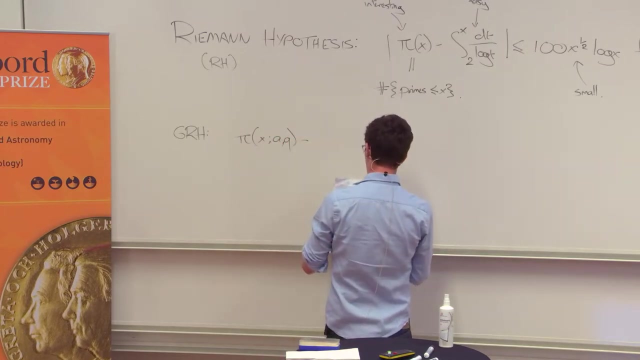 And again this can be formulated as zeros of certain L functions all lining up on special lines. but maybe a more down-to-earth way of writing this is that the number is a counting estimate for the number of primes in arithmetic progressions and having a very good approximation again. 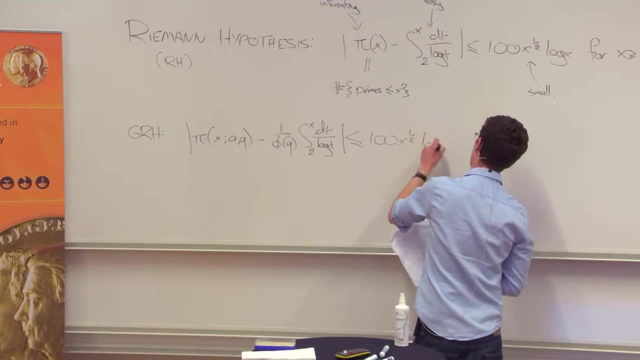 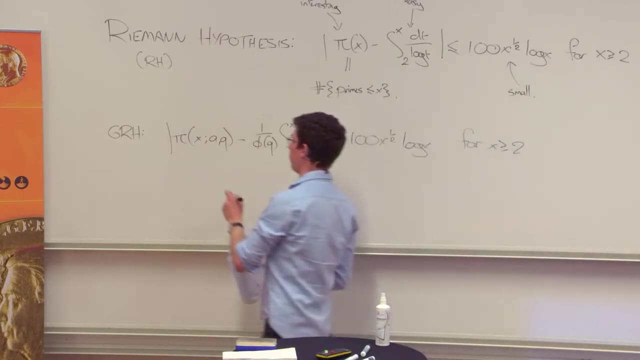 So I'm hopefully writing it in a way that will look somewhat similar to the phrasing of the Riemann Hypothesis, where here this is not just counting the number of primes up to x, but the number of primes up to x which are: 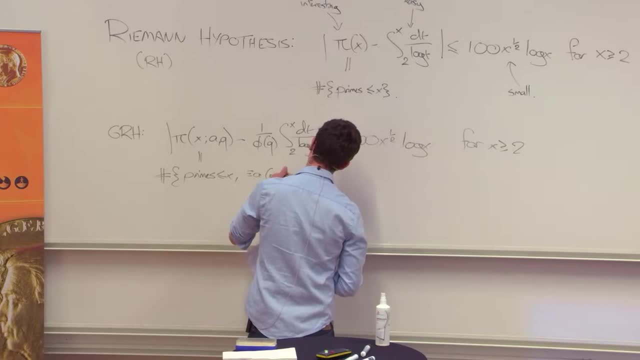 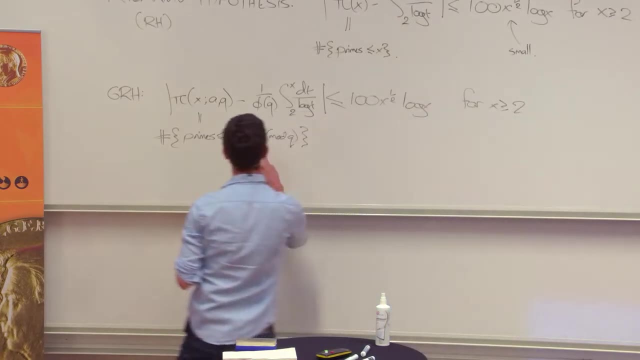 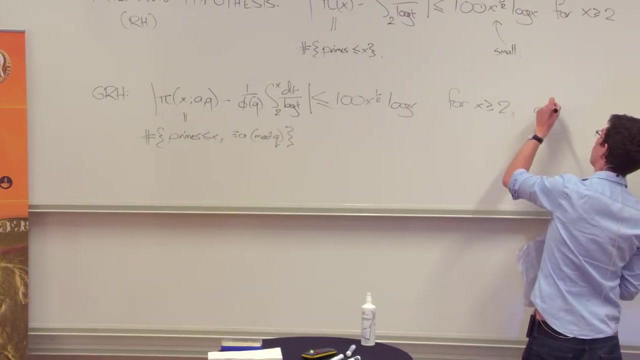 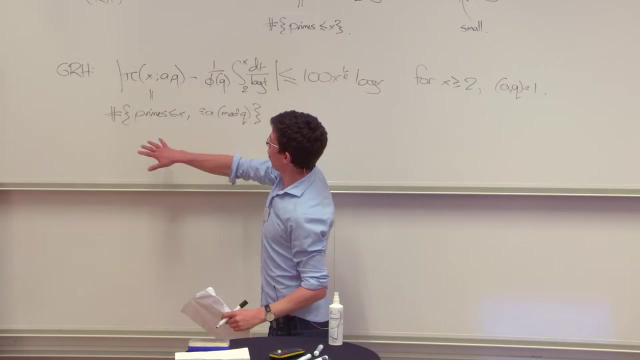 congruent to a modulo q, And this is obviously going to be false if a and q have a common factor. So this is for x being bigger than or equal to 2, and a and q being two co-prime integers. And so, again, this is saying that, if you're interested, 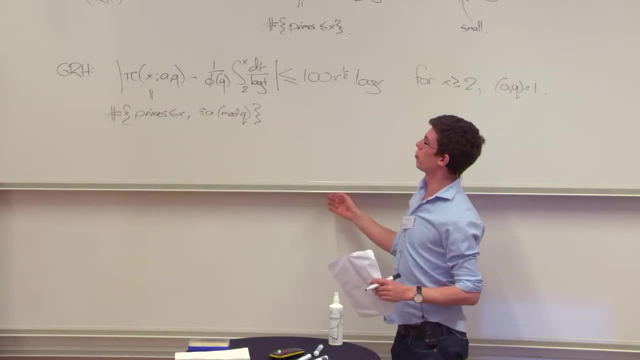 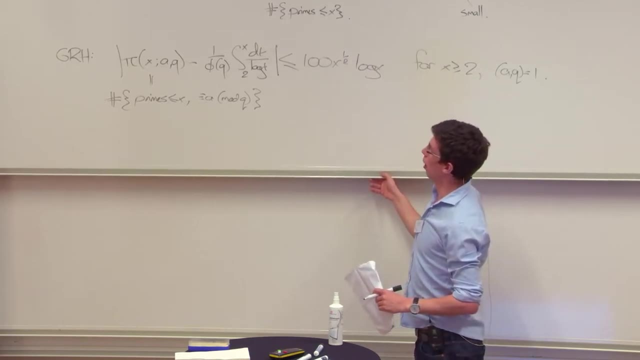 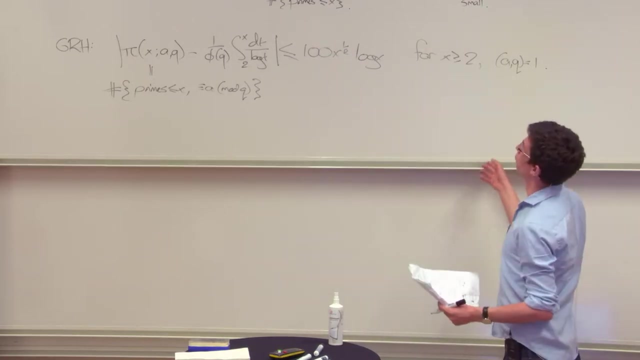 in the number of primes up to x in any given residue class. this has a very simple main term, approximation, and then some small error term. And this is just a reformulation of this question about the zeros of certain L functions And I guess, maybe one comment on that front. 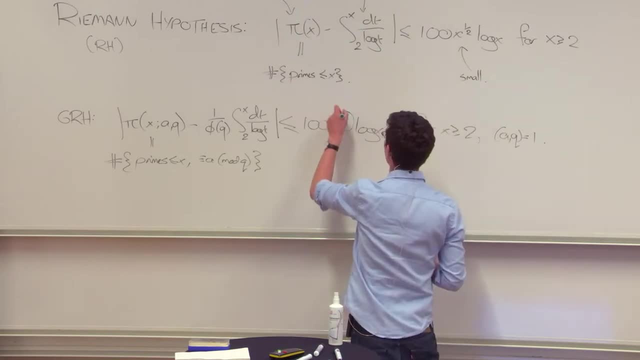 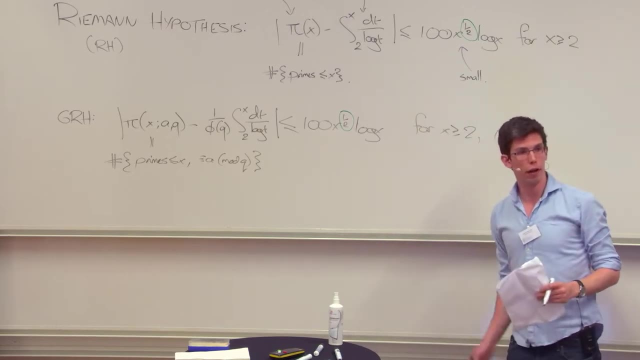 is. I'll just highlight this exponent 1 half here as being very much related to the line with real part 1 half If you could prove a weak version of the Riemann Hypothesis that all the zeros of the Riemann zeta function. 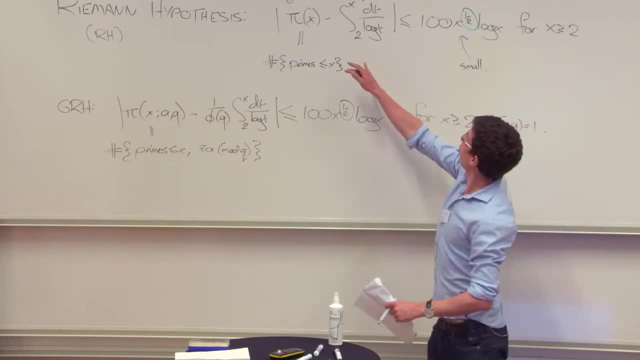 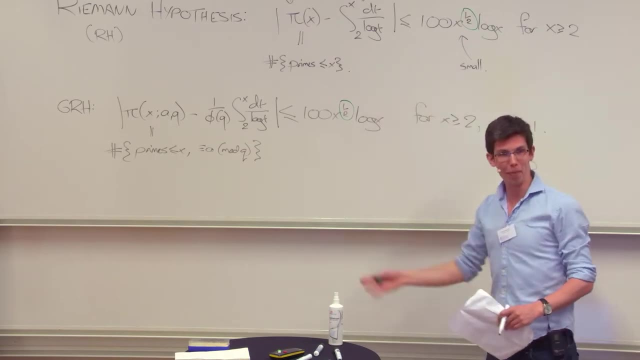 had real part, at most 3 quarters, then you get a statement very much along these lines, but with 1 half replaced by 3 quarters as a bound, And so it would be a weaker statement, but it would still be an amazing breakthrough. 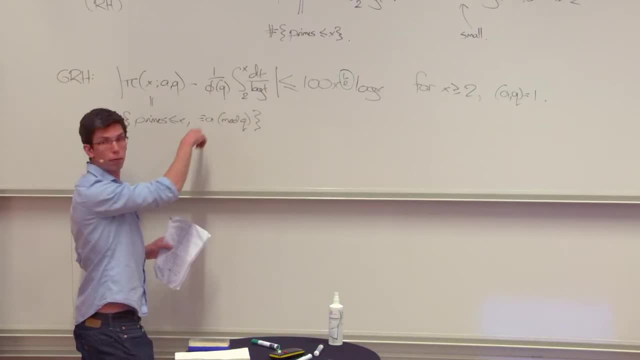 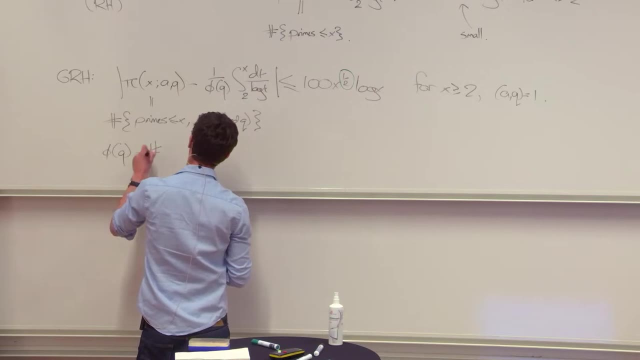 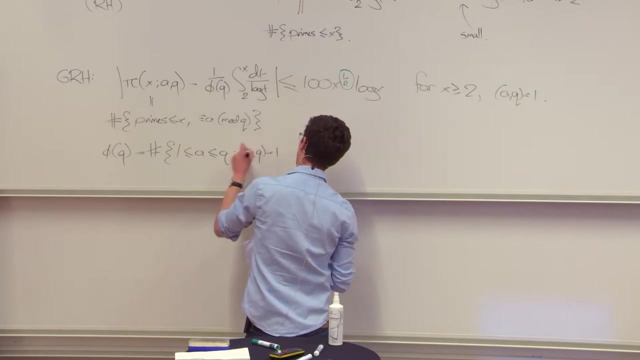 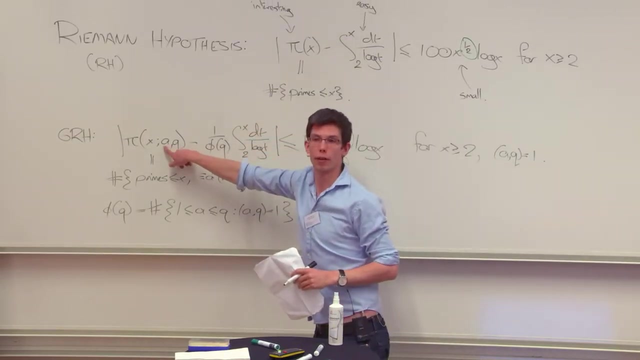 Fine here. yeah, sorry, this is the number of possible co-prime residue classes. So this is the Euler phi function. So this is saying this main term approximation doesn't depend on the residue class A, apart from the restriction that A is co-prime to Q. 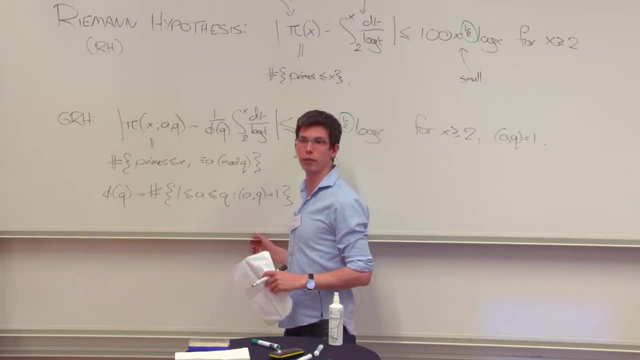 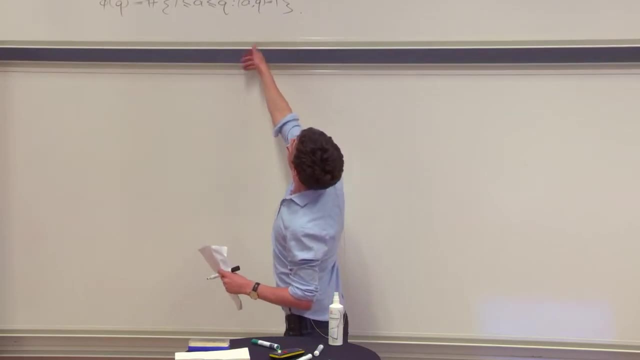 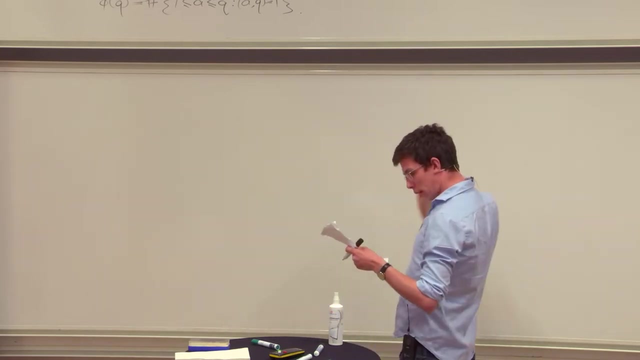 And so this is saying that every one of those different residue classes gets roughly the same number of co-primes. Maybe we could turn off the Oh great, thanks, Okay. Unfortunately we don't know how to solve the Riemann Hypothesis. 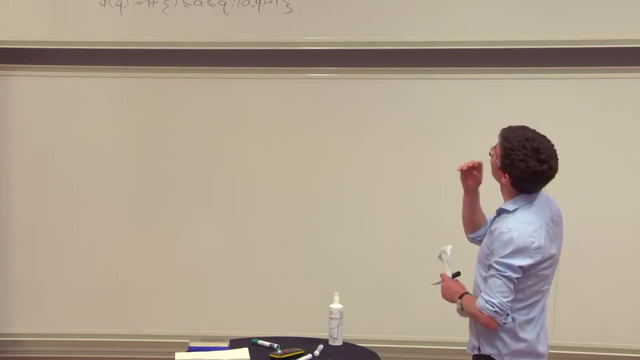 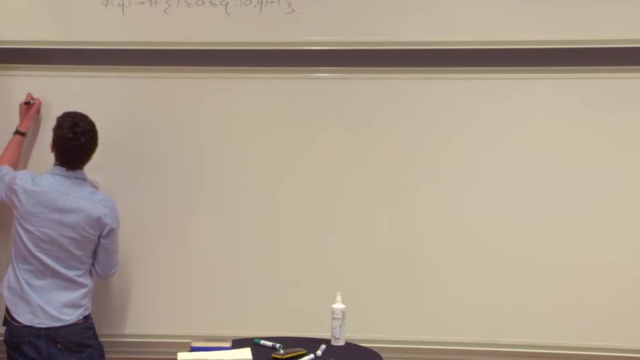 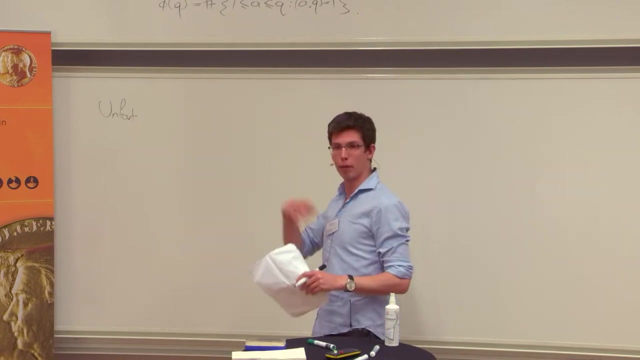 and we don't know how to solve the generalized Riemann Hypothesis, and this is a fairly major barrier to making progress And the We can't even get one of these weak results where we replace 1 half by some other constant. 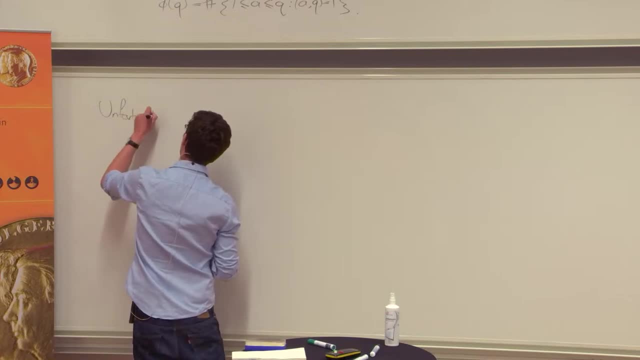 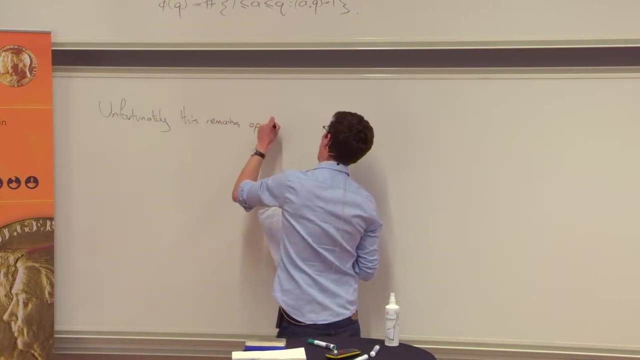 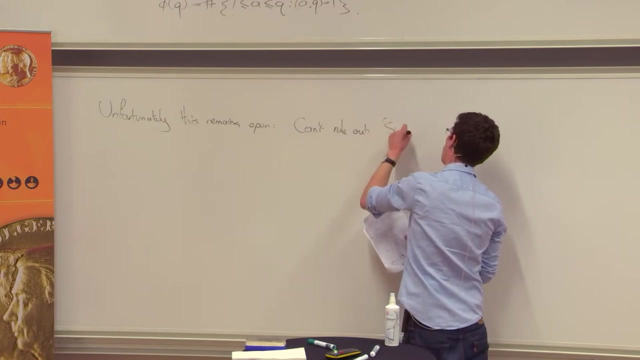 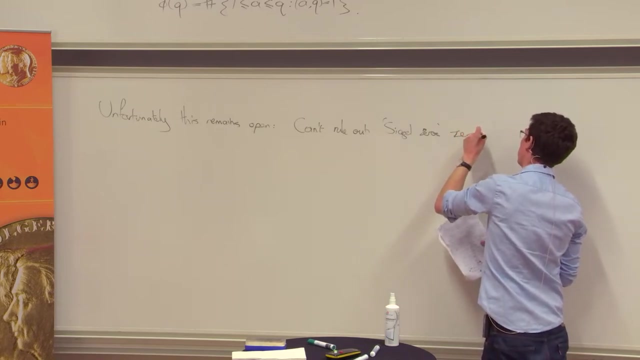 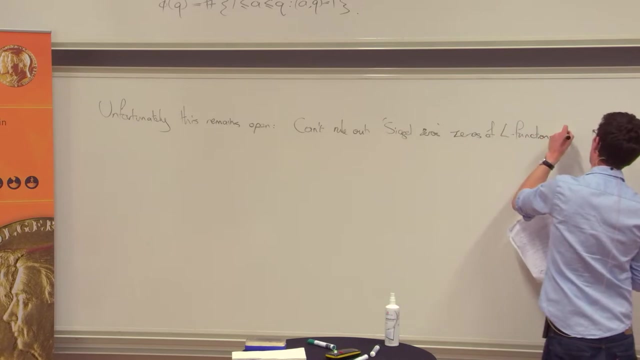 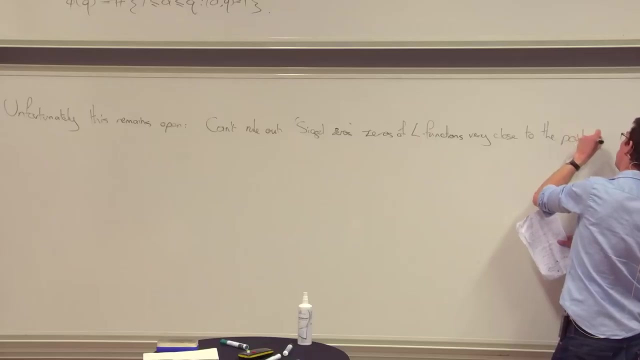 like 3 quarters And maybe the Well, certainly one key issue is we can't rule out so-called Siegel zeros, which are zeros of L functions very close to the point 1.. I don't want to be too specific about what I mean by very close. 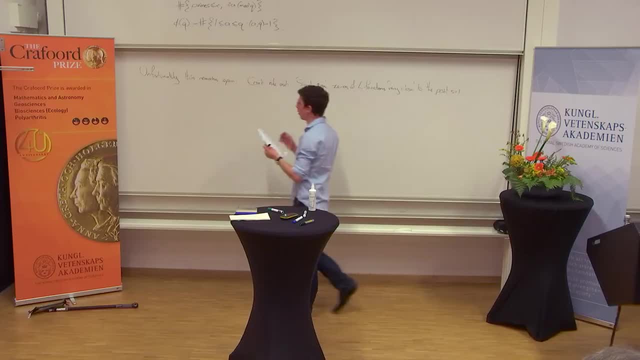 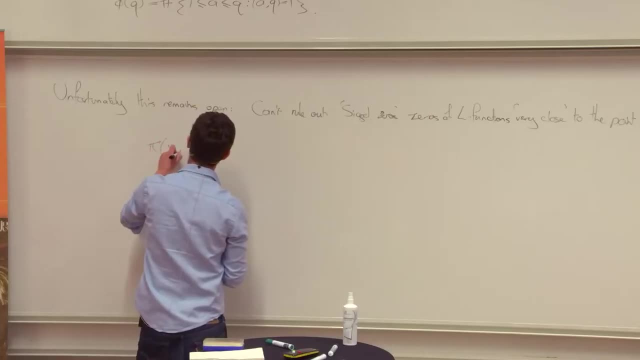 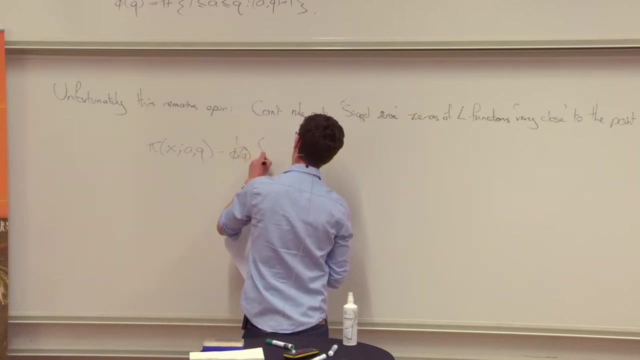 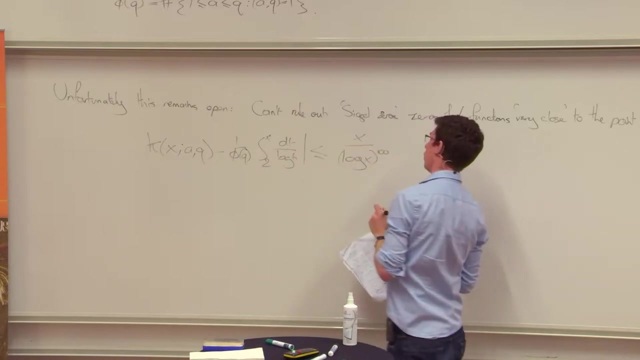 so I'll just put it in inverted commas And without making progress on this. we are stuck at showing that This thing that we're interested in is maybe bounded above by x, divided by some large power of log x, And that's why it's called the Riemann Hypothesis. 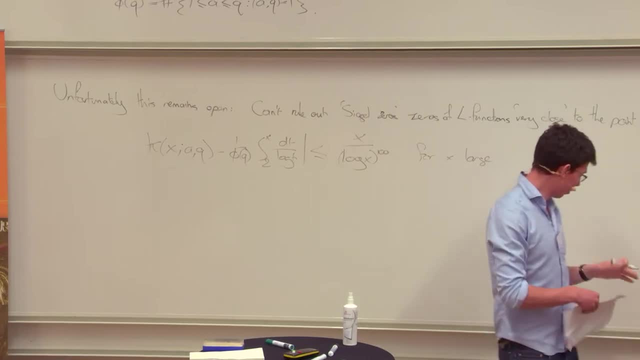 I think it's the most obvious answer to this, but it's good to know we're not going to have many people on the planet and we don't want to have any problems of using this form Or the similar thing we've done. 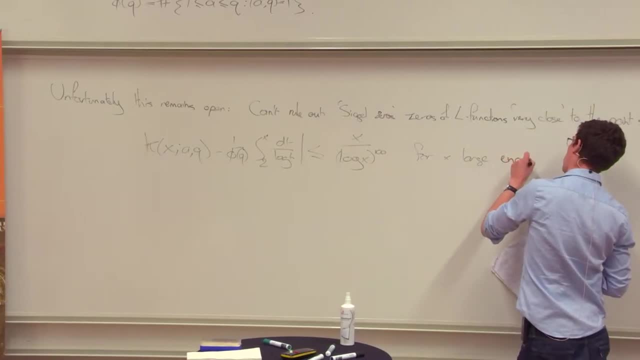 with a product because we don't want to use it as an executive form, Because what we are going to have is very own-use, And that's why we can't use it as an executive form, because that's what the whole problem is. 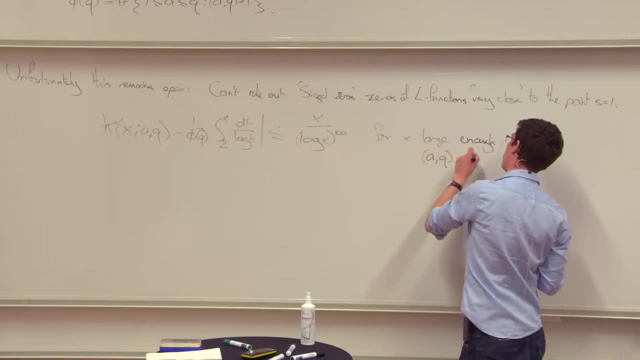 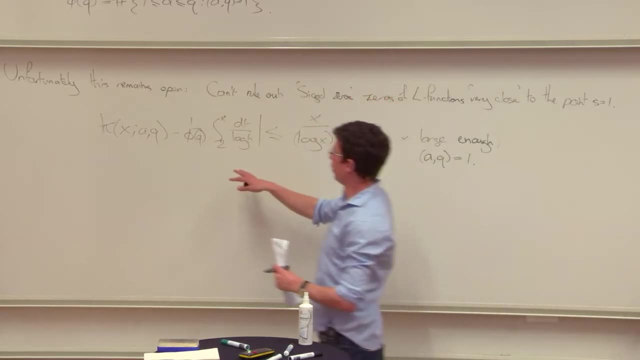 We'll talk a lot about it later, But we'll definitely talk about it in my next last talk. Some of you might be curious about their power. So we have. but this is this whole result is only non-trivial if q is bounded above by some power of log x. 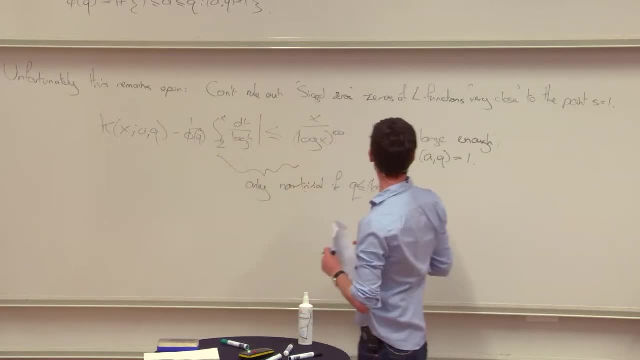 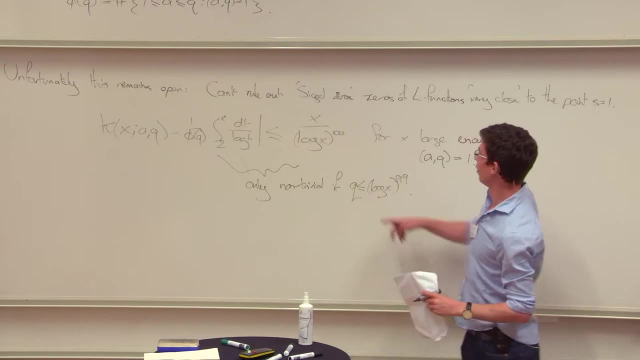 As I have stated it here, this has size, maybe x over log x. so for this choice of constant 100, then this is non-trivial, only for q less than x to the power of log x, to the power of 99. Obviously, 100 is not important here. 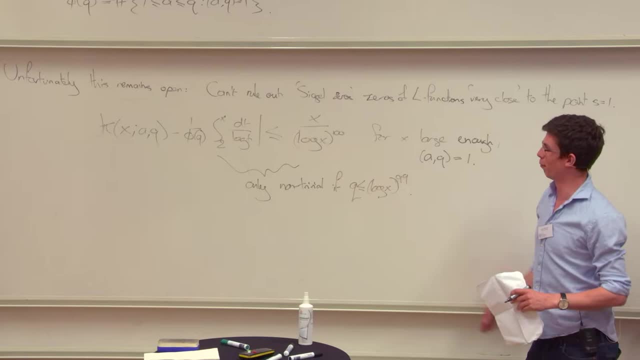 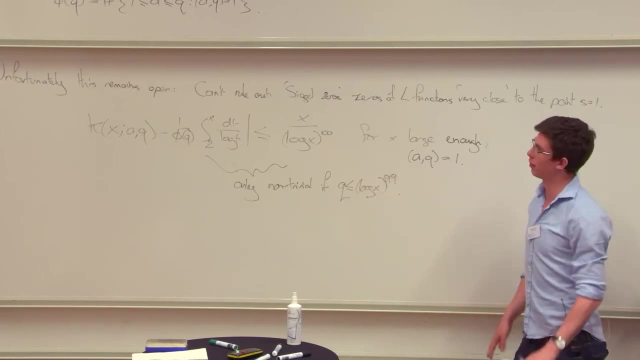 You can replace 100 by 1,000, and then it would be non-trivial for q going up to log x to the power of 999, but q has to be of size logarithmic in x, and this is really a big issue for analytic number theory. 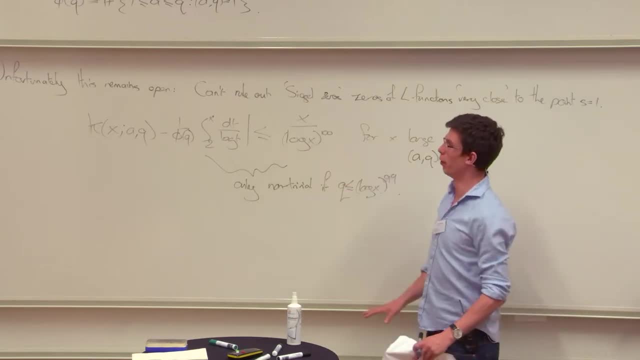 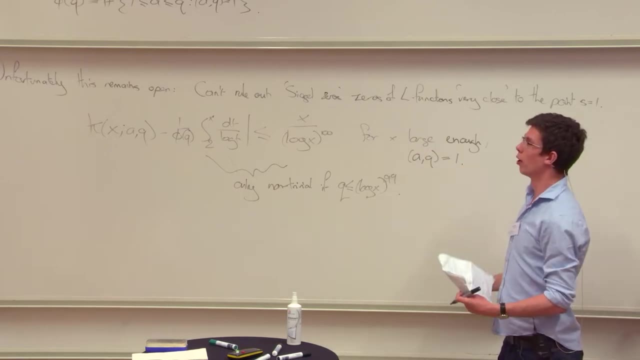 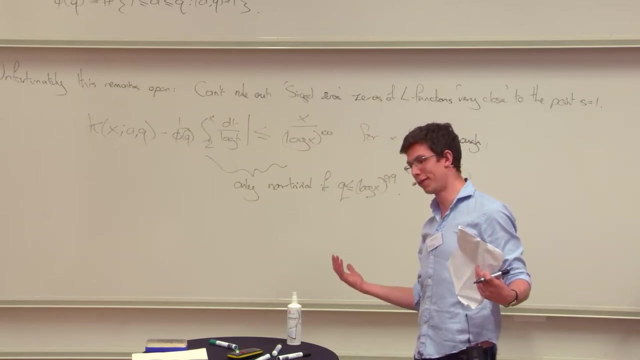 It really limits lots of progress, and if this was all we knew, then there would be lots of different problems and applications which really remain out of reach. So one of the reasons that the Riemann Hypothesis is viewed as the most important open problem in mathematics. 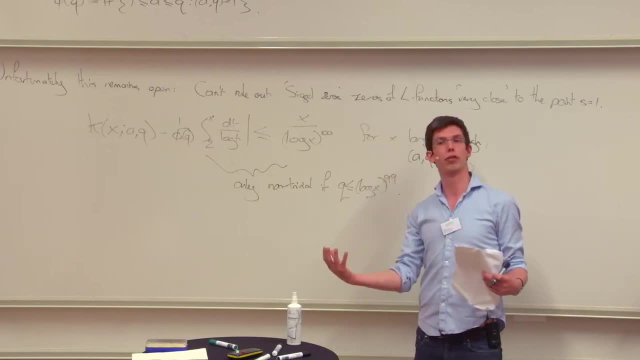 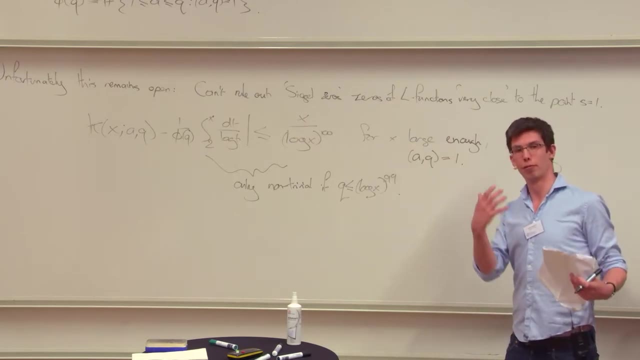 is because it points to some very fundamental deep structure within the prime numbers. but another reason why the Riemann Hypothesis and the generalized Riemann Hypothesis are viewed as some of the most fundamental problems in mathematics is because it would have 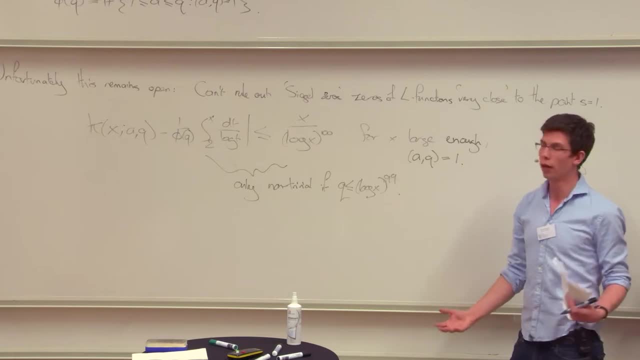 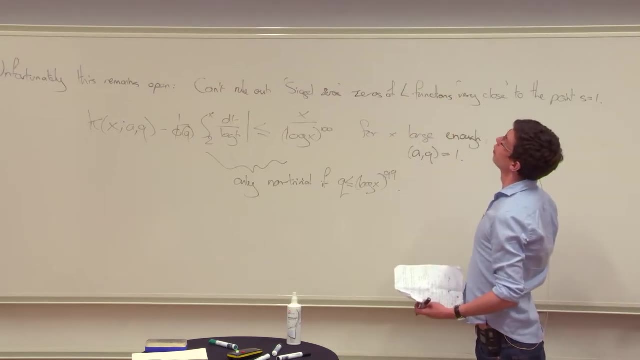 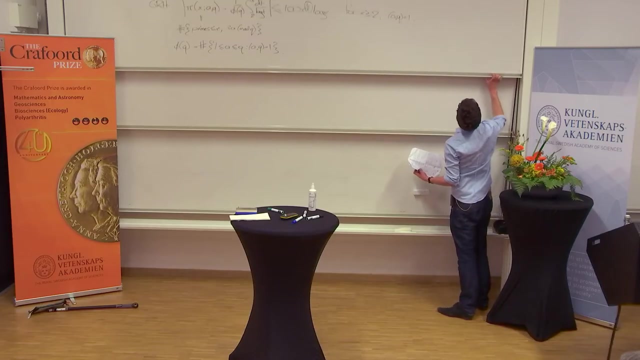 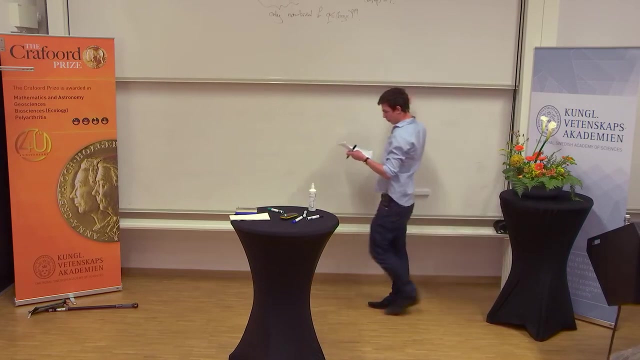 lots of further applications to lots of other different problems, And so they're both fundamental, useful and useful. Let's try again a bit harder. I don't want to break anything, Okay, but that gets us to the Bombieri-Vinogrado theorem. 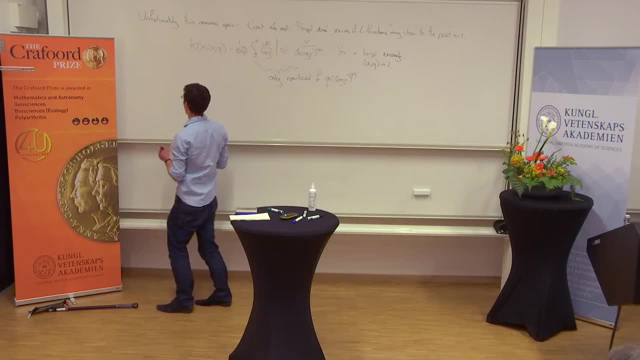 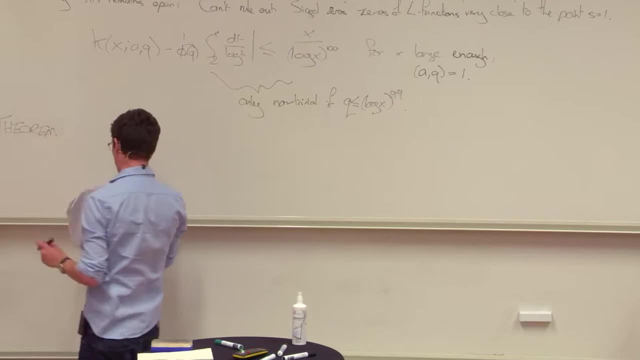 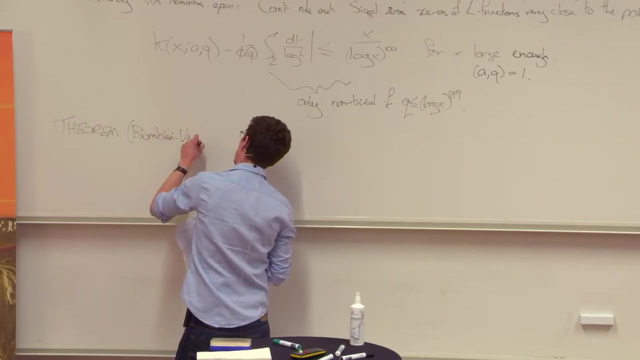 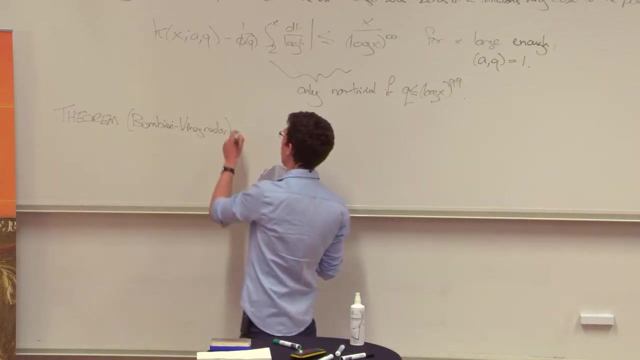 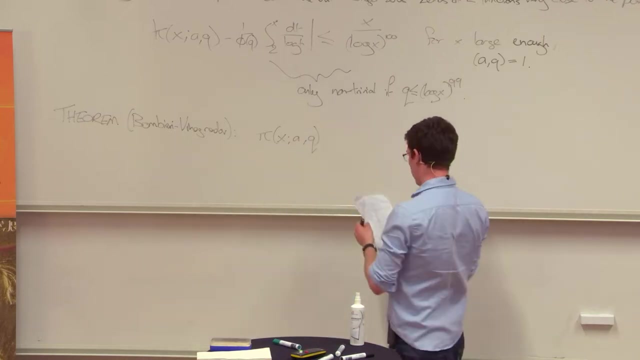 which is maybe my favorite one of Bombieri's results. So it can take a few different forms, but maybe a weak version would be that the generalized Riemann Hypothesis holds for most queues. So this is equal to what you would expect. 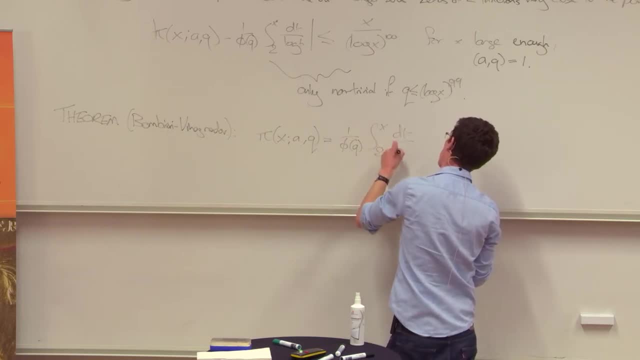 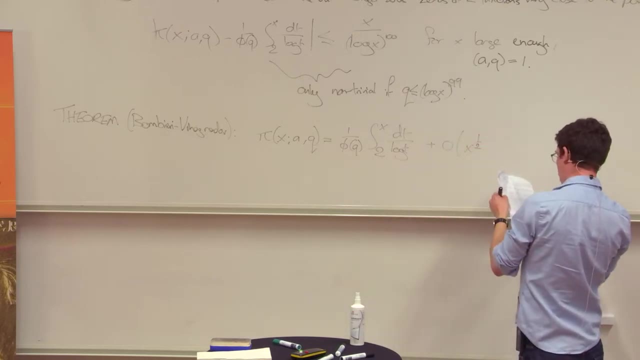 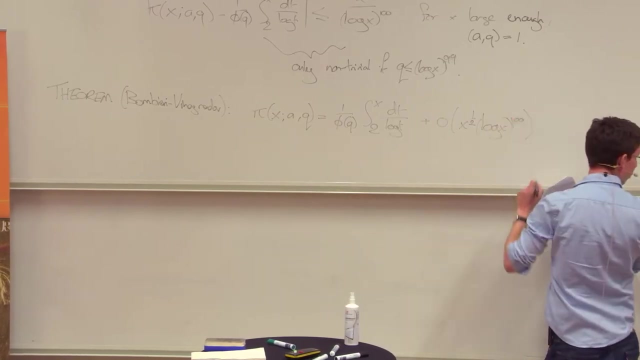 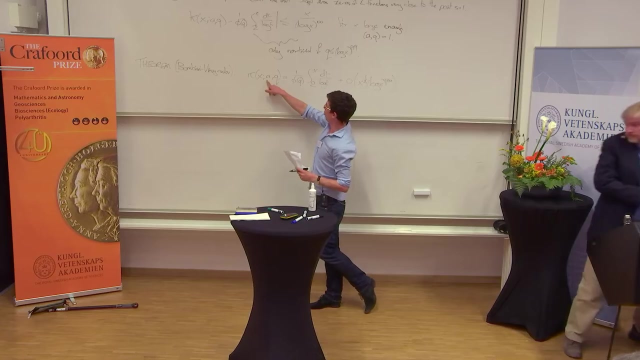 if the generalized Riemann Hypothesis was true, Maybe with an error term that's ever so slightly bigger than what I had up there, but is essentially of the same size. So maybe I'll have log x, the power 100, and if this was true for all values of a and q, which are co-prime, we'd 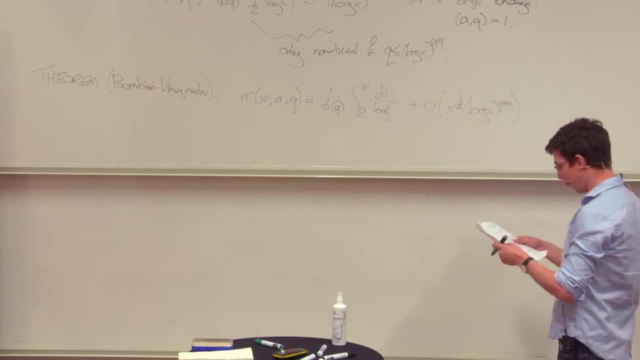 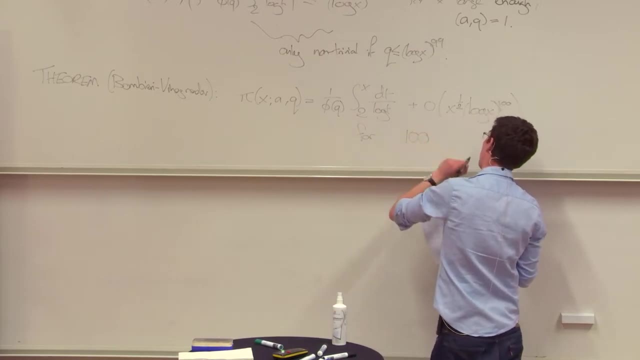 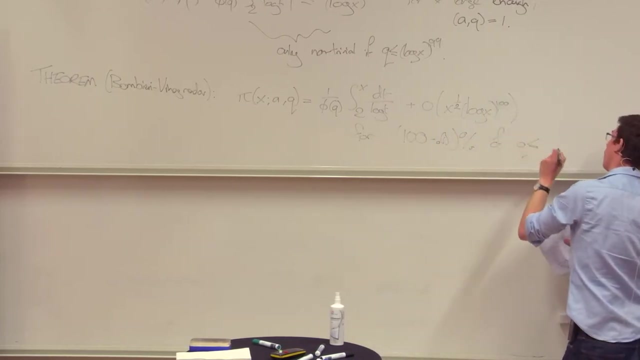 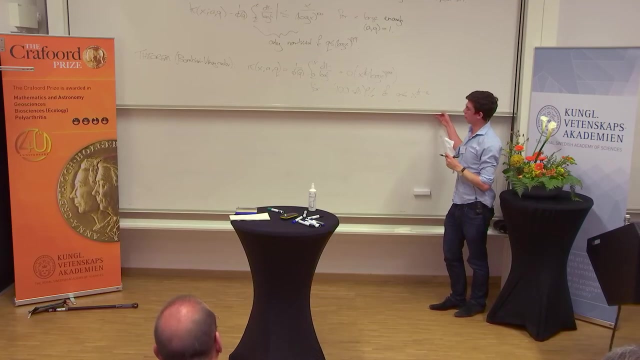 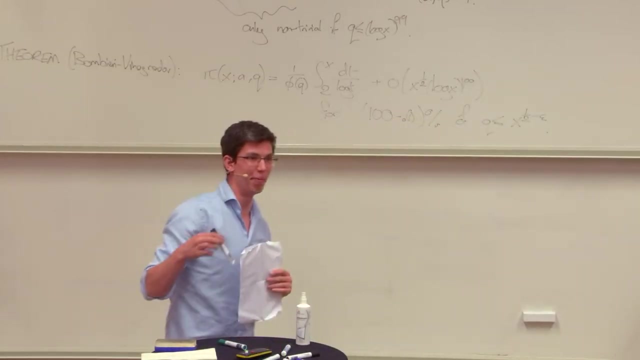 have proven the generalized dream hypothesis, which would be great. but this is true for 100 minus little o 1% of values of q less than or equal to x, to the half, maybe minus some fixed constant. So please continue to bug. 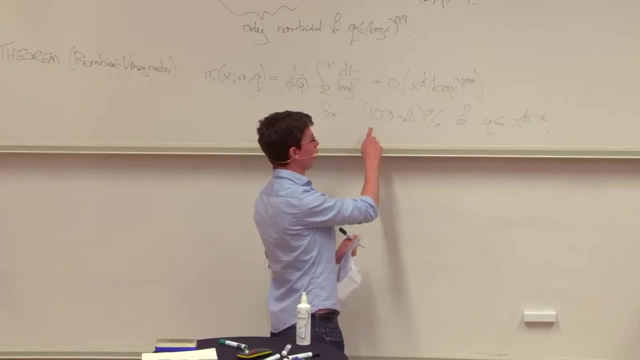 So by this time we're going to be able to do this. So by this time we're going to be able to do this. So by this time we're going to be able to do this. So by this I mean, as x gets larger and larger, we get closer and closer to 100% of different. 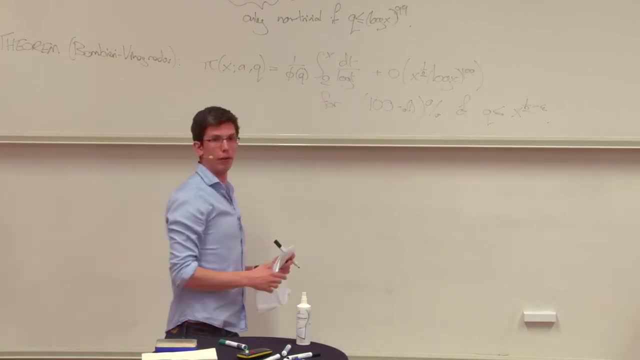 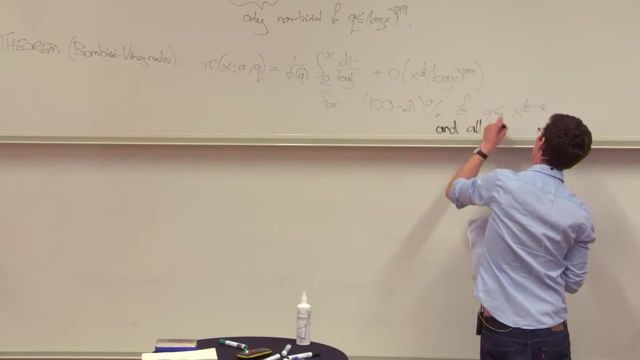 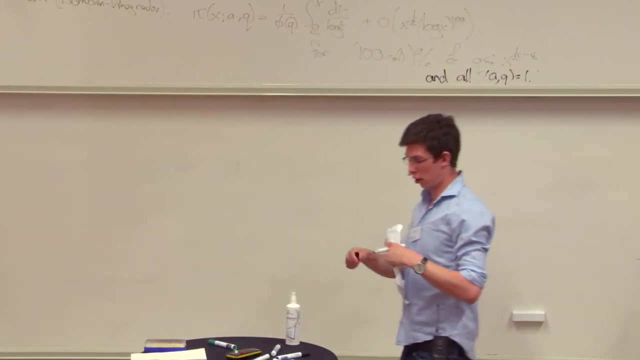 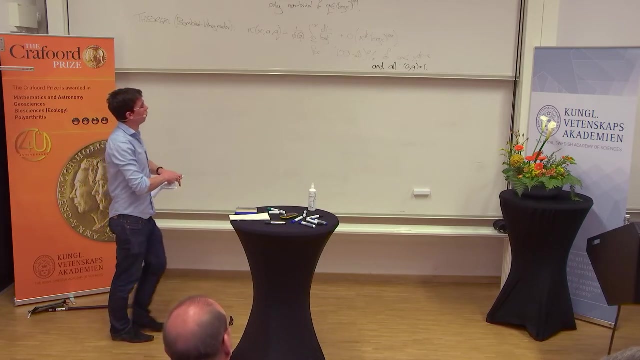 module iq, for which this generalized dream and hypothesis statement holds, And so this has not proven the Riemann hypothesis, but it is proven that Riemann hypothesis is a very good hypothesis for almost all values of q in this sort of statistical sense. 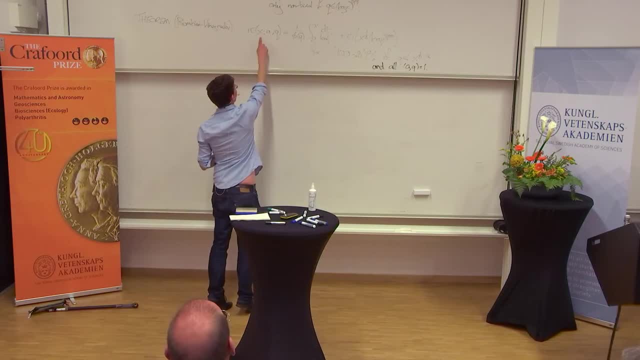 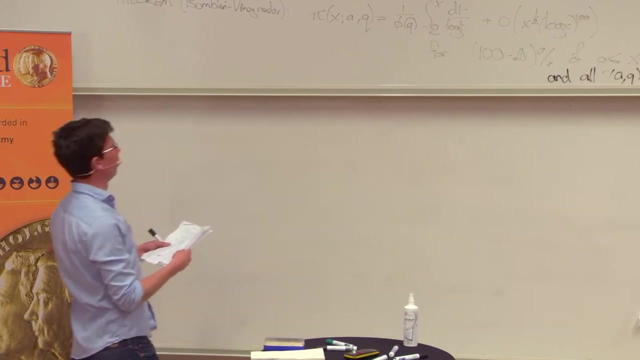 And so at least if you're only looking at primes of a sensible size relative to q, then you can choose the value of q at random and be reasonably confident that the generalized dream hypothesis up to that sort of height will hold for your value of q of interest. 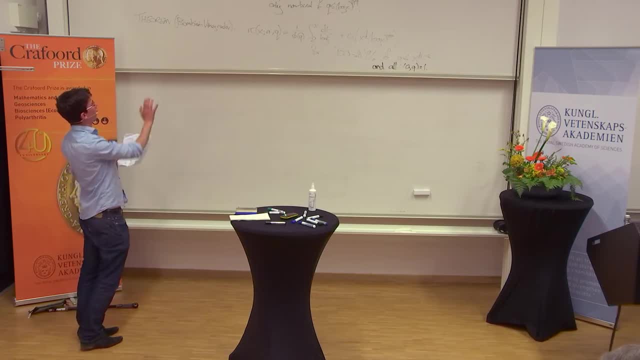 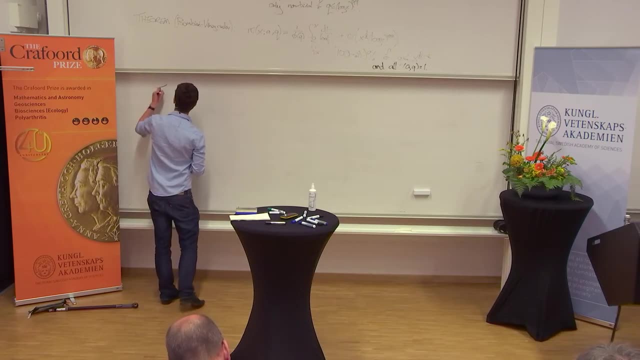 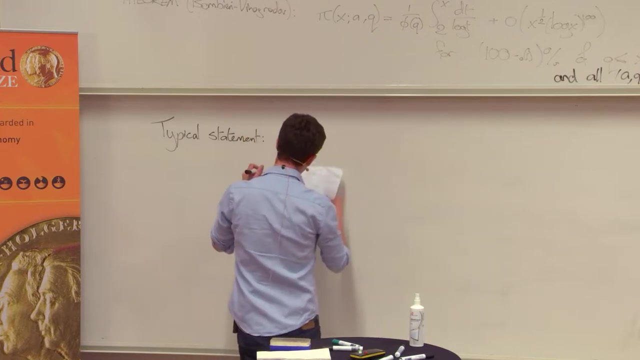 So this is why it's often referred to as proof of the Riemann hypothesis. In fact, it is a generalised dream hypothesis on average, and maybe a more typical statement which is a little bit more technical is that if you sum over all moduli q, which are a little 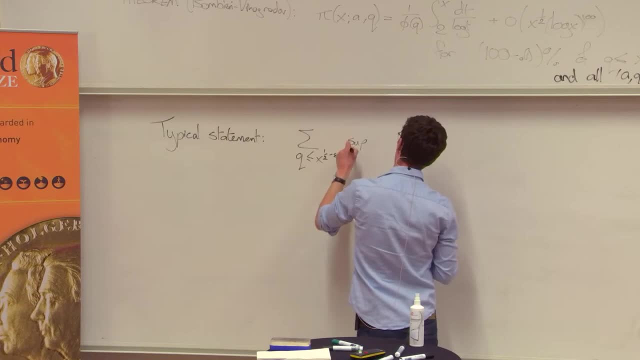 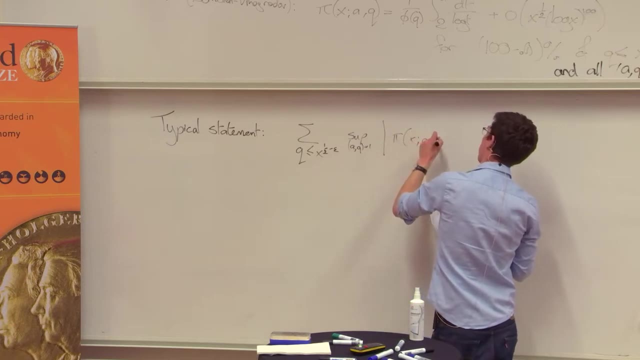 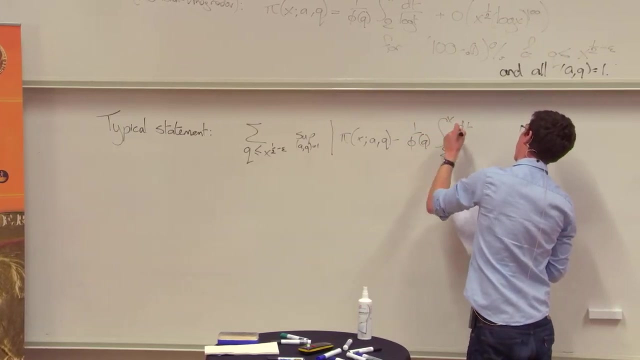 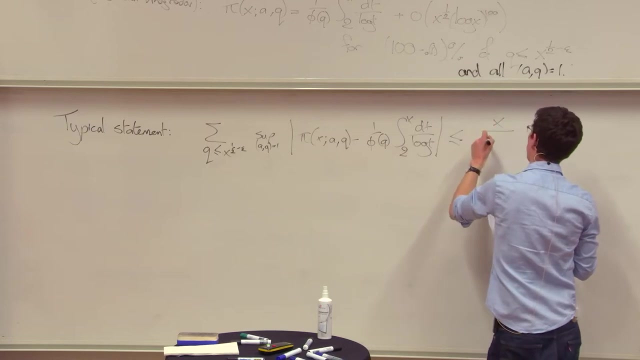 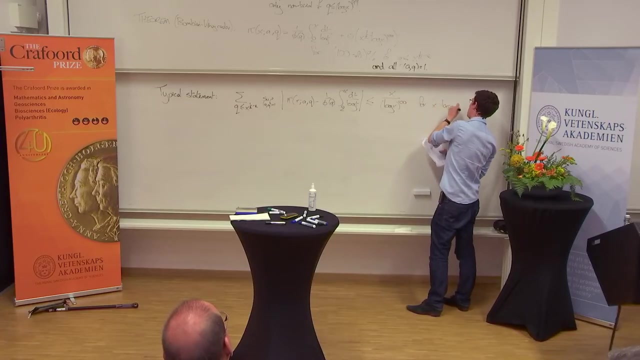 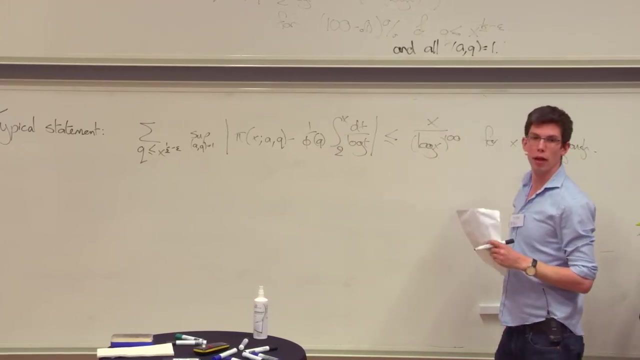 bit less than x, 1 1⁄2, and you take a supremum over a and q. and then you look at this difference that we're interested in. for the generalized Riemann hypothesis you get an answer which is essentially the same sort of thing as what you would get if the generalized Riemann hypothesis 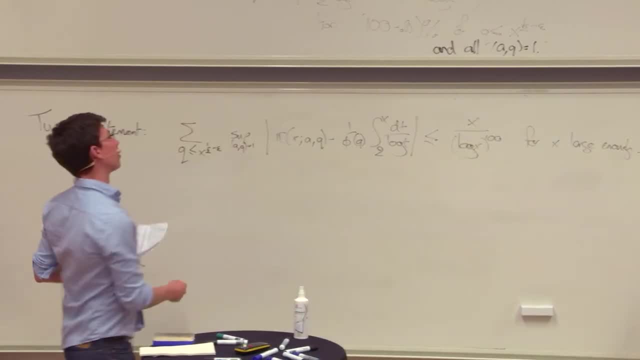 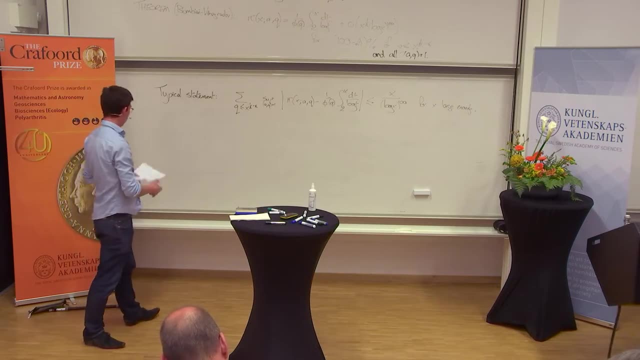 was true. So this is very interesting in and of itself as a result, about the distribution of prime numbers in arithmetic progressions, but the key reason that I, at least personally, really like the Bombier–Winogradov theorem is that, as was mentioned by Per, this is: 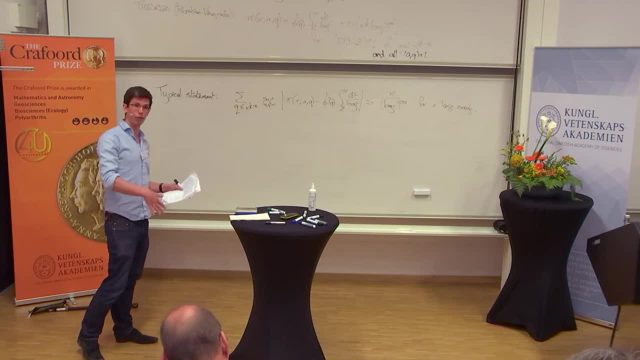 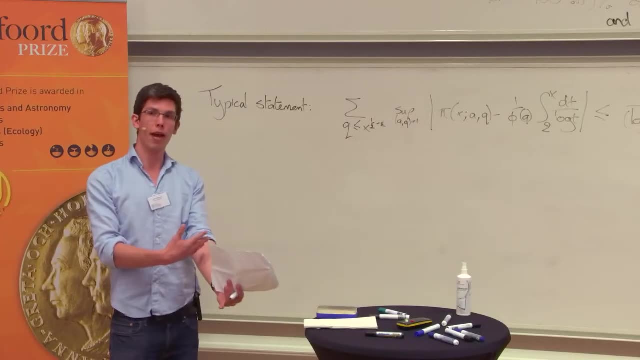 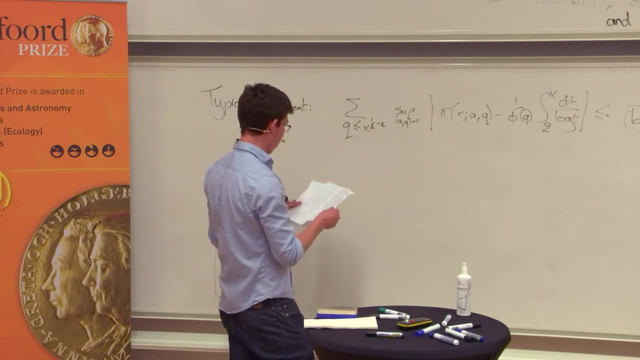 for many applications a perfectly adequate technical substitute for the generalized Riemann hypothesis itself. So one of the key reasons that we're interested in the generalized Riemann hypothesis is its profound other implications for the distribution of prime numbers. but the Bombier–Winogradov 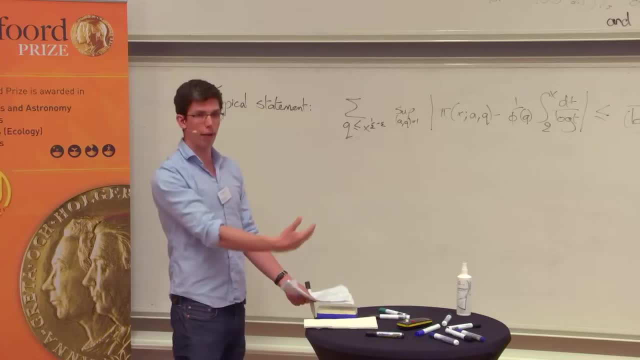 The Saldana Theorem often allows you to deduce essentially the same consequences as you would do if you assumed the generalized dream hypothesis now unconditionally. so you maybe have to work a tiny bit harder to incorporate this slightly more technical formulation, but otherwise it's basically as good. 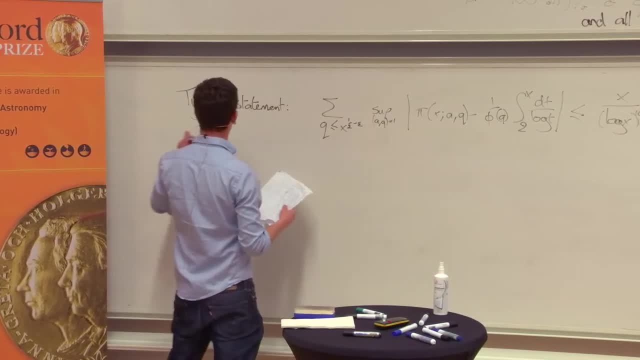 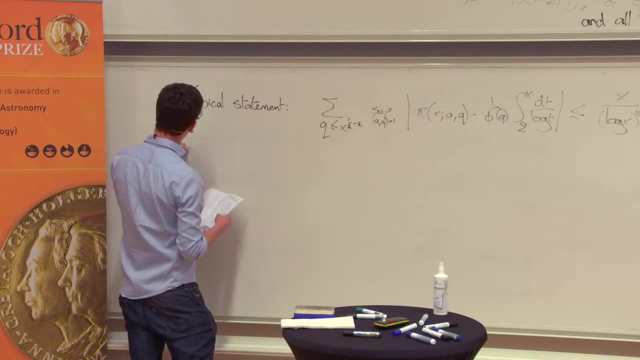 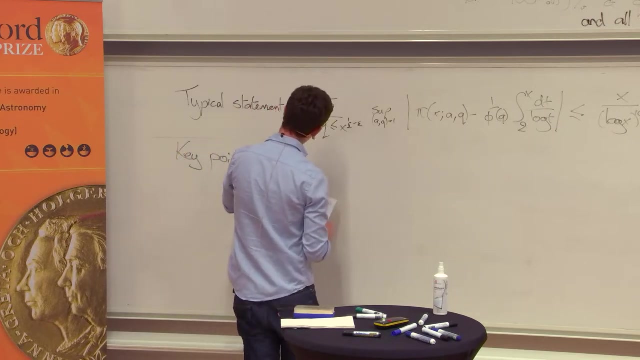 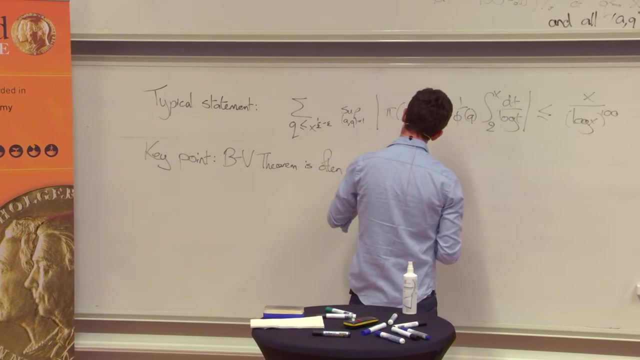 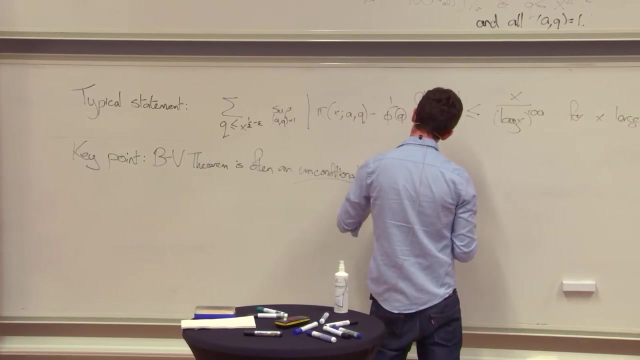 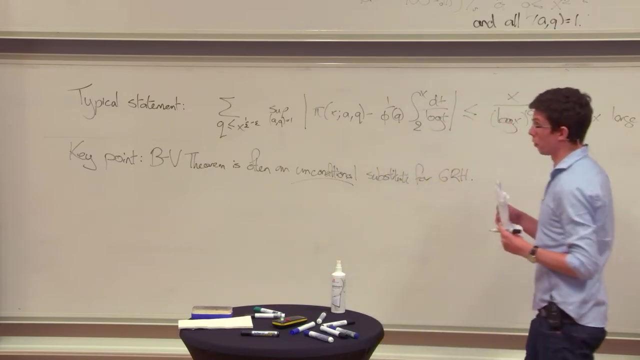 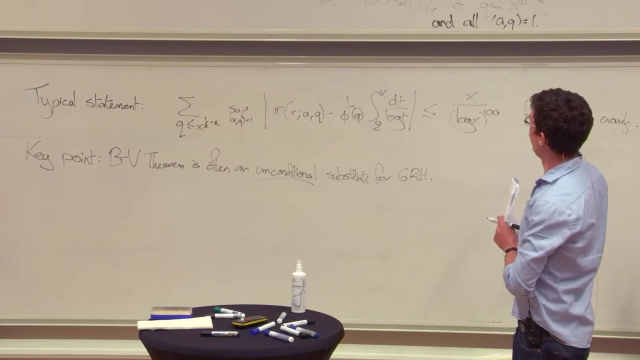 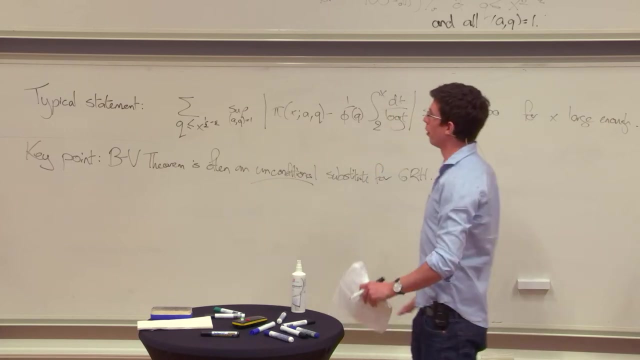 as if the generalized dream hypothesis was true. So certainly when I have students who think about problems to do with the distribution of prime numbers, I'm always very happy to tell them. to first of all make your life easy, assume the generalized dream hypothesis is true. 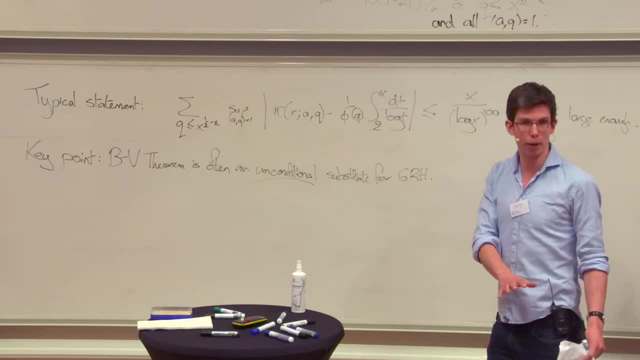 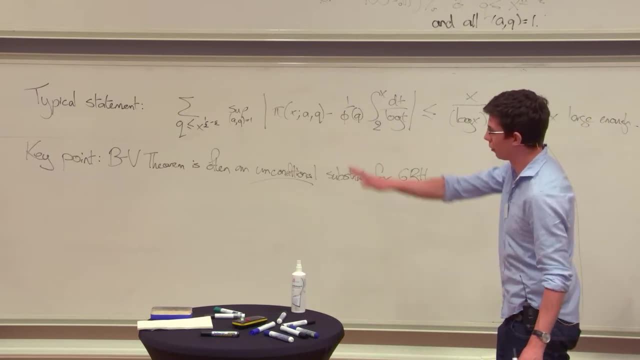 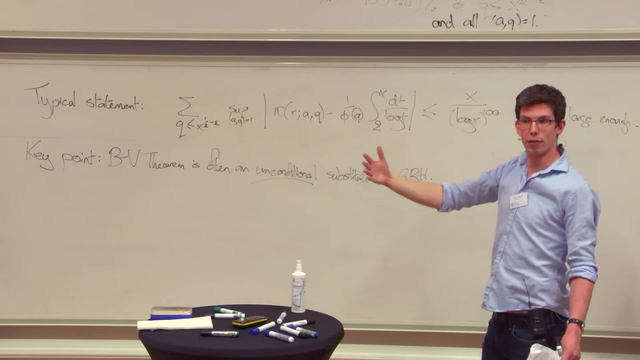 and then, once you have a result assuming the generalized dream hypothesis, you can think about whether the generalized dream hypothesis is really necessary, and in almost all circumstances either. there's some big obstruction to do with z equals zeros, in which case you've hit a famous roadblock. 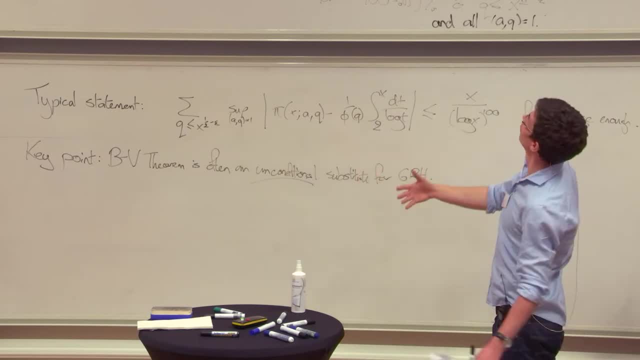 and it's likely that you're. the theory is that you've hit a famous roadblock. and it's likely that you've hit a famous roadblock, and the theory is that you've hit a famous roadblock, that the problem that you're trying to prove is kind of false. 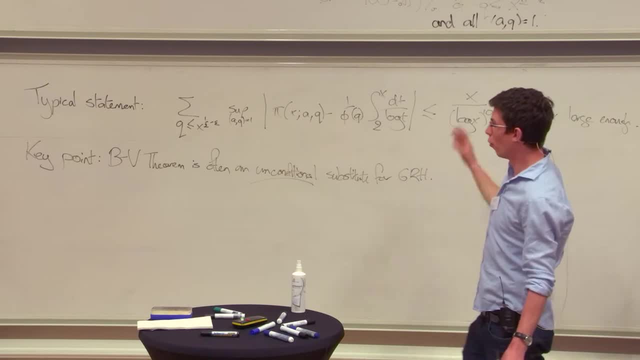 that the problem that you're trying to prove is kind of false. if these putative z equals zeros really existed. if these putative z equals zeros really existed, or you can use the Bombier-Vinogrado Theorem or you can use the Bombier-Vinogrado Theorem. 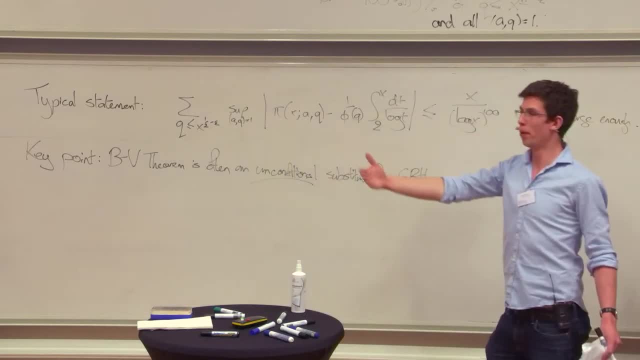 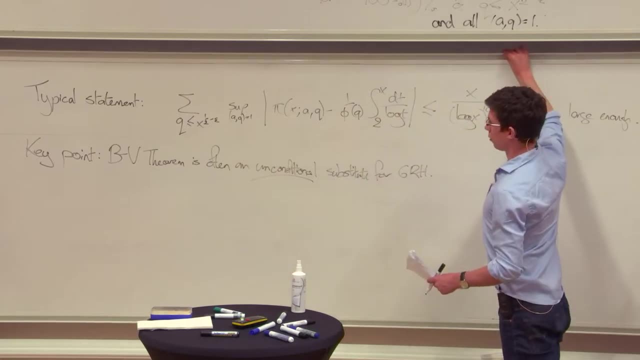 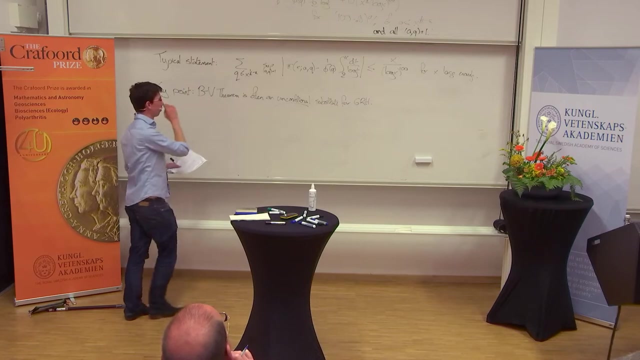 and you can make your result unconditional. And so either there's this big famous obstruction or you can make it unconditional using the Bombier-Vinogrado Theorem. So this has happened for a number of different things. so I guess the Bombier-Vinogrado Theorem. 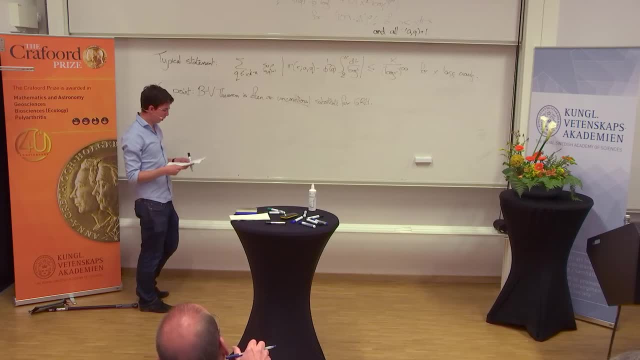 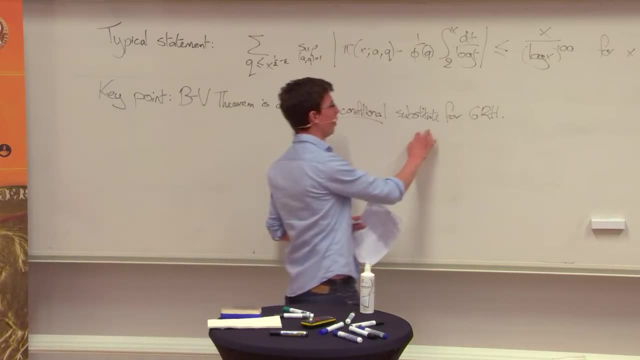 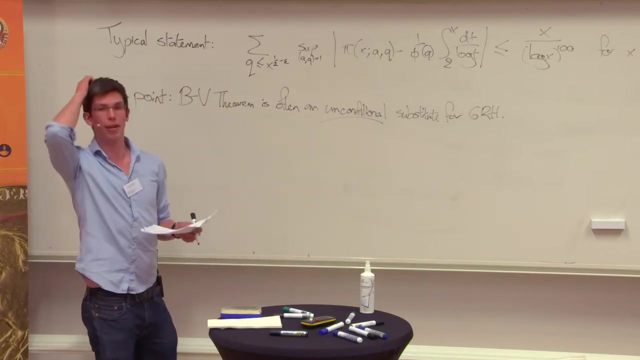 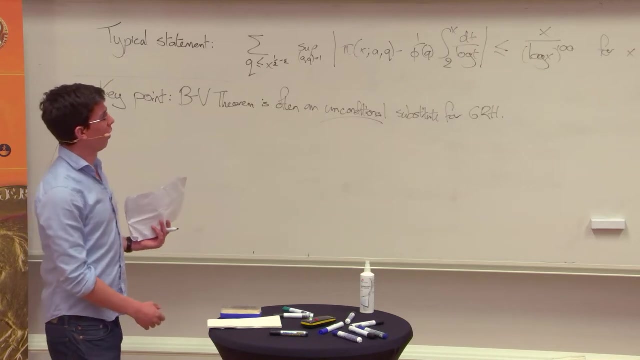 came out around 1960, and I think lots of people were then going through different arguments to see in which ways this could make different results unconditional. So I certainly remember Peter Sarnak talking to me about when his student Zaharescu was working about diaphragm-to-hand approximation with squares, and it went through exactly. 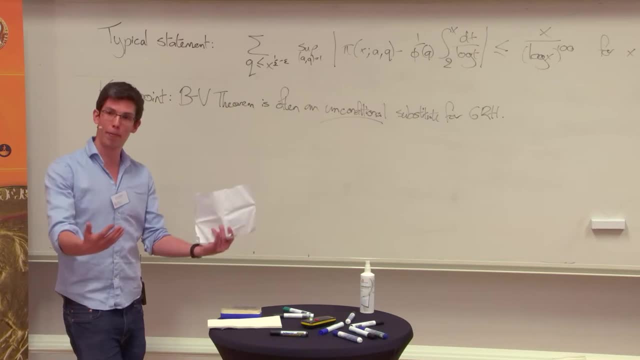 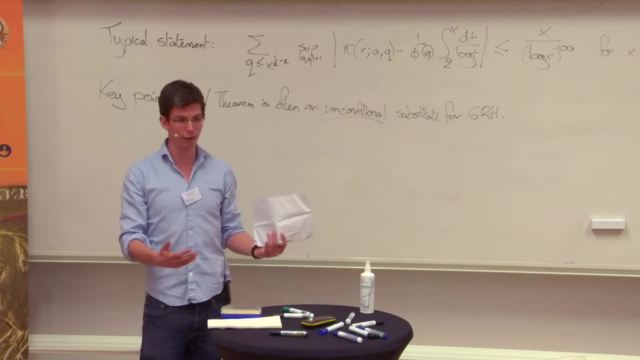 this process that Zaharescu came up to Peter Sarnak and said very excitedly: oh, I think I proved this really nice result about diaphragm-to-hand approximation with squares. I'm very pleased with it. the only downside is that I have to assume the generalised dream hypothesis. 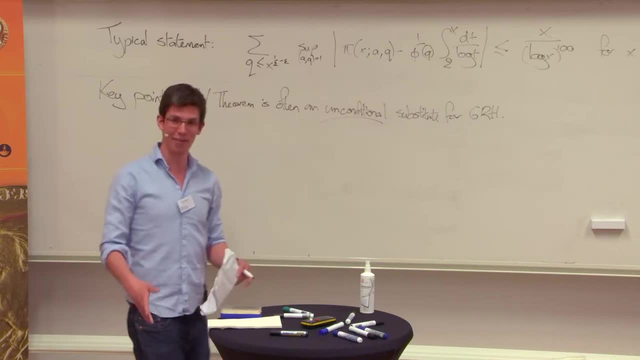 and Peter Sarnak said: I wouldn't worry too much about that, you explain the result to me and then I'll tell you how you can make it unconditional. And it was the ideas, at least, behind the Bombier-Vinogrado theorem that applied then. 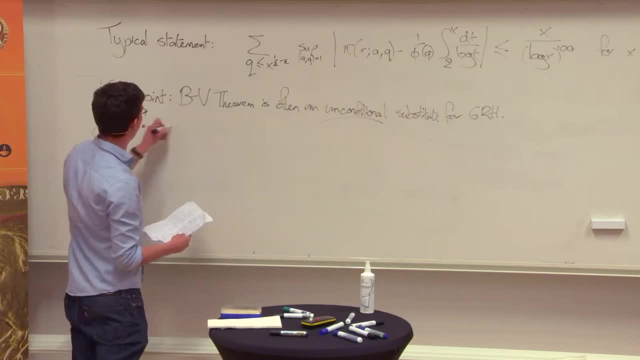 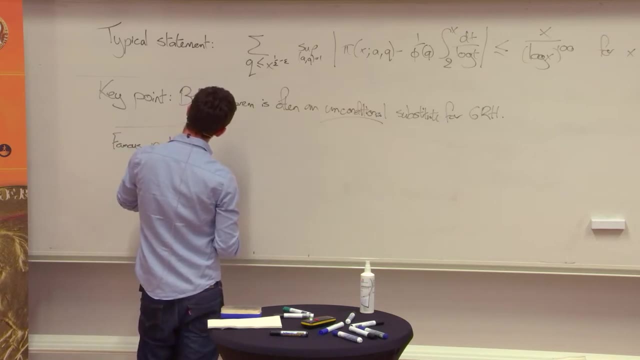 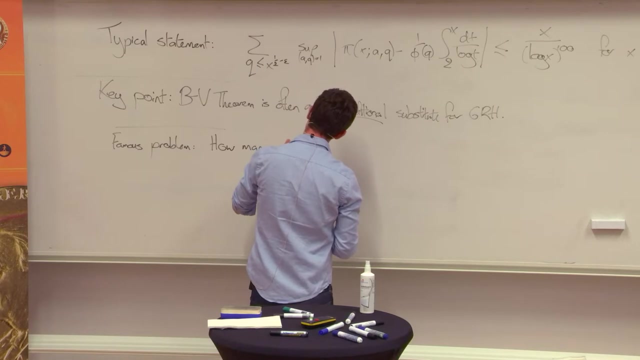 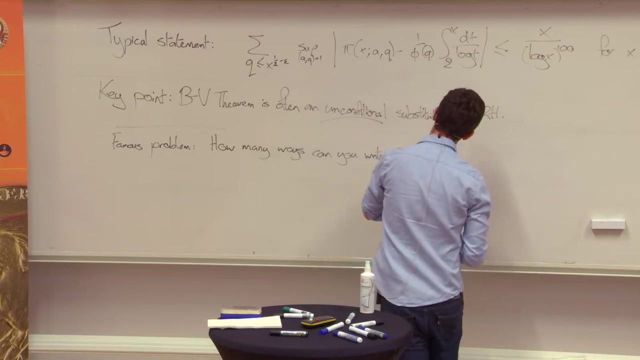 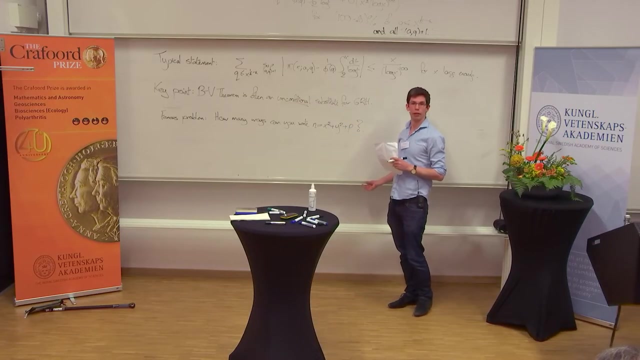 and maybe another famous example, or or famous problem at least, was: how many ways can you express an integer as the sum of a prime and two squares? In particular, can you write every large integer as the sum of a prime and two squares? 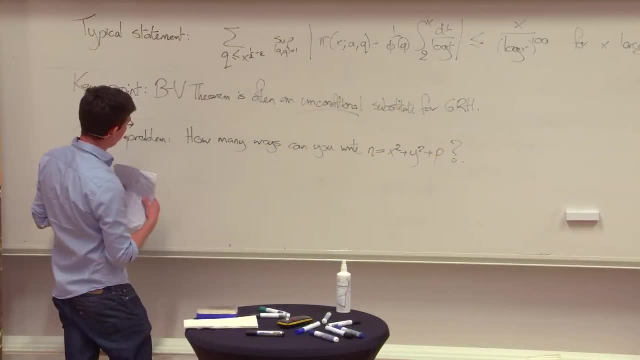 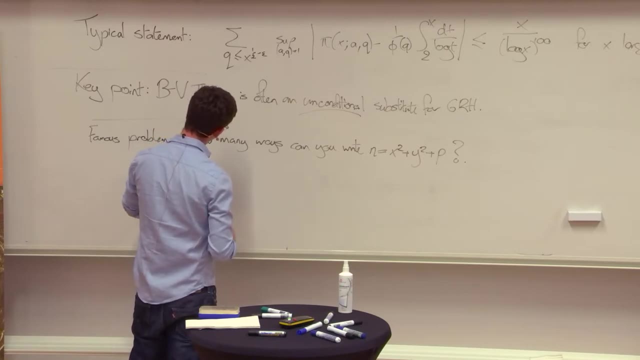 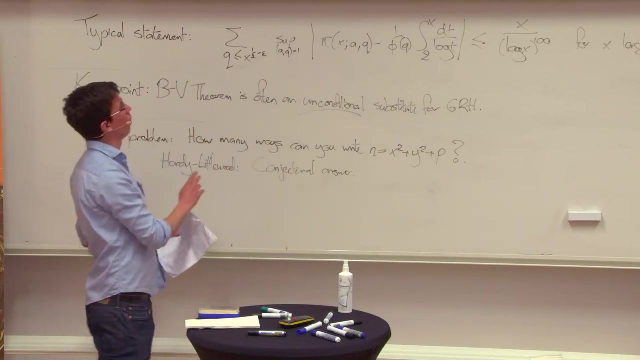 This was maybe a slightly strange problem from today's perspective, but this goes back to Hardy and Littlewood, and they gave a conjectural answer. They suggested that it should be possible to write every large integer as the sum of two squares and a prime, and they guessed a formula for how many ways you should be. 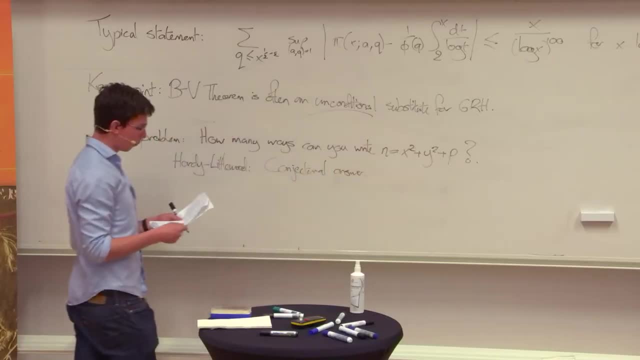 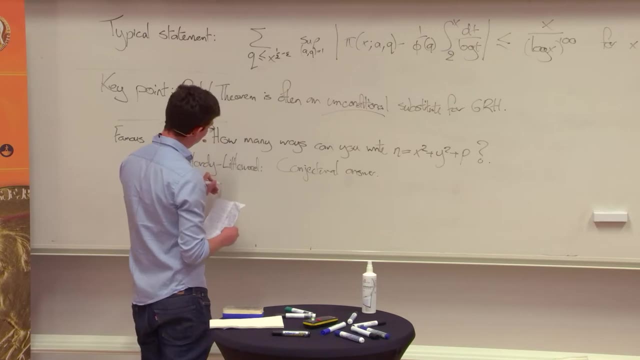 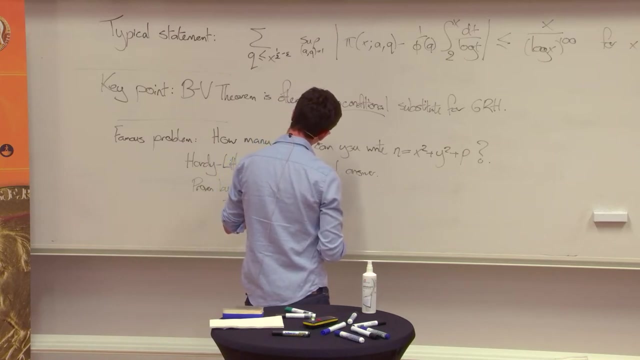 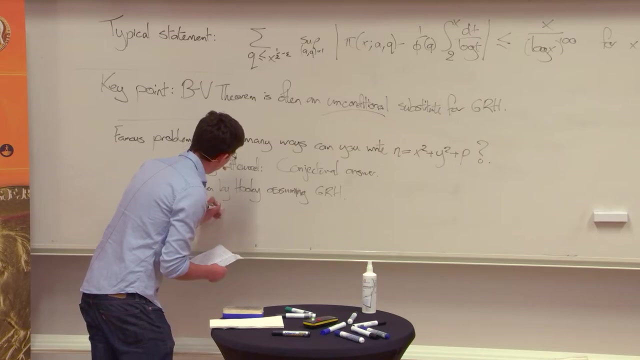 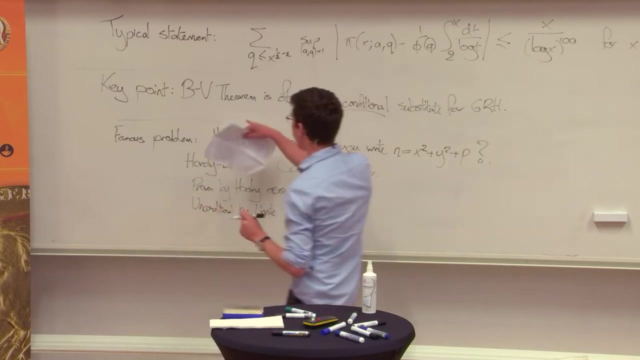 able to do this An approximate formula for when n is large. This was then proven by Hooley, assuming grh. if I can spell, This- was made unconditional Okay By Linick, slightly before the Bombier-Wintergaard theorem, but using a very technical argument. 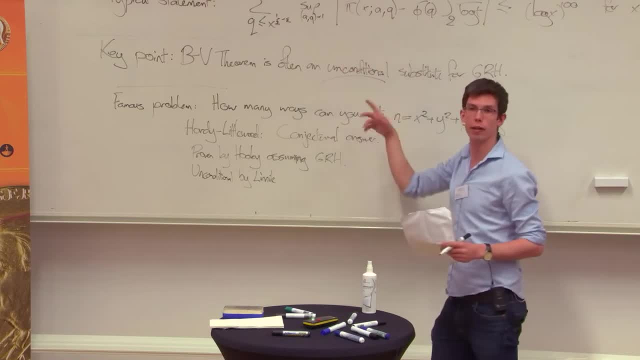 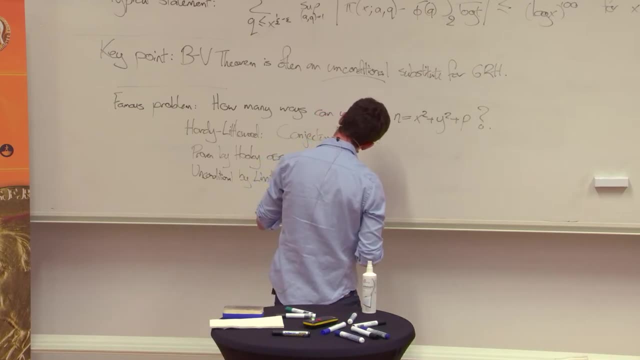 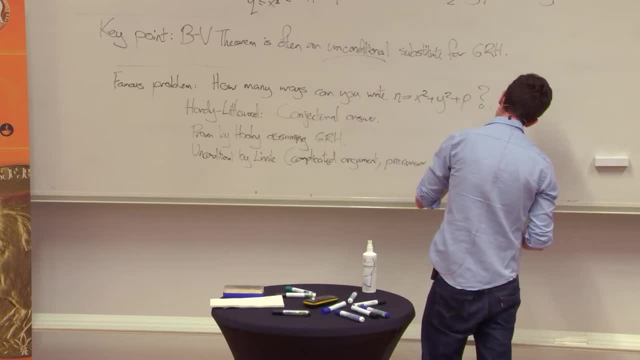 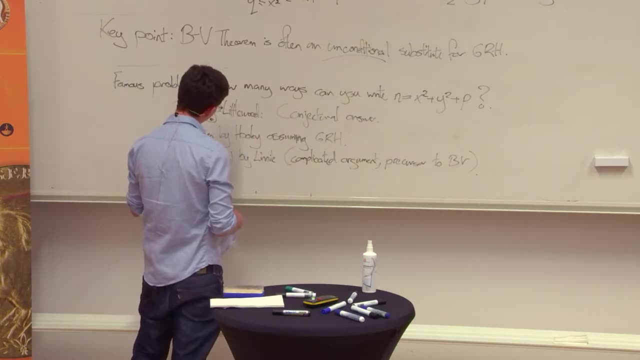 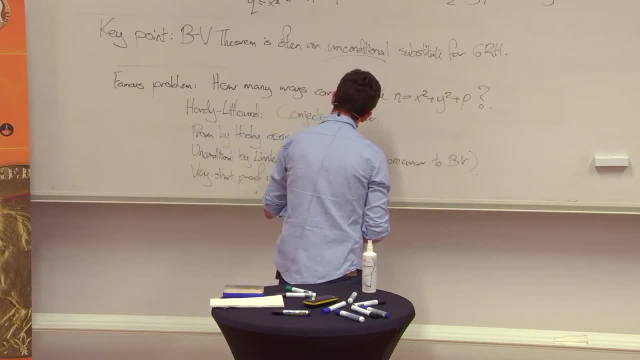 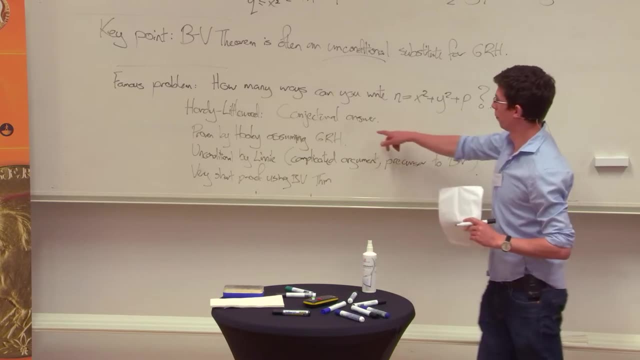 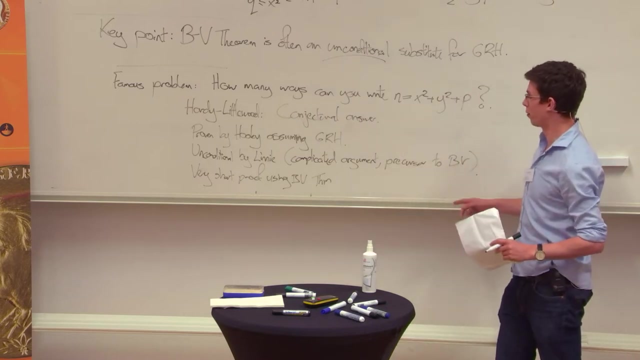 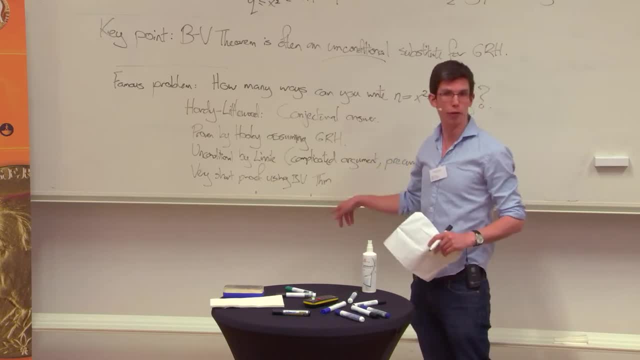 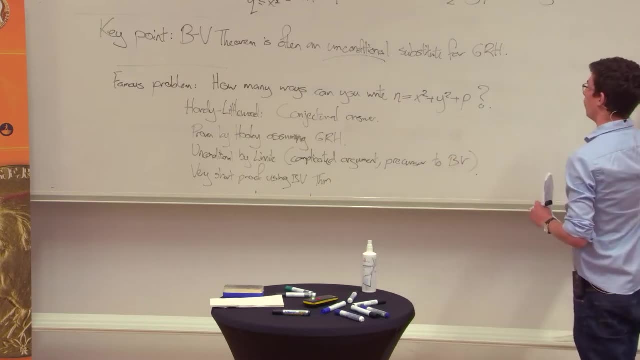 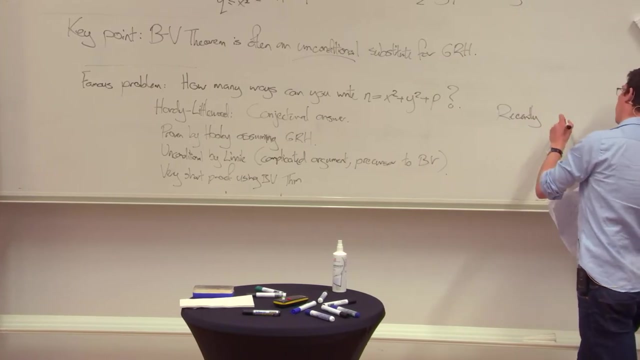 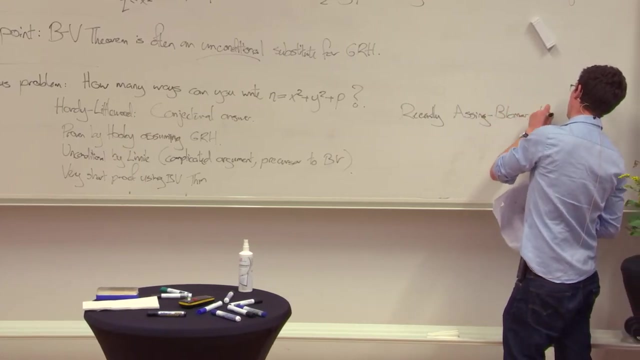 and now has a very simple, clean proof just using the Bombier-Wingard of them as an application. But the story doesn't quite end there, because I guess recently there's a very nice paper of asking Blomer and Lee, who have some technical extension. 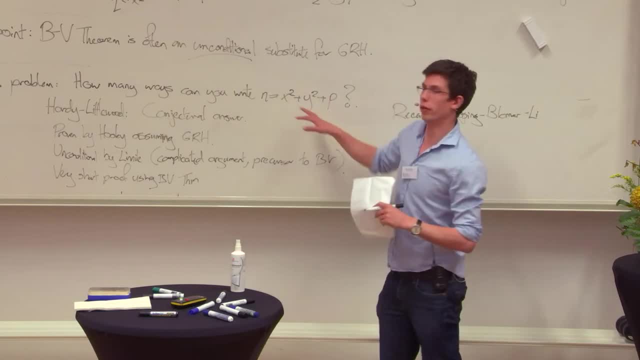 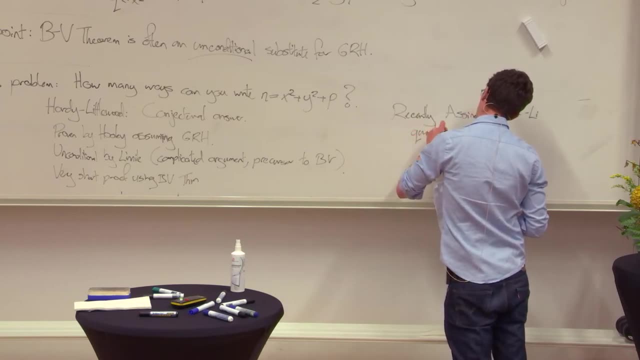 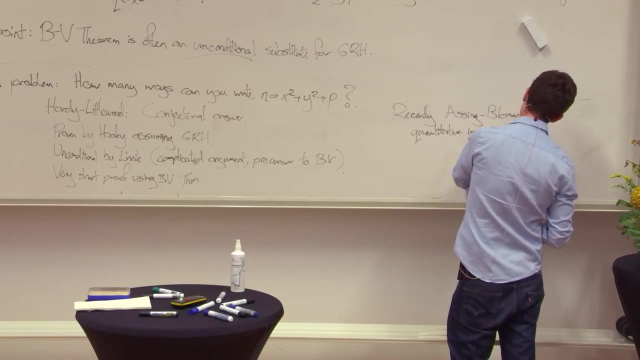 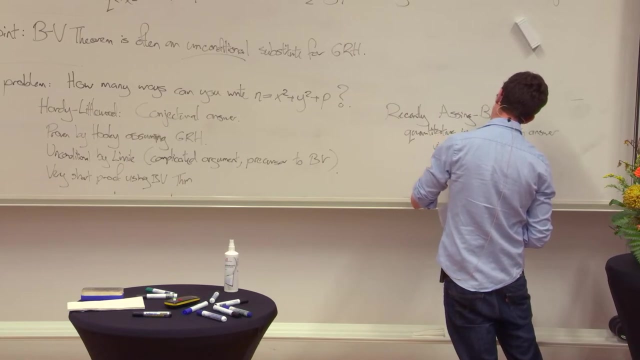 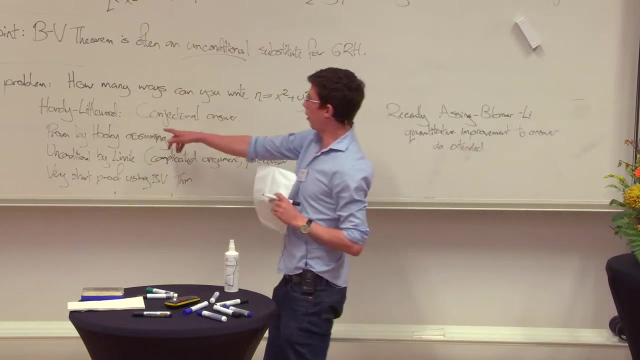 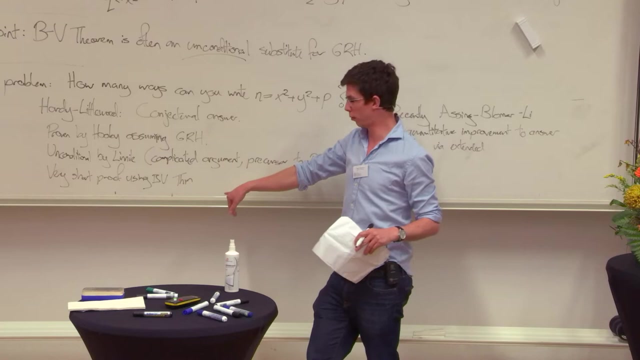 of the Bombier-Wingard of them. that allows them to answer this question in a slightly more quantitative way. So Hardy and Littlewood said it should be approximately this number when n is large, and that's what all of these results were proving. 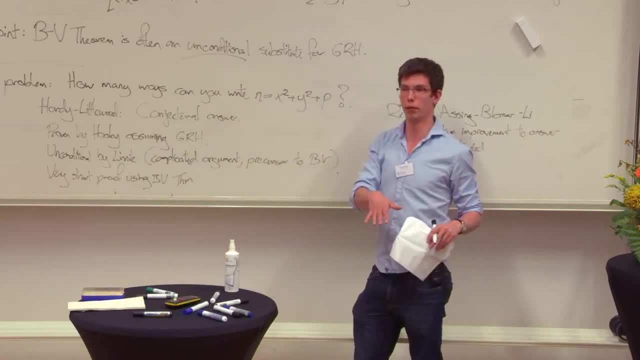 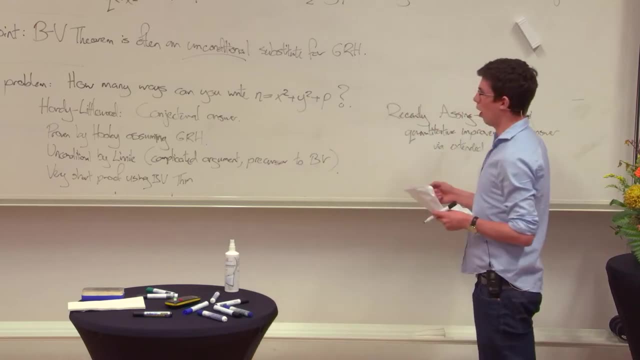 that as n got very large, it was approximately Hardy and Littlewood's guess. But then there's a question as to how close to that guess really are you, and there was a natural sort of limitation in these sorts of arguments that meant that you could only get. 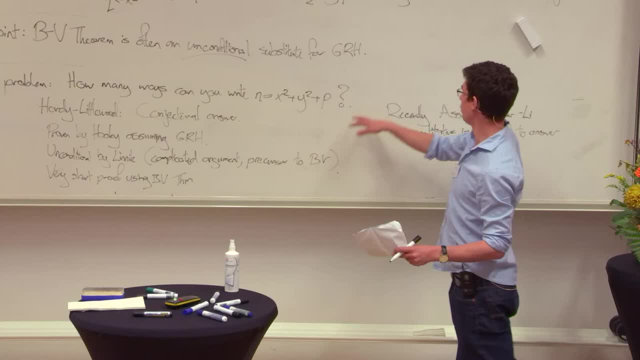 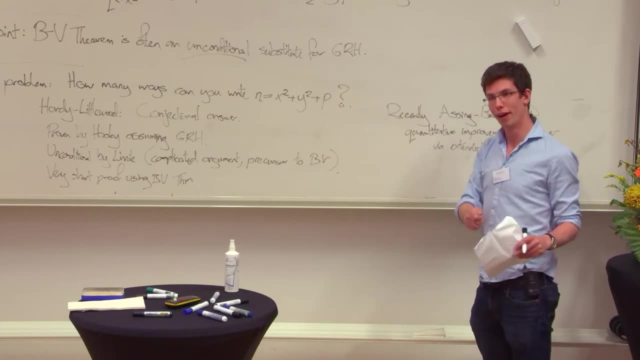 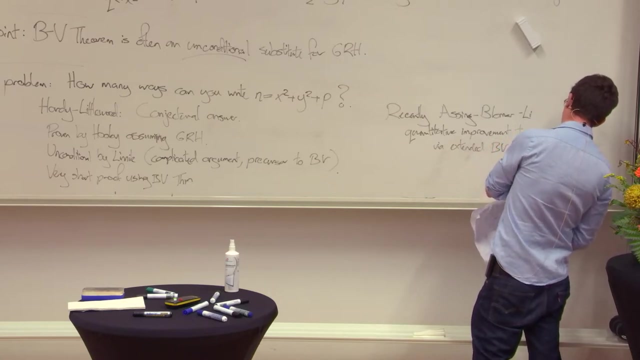 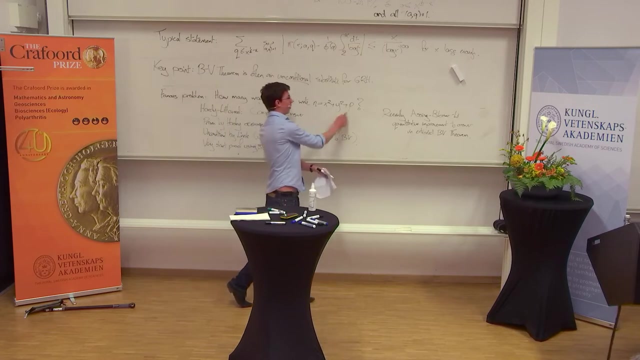 a fairly approximate answer using these sorts of techniques. But this work of asking Blomer and Lee shows that actually this conjectural guess is rather more accurate than the previous works. So the point of this is that there's a lot of- there are some- of these sort of. 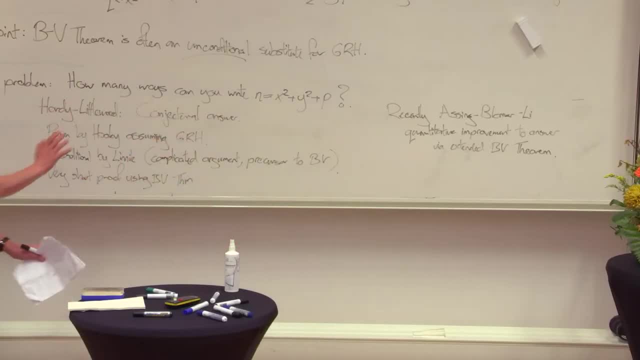 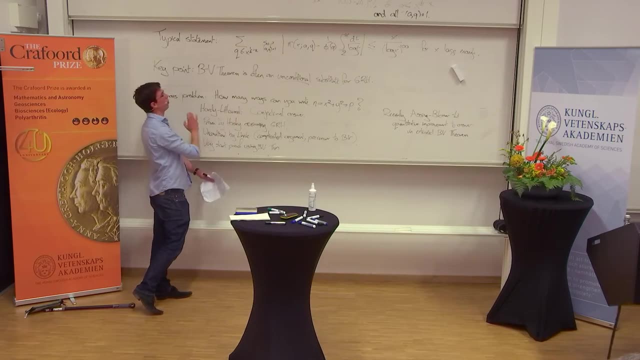 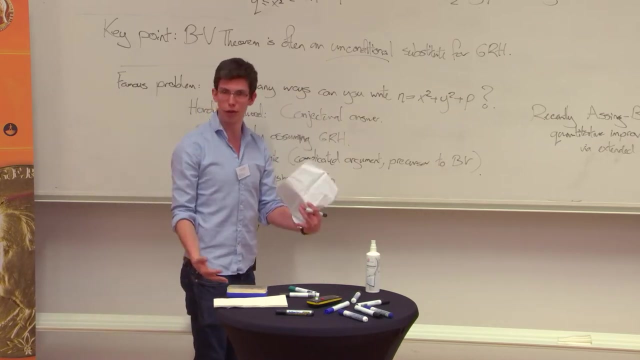 strange old historical questions going back to Hardy and Littlewood, and the whole question was initially solved, assuming these big conjectures was made unconditional. the Bombier-Wingard of them was a kind of perfect drop-in substitute. but even nowadays, 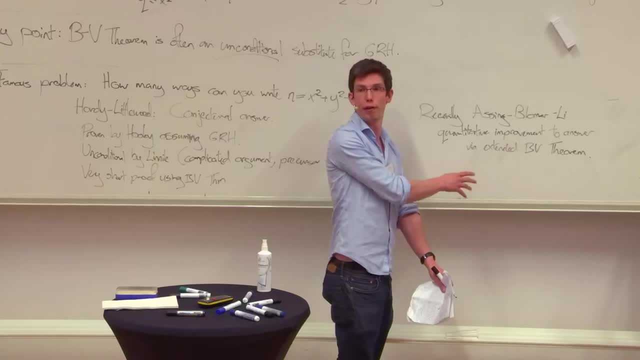 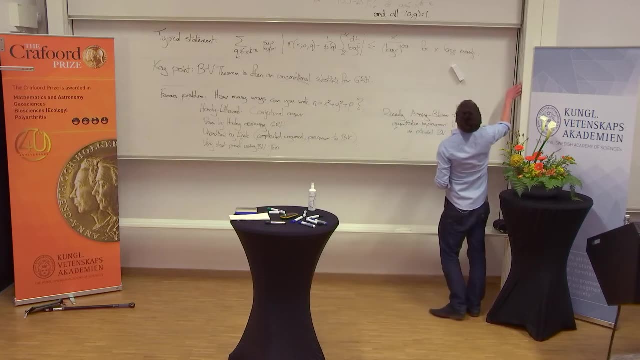 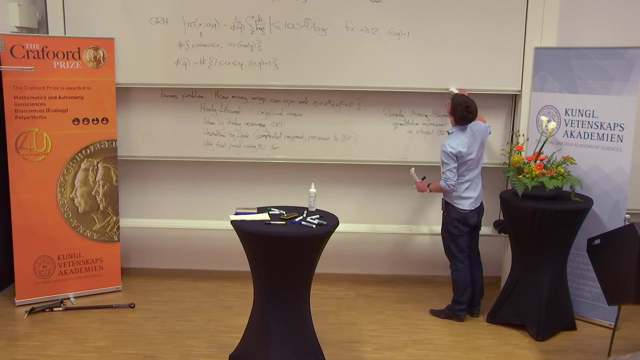 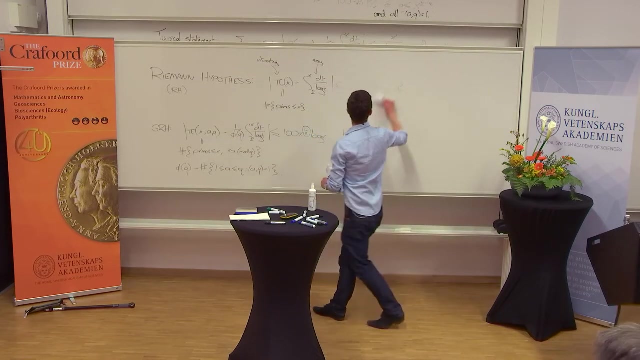 or just a few years ago. the Bombier-Wingard of them is still very relevant and is still leading current developments. So that's supposed to just be a proof of concept that in various ways, the Bombier-Wingard of theorem acts as an unconditional substitute. 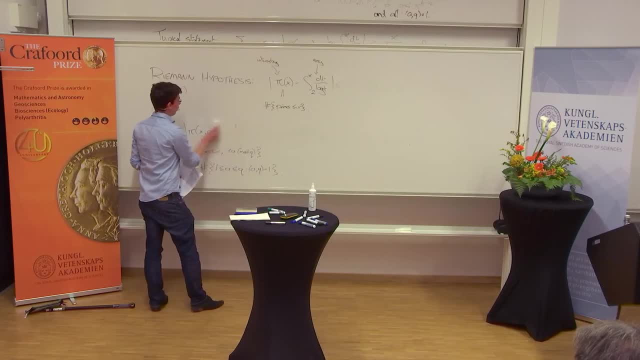 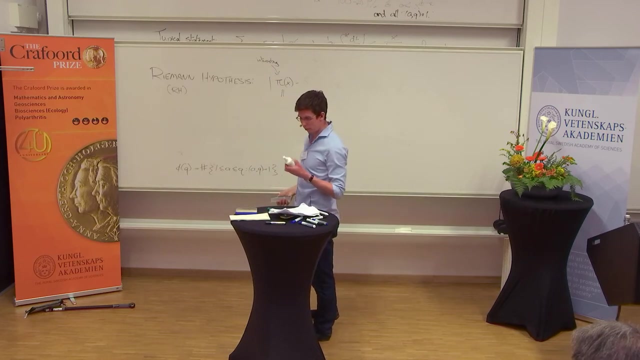 for these very powerful but out-of-reach results on primes and arithmetic progressions. Maybe I should use the spray. Okay, great. 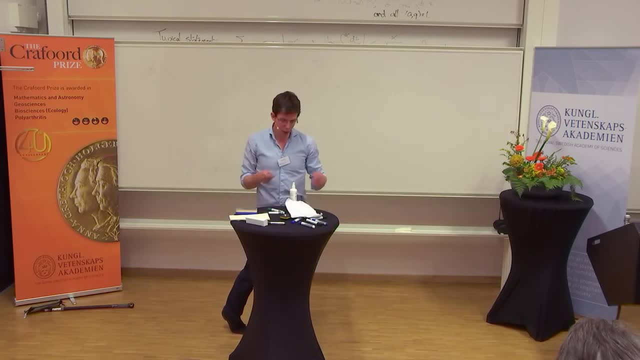 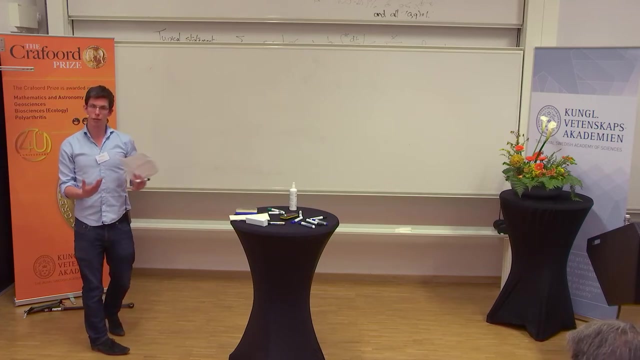 So that's one reason that the Bombier-Wingard of them is very powerful, that it sort of uses It allows you to have a substitute for grh. Another key reason is that this kind of quantity of result about primalt in arithmetic progressions. 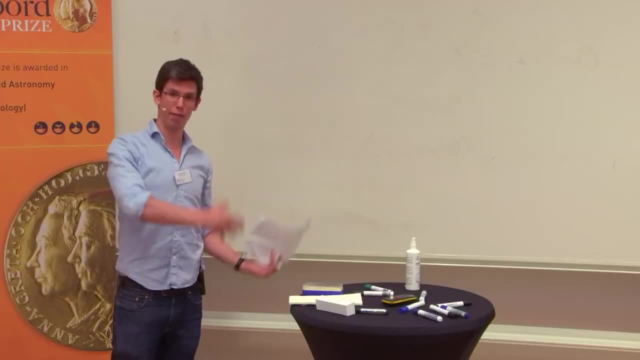 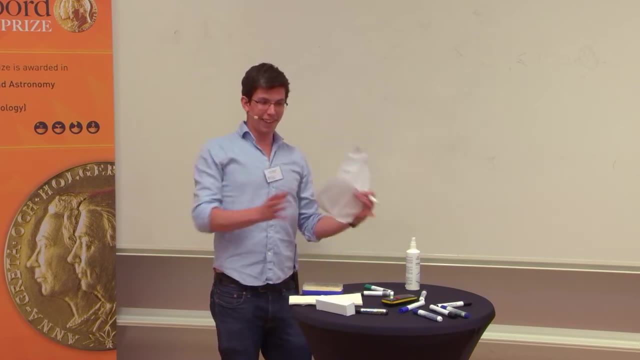 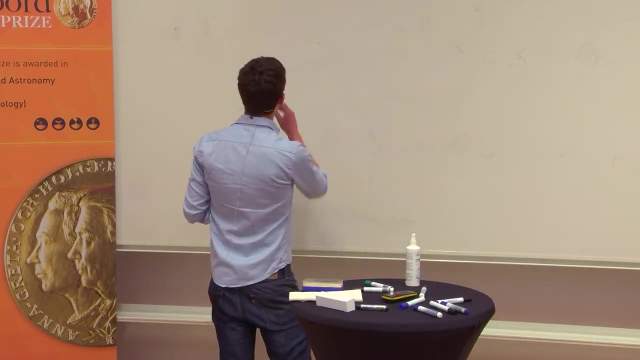 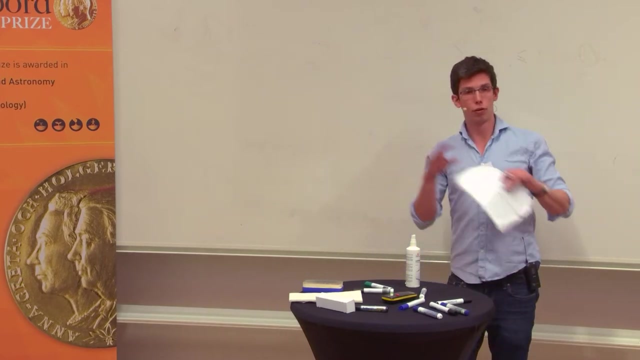 turns out to be an absolutely vital input to sierreff methods. So sierreff methods in general, a sort of- It's a kind of collective noun for a number of different sort of techniques that apply in different contexts, But the way that I like to think of them is as tools that convert certain types of arithmetic information. 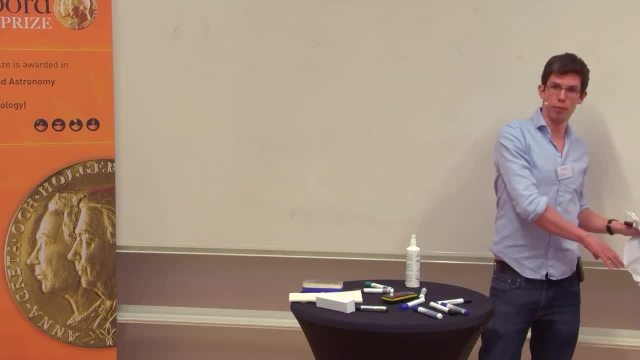 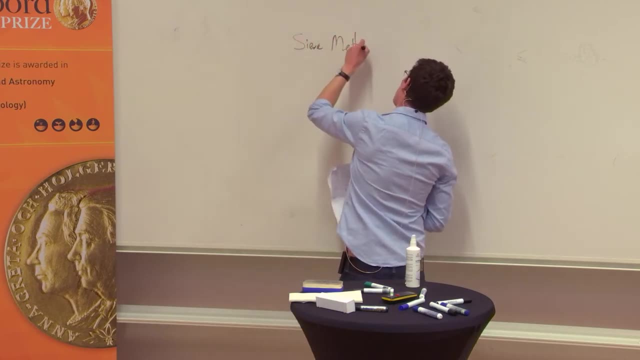 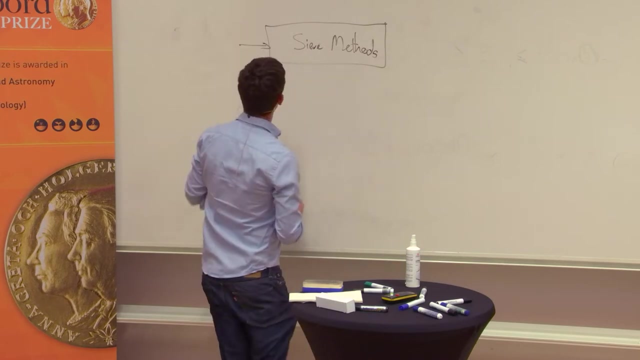 maybe about a set or a problem- into other types of arithmetic information. The picture that I like to have in my head is that civmethods are a set of tools in arithmetic number theory and you're interested in maybe trying to count primes or some other objects like primes in some set. 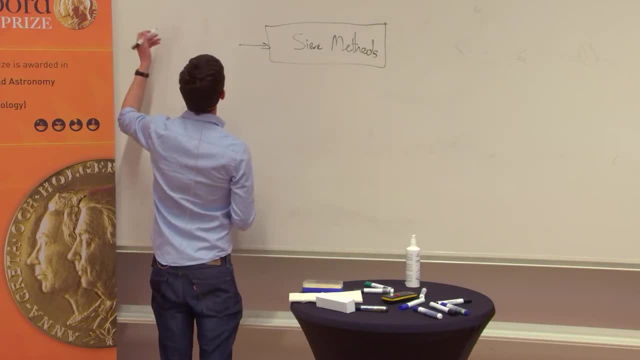 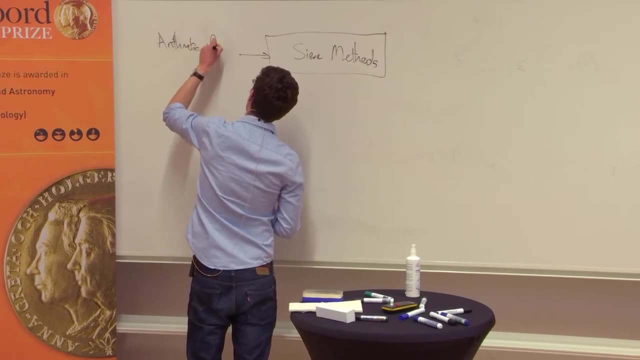 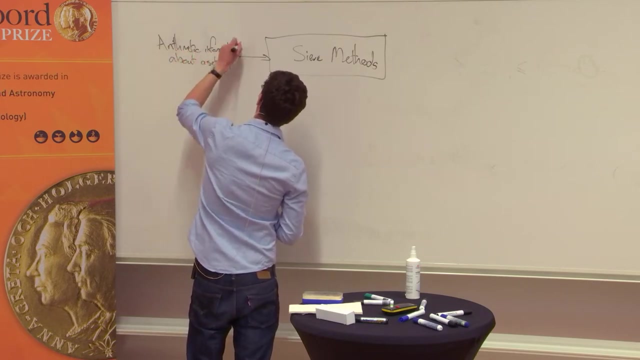 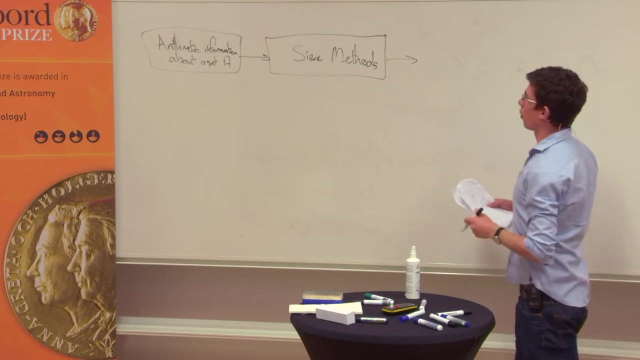 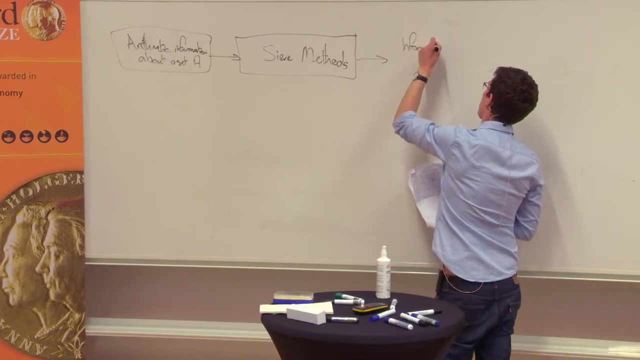 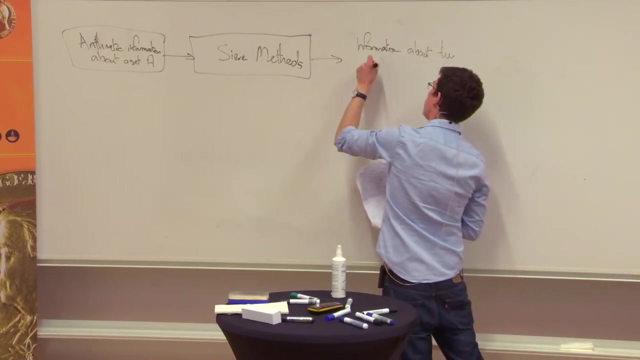 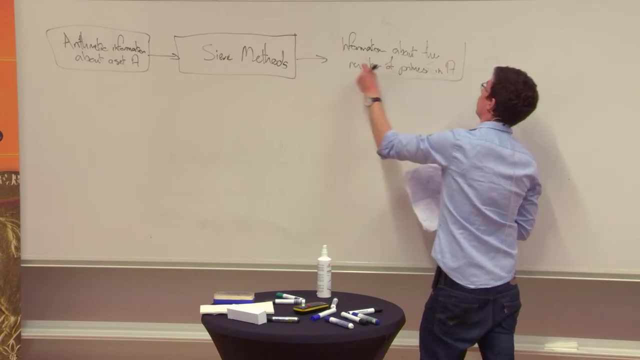 I'll call the set A, and it takes in some arithmetic information about a set A and it converts this arithmetic information into some other arithmetic information about the set A, So information about, let's say, the number of times. So you take in some arithmetic information. 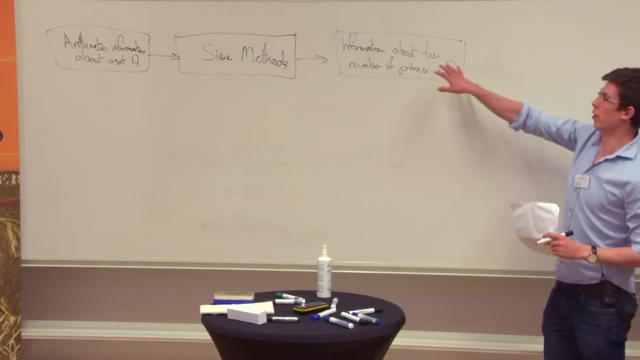 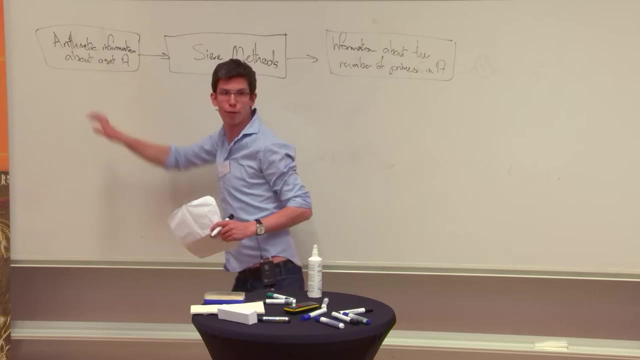 and you use the SIV methods to convert that information into the information about the number of times. And obviously this is useful when this is the sort of information that you can prove and this is the sort of information that you're interested in. 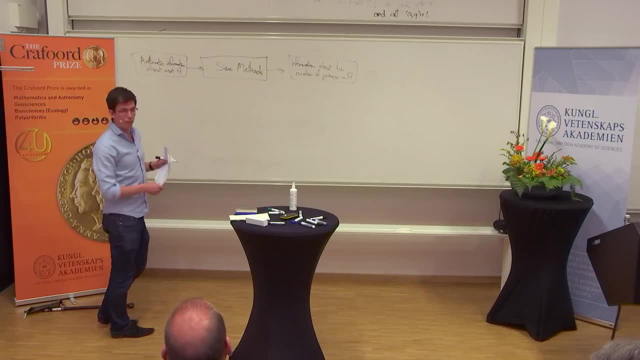 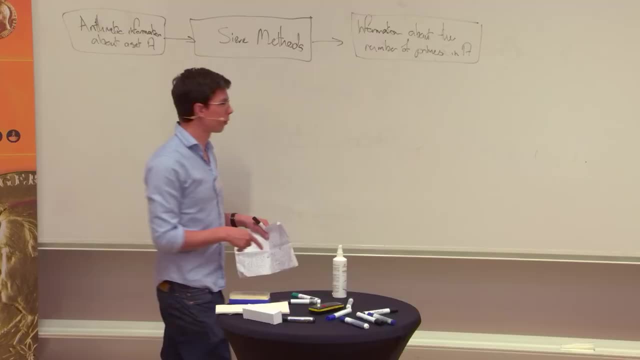 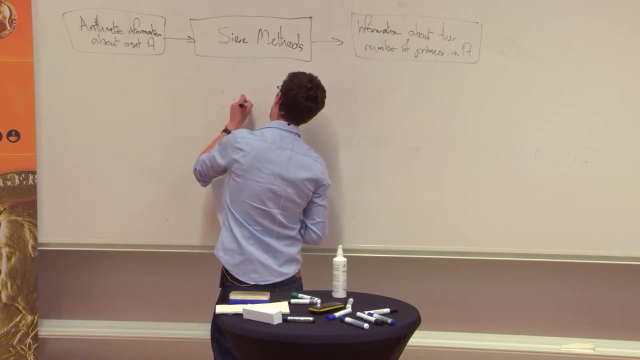 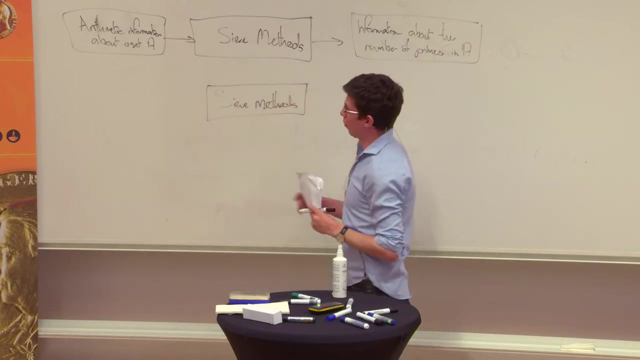 And so, in particular, Enrico mentioned in his talk the question about gaps between primes, And so this is certainly something where SIV methods have been successful, And so, in that context, the sort of arithmetic information that often you're interested in, 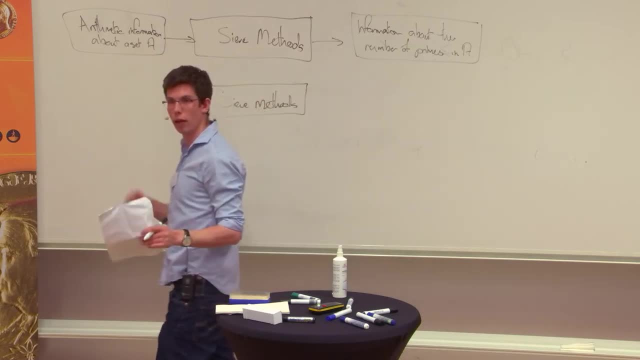 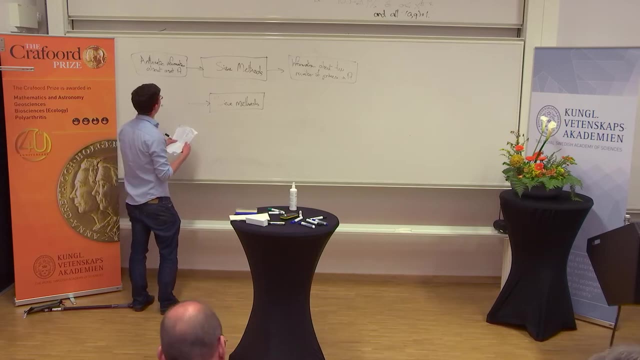 is the distribution of the set A and arithmetic progressions and maybe some other sorts of things. And so for the question of small gaps between primes, at least after the work of Goltz and Pintz and Yildirim, 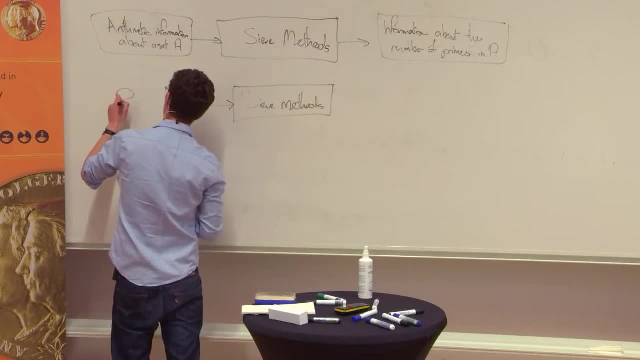 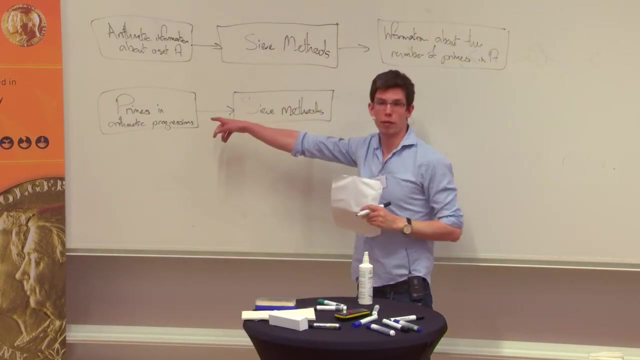 the typical way of studying this was via SIV methods and you take in as arithmetic information results about primes and arithmetic progressions, So exactly the sorts of results that the Bombay area vinegar got that Raddathium talks about. 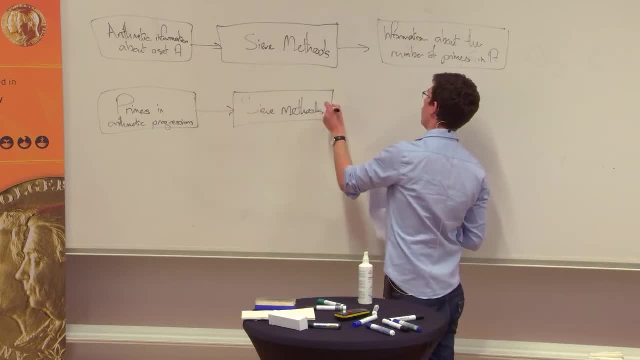 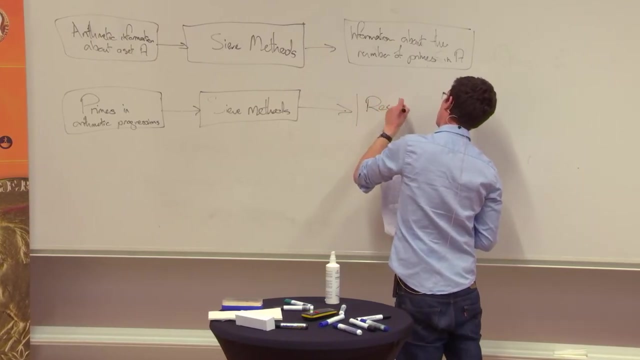 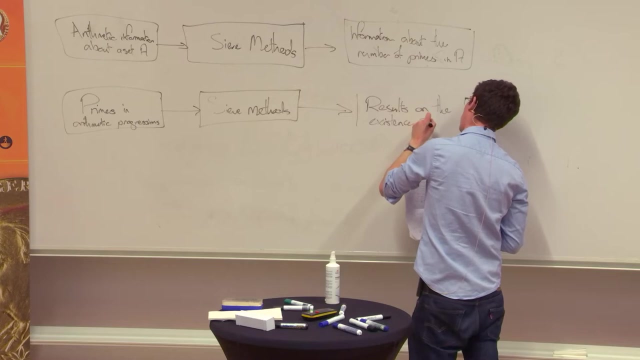 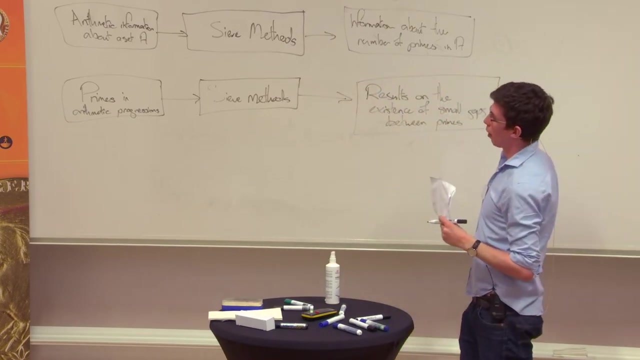 or the generalized dream hypothesis talks about, And SIV methods are these sort of combinatorial tools that allow you to convert information about primes and arithmetic progressions to results on small gaps between primes, The existence, And a key technical point is that somehow we know. 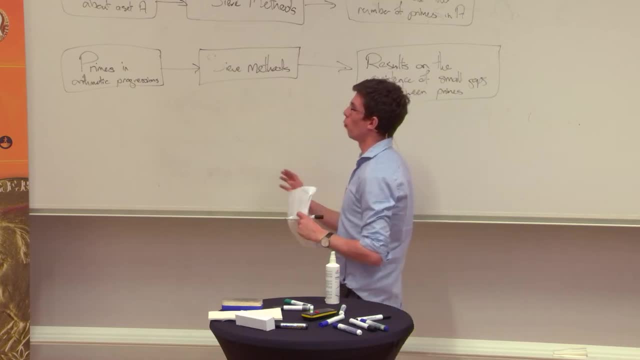 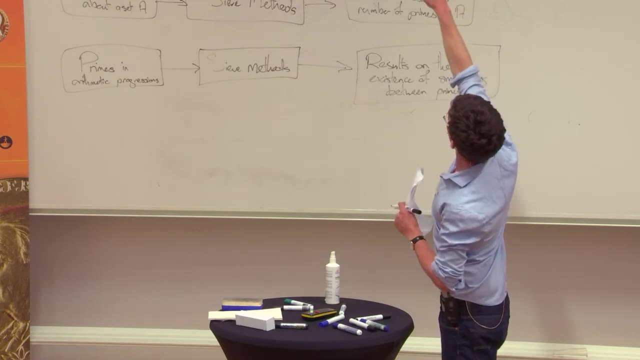 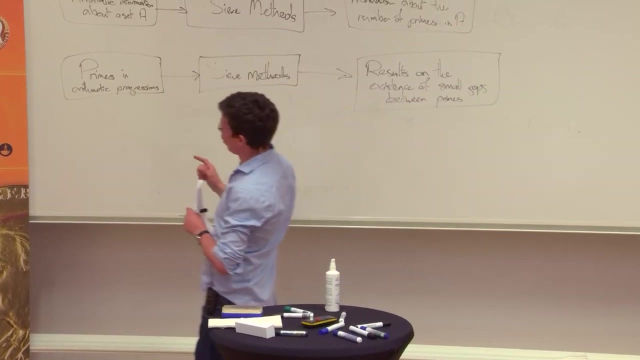 that this whole attempt at working like this would be completely useless. if you were limited just to the ranges of Q that we're limited to by the Z equals zero effect where Q is just of logarithmic size. But when you have something like the Bombay area vinegar Raddathium. 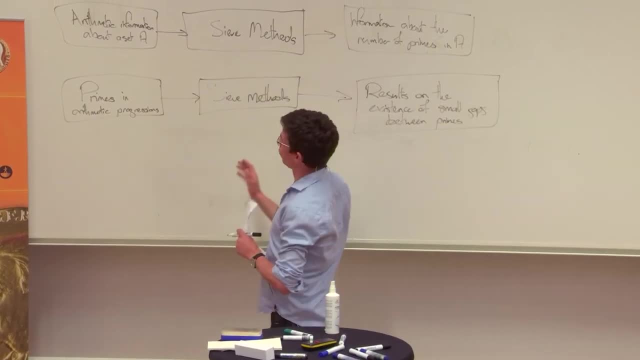 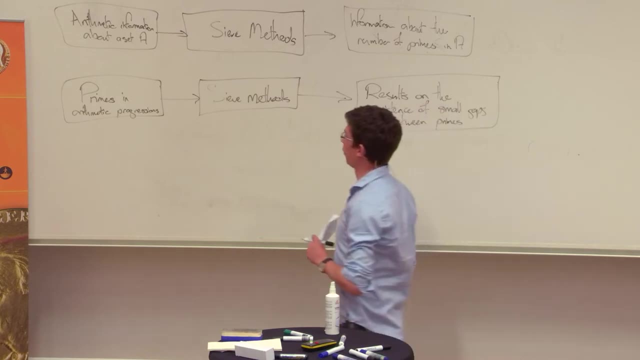 or the generalized dream hypothesis. when you can look at arithmetic progressions which are of size maybe roughly the square root of the size of the primes that you're looking at, or something like that, then SIV methods can be rather effective at converting results about primes. 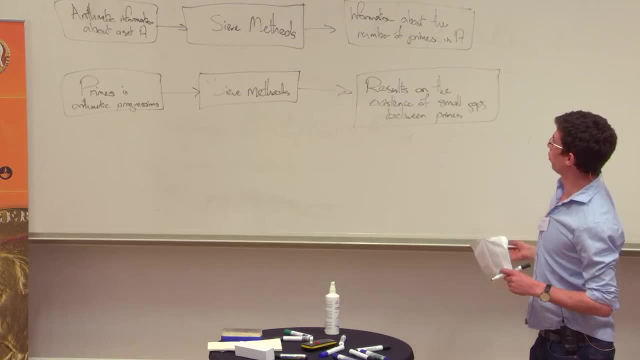 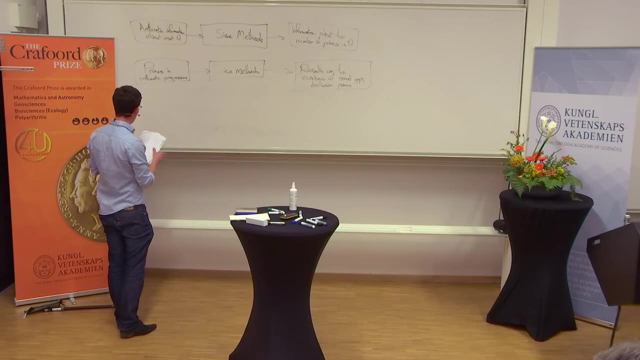 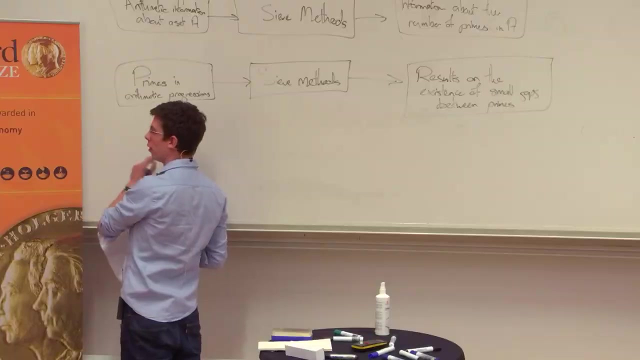 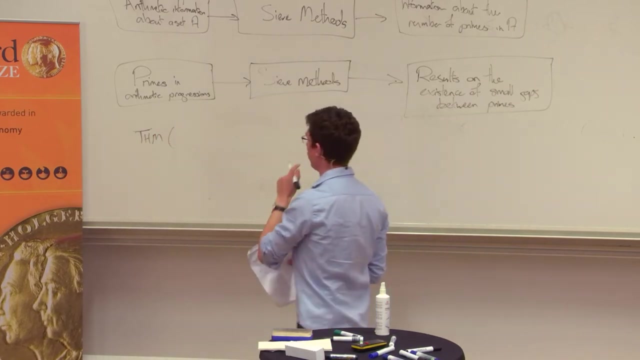 and arithmetic progressions into results on the existence of small gaps between primes And so, as Per mentioned, one set of results that I've been quite actively involved in now, sort of 10 years ago or so, but has been due to many different authors. 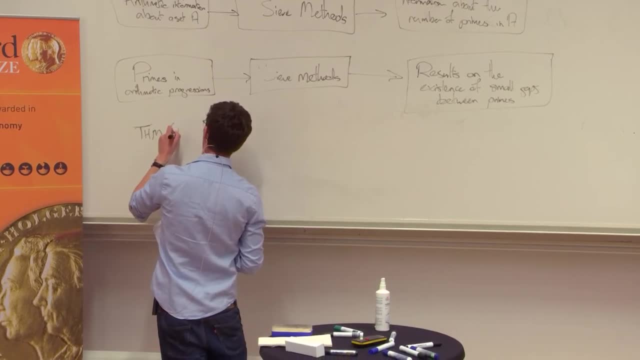 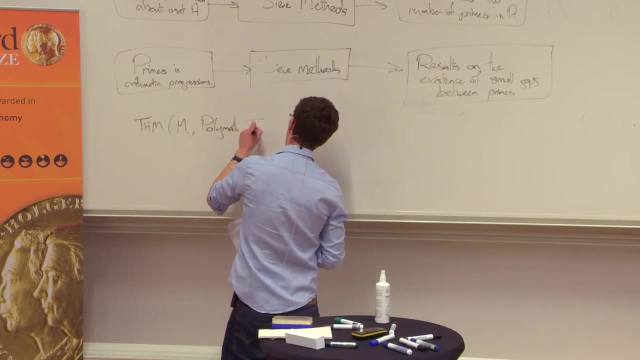 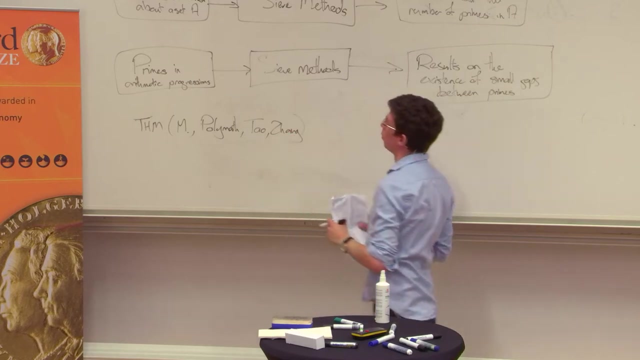 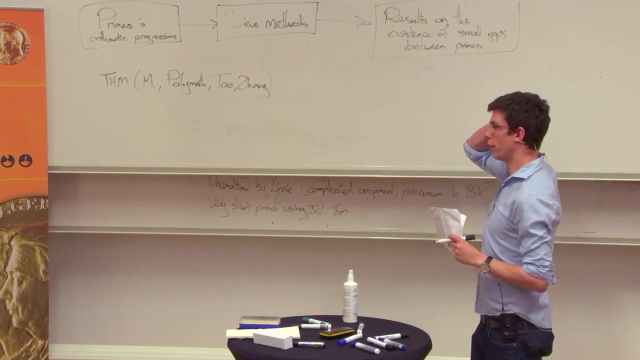 So, in no particular order, I'll put myself. there was the Polymath project, There was Tao and there was Zhang, And maybe the whole setup in this way was at least partly due to Golden-Pinson-Yildirim, although it certainly has lots of similarities. 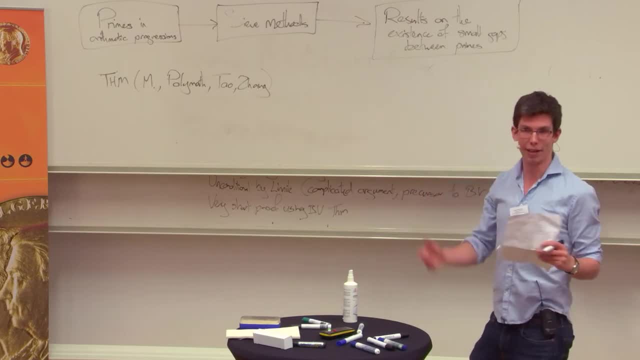 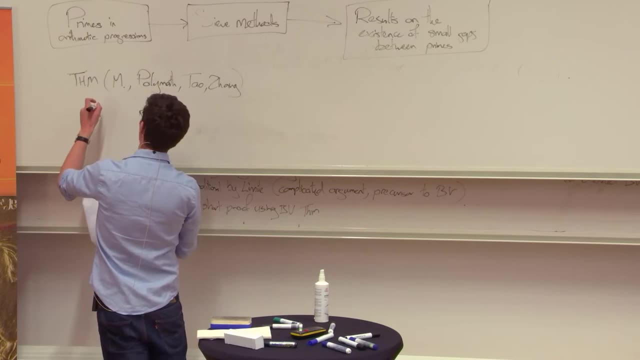 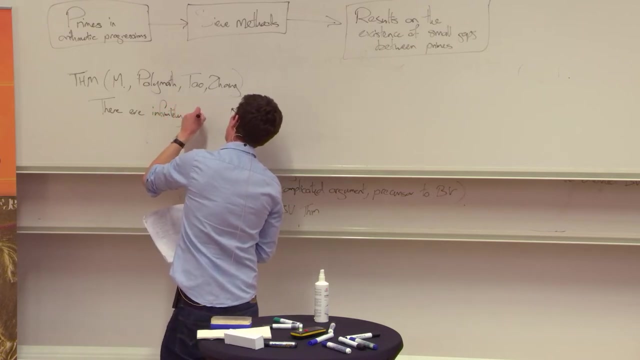 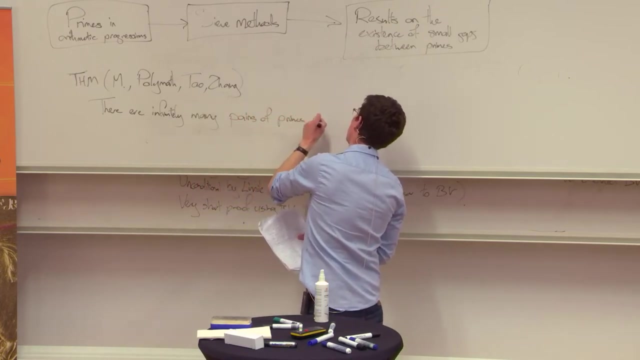 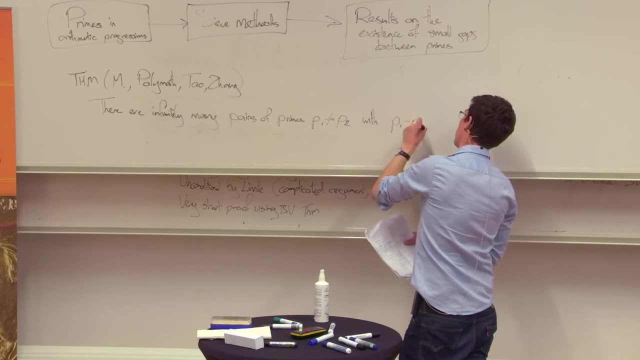 to the much earlier work, including the work of Bombay and Davenport that Enrico mentioned earlier on. And so this is: there are infinitely many pairs of primes, p1 not equal to p2, so distinct primes with p1 minus p2. 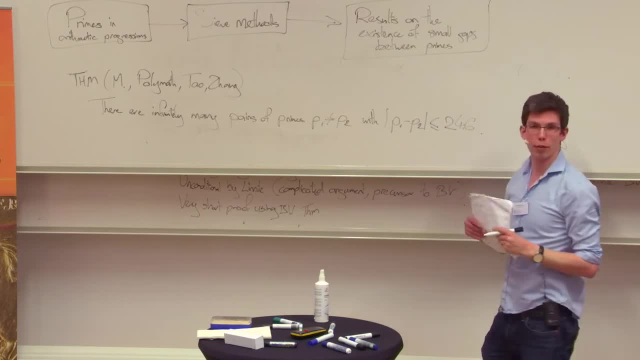 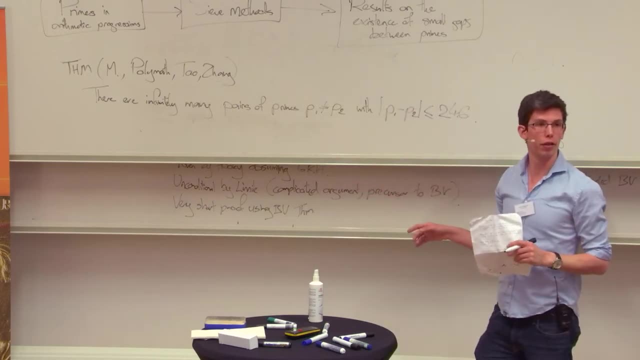 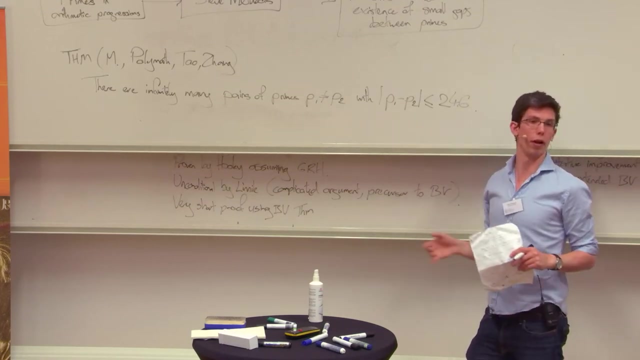 differed by at most 246.. So the famous twin-prime conjecture is the assertion that there's infinitely many pairs of distinct primes by exactly two. This is completely open, but as an approximation to that, you can look at pairs of primes which come very close together. 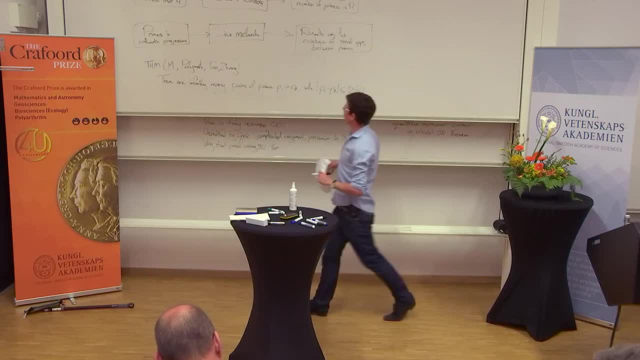 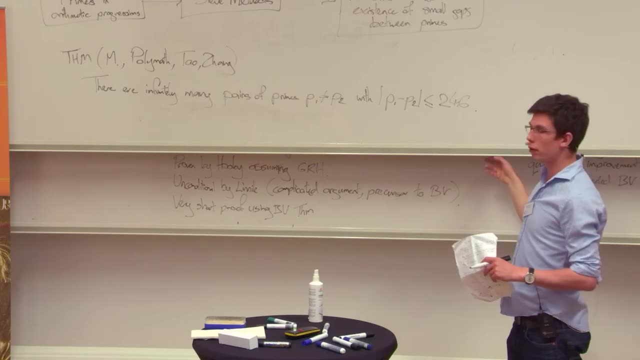 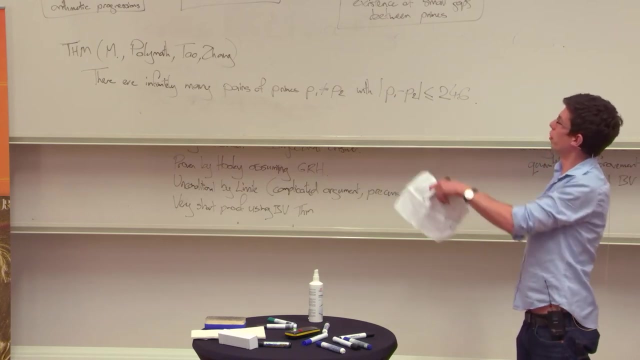 Until the work of Zhang, we did not know that there was infinitely many pairs of primes that differed by any finite quantity. We are now able to show that there are infinitely many pairs of primes that do come, unusually small, close together, and we cannot quite get down to two. 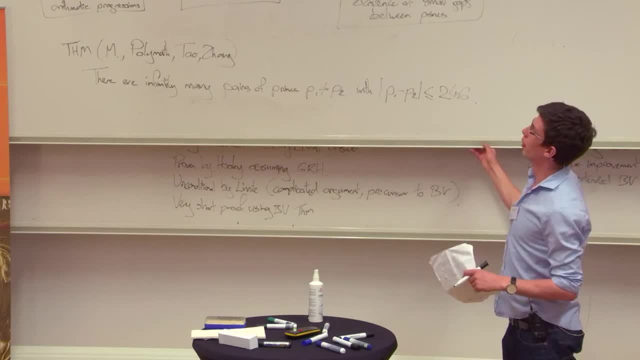 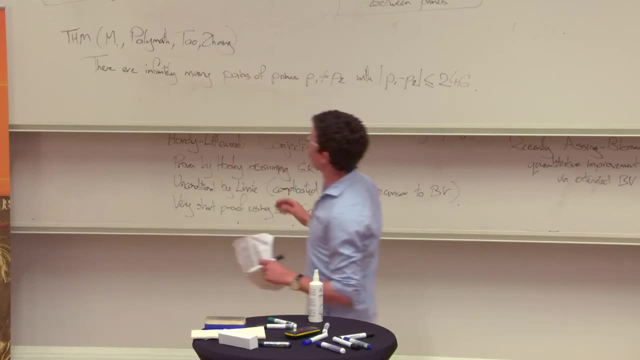 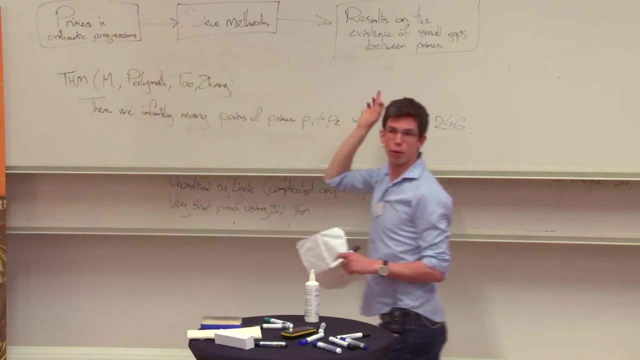 but 246 is some sort of quantitative approximation of two At least. so Zhang's work, the key input to that was about trying to improve the arithmetic information that went into this sort of argument, and so the default arithmetic information that would go in would be the Bombay-Ever-Nagano theorem. 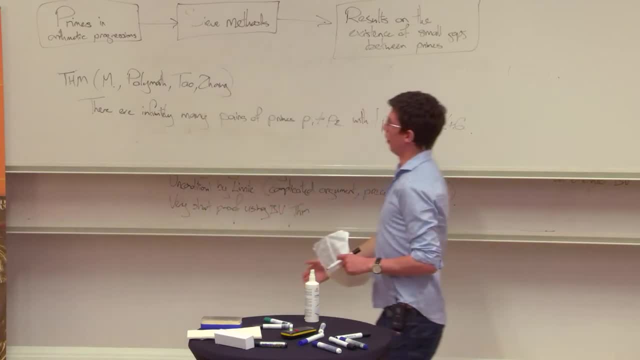 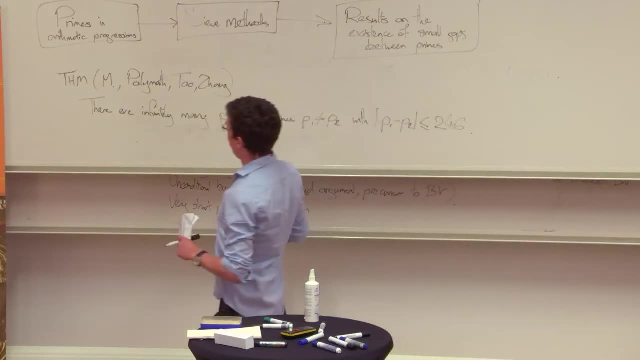 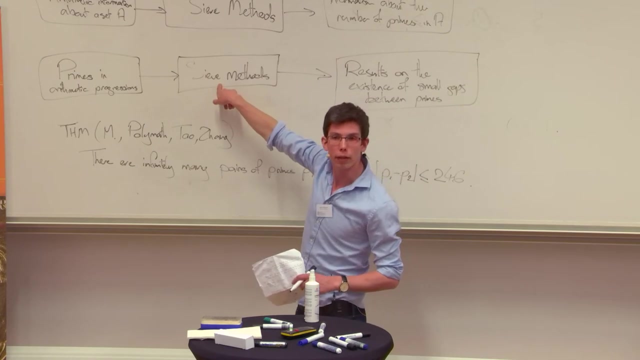 and he had to prove a technical extension of the Bombay-Ever-Nagano theorem that allowed him to show that there is infinitely many pairs of primes that differ by some bounded amount. The later work of Tao and I refined the sieve methods at the heart of this argument. 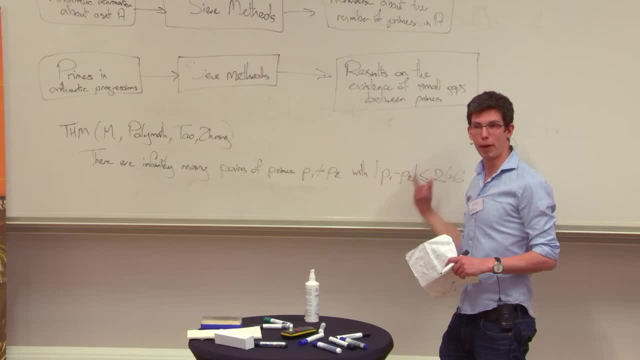 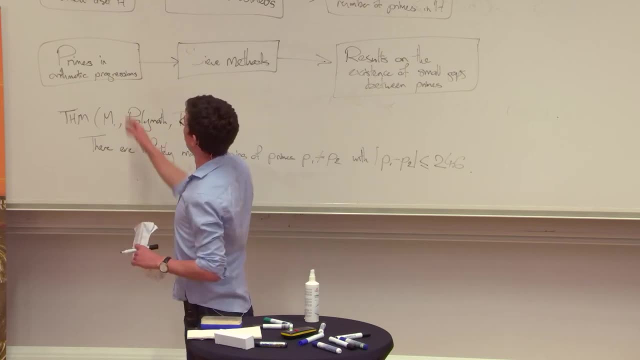 so it was more efficient to transfer this arithmetic information, and that meant that actually we did not need Zhang's technical extensions of the Bombay-Ever-Nagano theorem, and so just the Bombay-Ever-Nagano theorem itself was the key, unconditional input that we used. 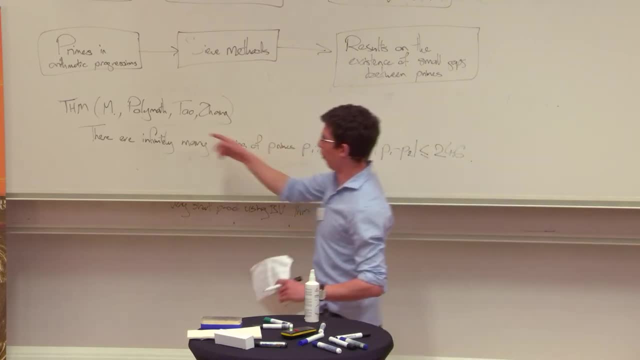 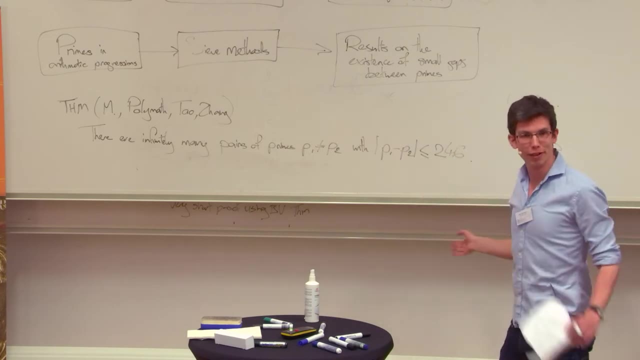 to show this, combining it with sieve methods. and then the Polymath project was about trying to quantitatively optimize things and get as small a constant here as possible. 246 is the number that came out after various bits of numerical optimization. 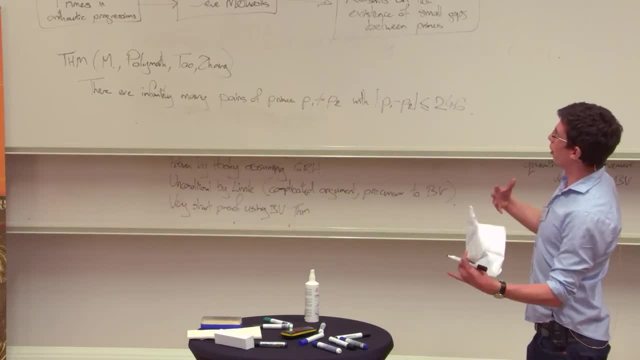 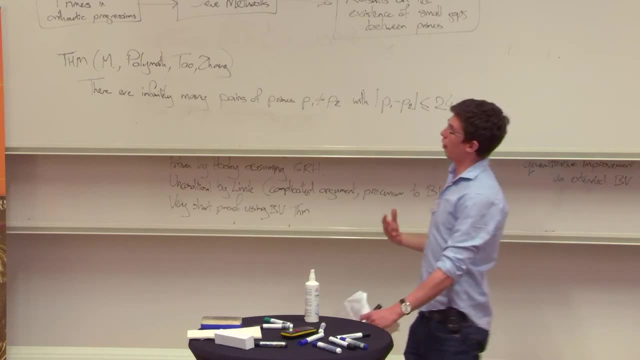 But again, this is highlighting very much how the Bombay-Ever-Nagano theorem is absolutely vital for the whole of sieve methods, that it is the kind of key input that goes into the Bombay-Ever-Nagano theorem, This whole field, and, depending on the sieve method. 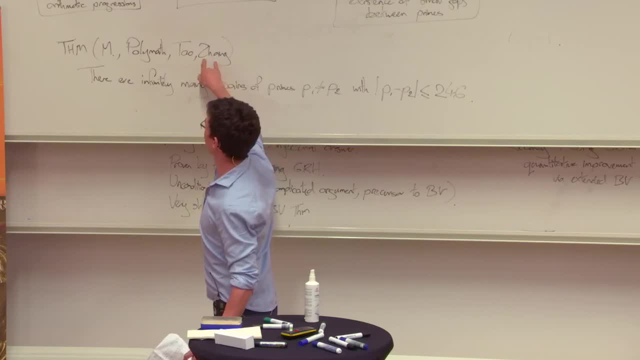 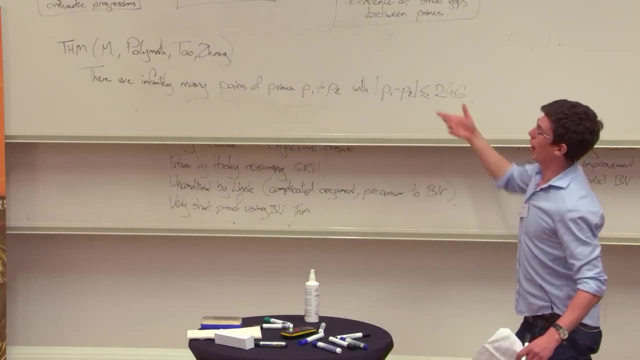 you are using. maybe you need a technical extension of the Bombay-Ever-Nagano theorem, or you can use a slightly more efficient sieve, but then the Bombay-Ever-Nagano theorem itself can be the powering thing. But even relatively recent advances in arithmetic number 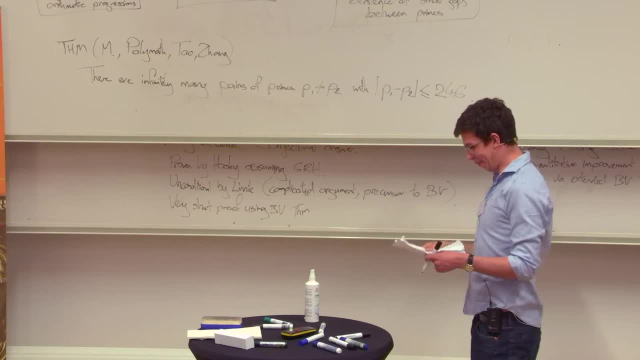 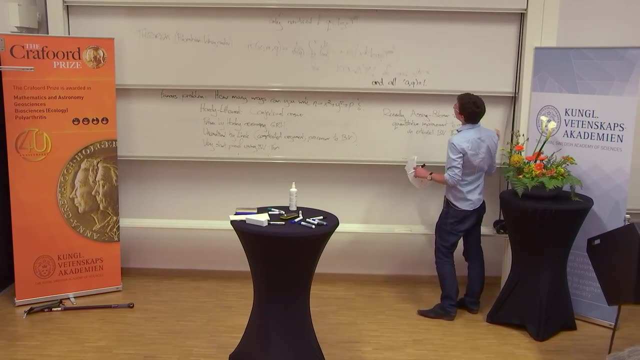 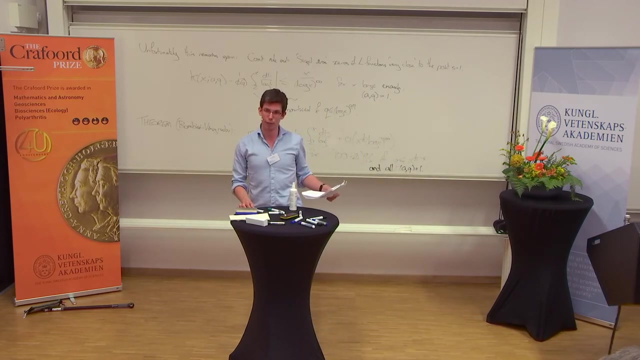 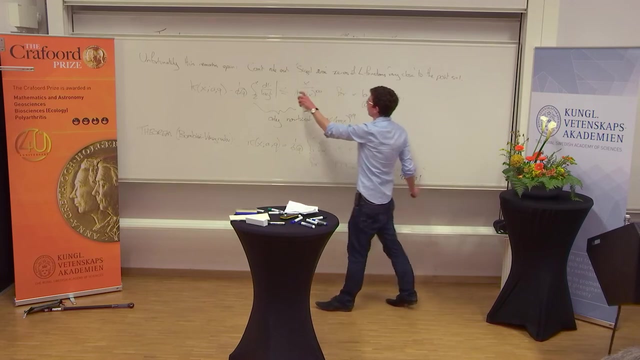 theory are still fundamentally relying on the Bombay-Ever-Nagano theorem as the key input. So maybe my first favorite result of Enrico is the Bombay-Ever-Nagano theorem, But my second favorite result that I thought I would also talk about here- 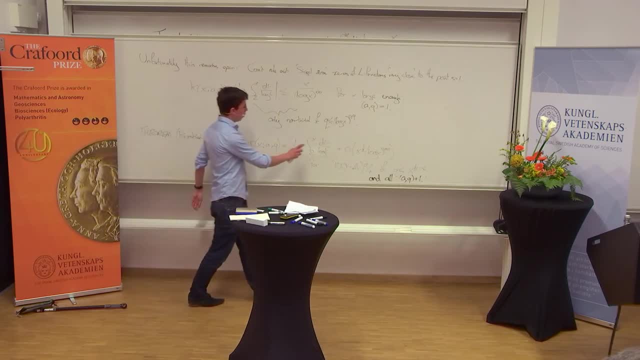 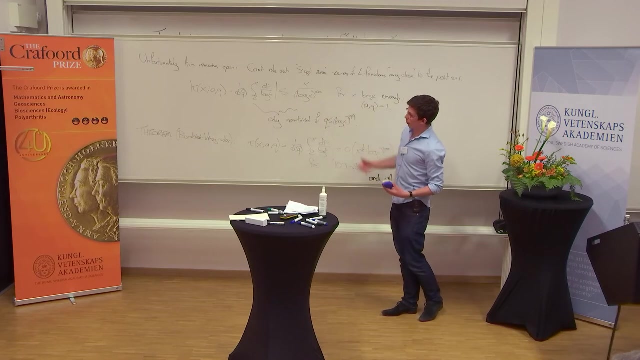 is a closely related result that's joint with Henrikh Ivanić and John Friedlander, which goes beyond the Bombay-Ever-Nagano theorem. It goes beyond the Bombay-Ever-Nagano theorem and in fact goes beyond the reach of the generalized dream. 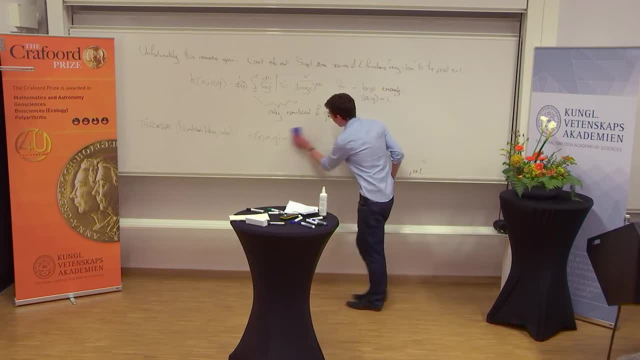 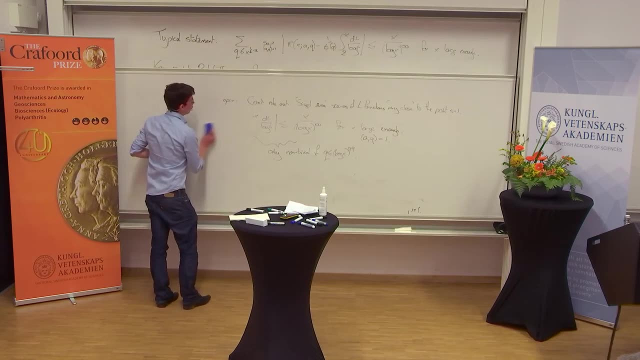 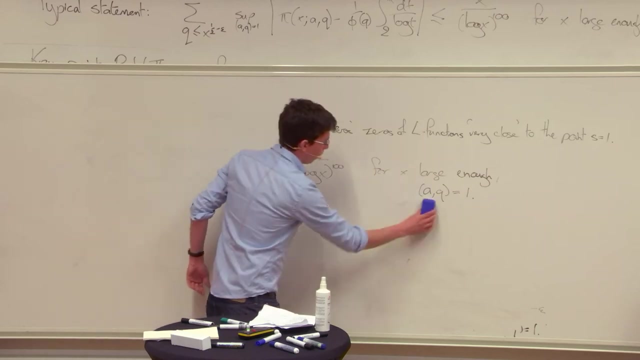 hypothesis. So in many ways the generalized dream hypothesis can be seen as a sort of slight roadblock in analytic number theory. that it's clearly an absolutely central conjecture, but we don't really have too many ideas about how to prove it. 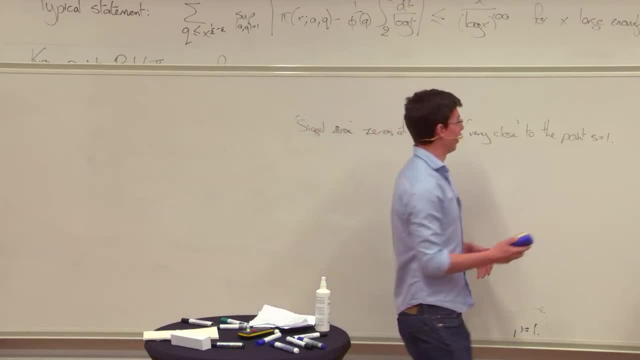 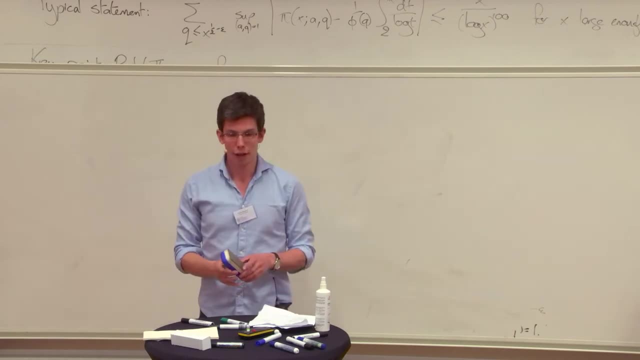 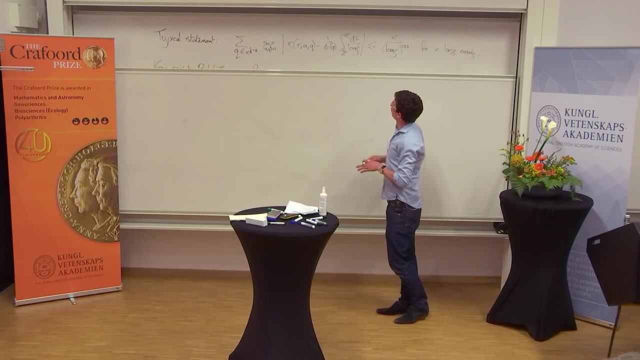 And so how can we make any progress beyond the generalized dream hypothesis if we are really stuck at proving it? But it turns out that, at least in these maybe lo-fi versions of the generalized dream hypothesis, for counting primes and arithmetic progressions there's no terribly natural reason. 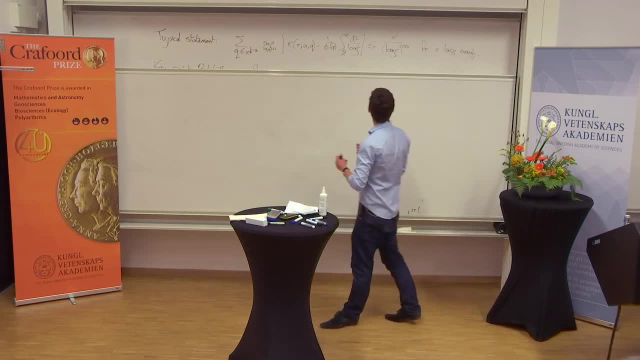 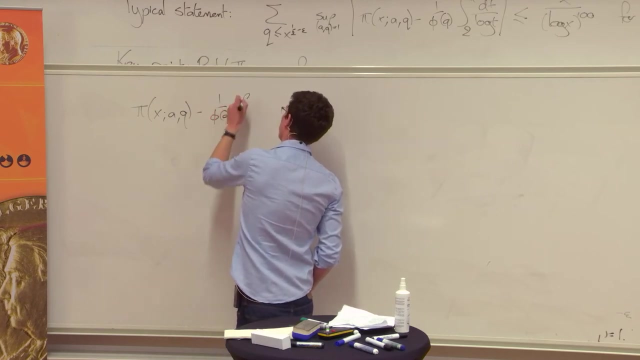 to be limited to the ranges that we were talking about before. So, if you remember, we were talking about the generalization of the generalized dream hypothesis. I said that the generalized dream hypothesis was equivalent to the statement that the number of primes in arithmetic progressions has a very nice main term. 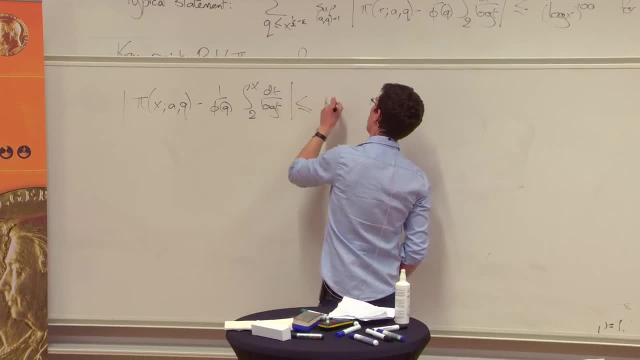 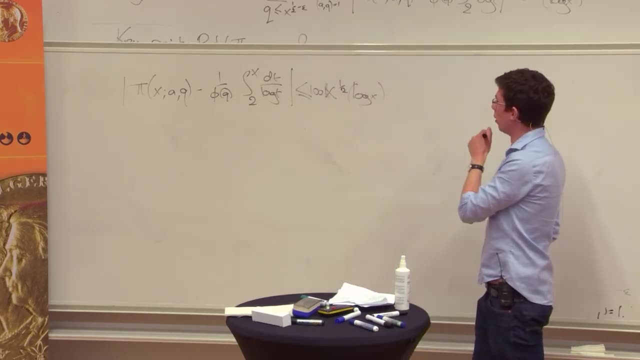 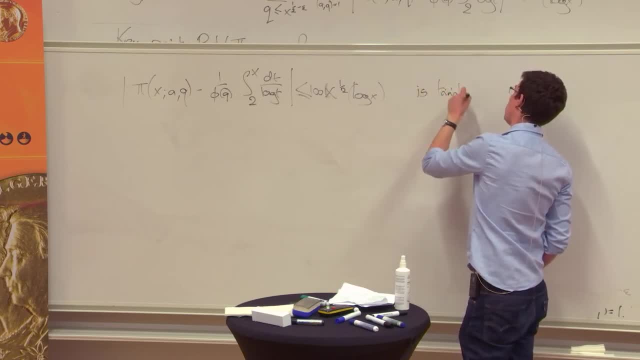 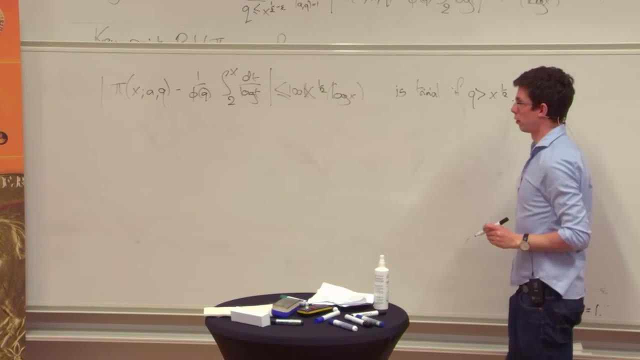 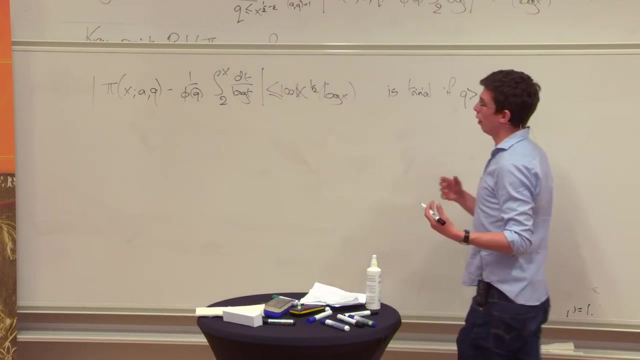 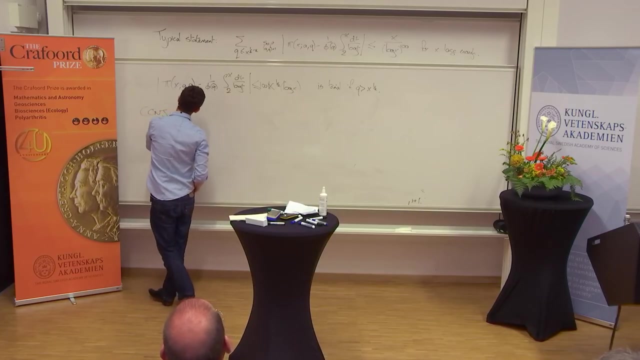 But this is trivial in this formulation if q is bigger than the square root of x, because this error term here would then be bigger than the main term, And so this wouldn't even be an approximation then. But it's conjectured that, despite the fact that this 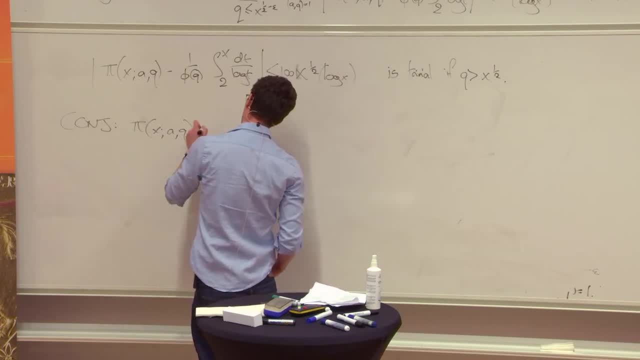 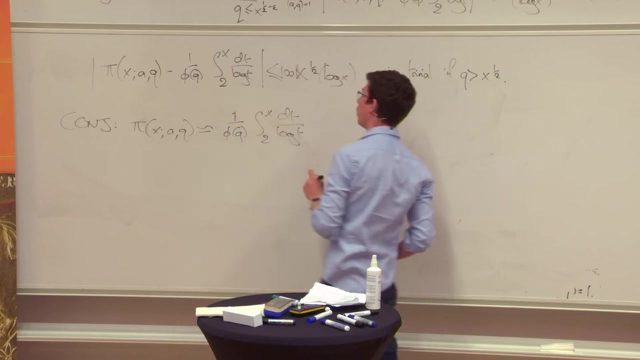 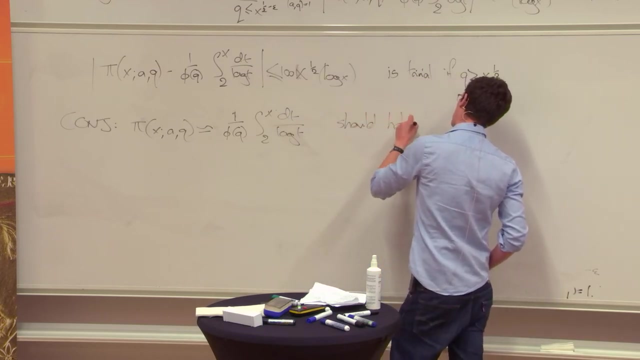 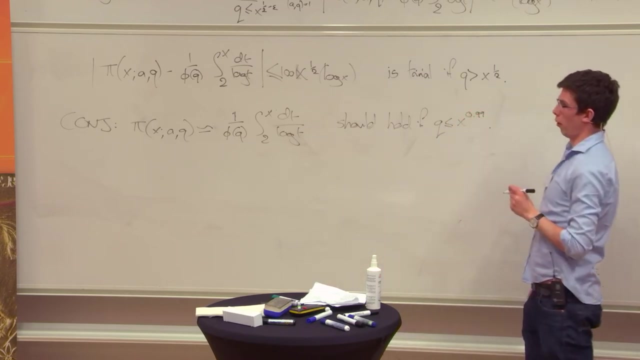 is well outside of the reach of the generalized dream. hypothesis that this should- maybe- I'll just write an approximate- equals that this sort of nice main term approximation should hold in a much wider range of q. So again, I'm just going to write down some explicit constant. 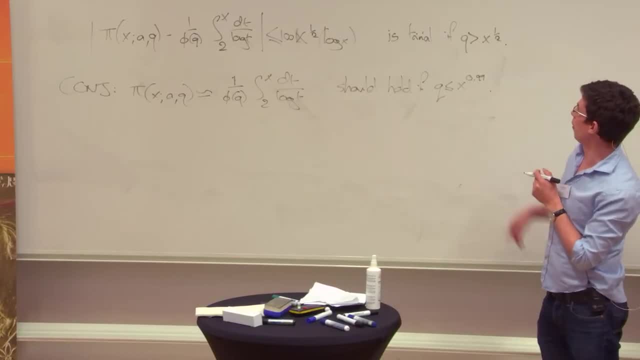 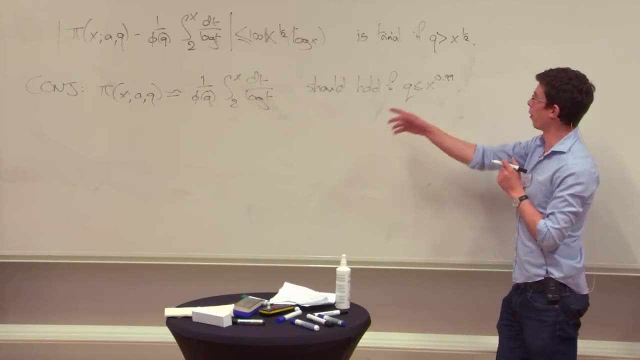 here for the sake of being concrete. So if q goes up to x, to the power 0.99,, then this sort of approximation should still hold. It's clearly going to break down if q is bigger than x And it breaks down in slightly technical ways. 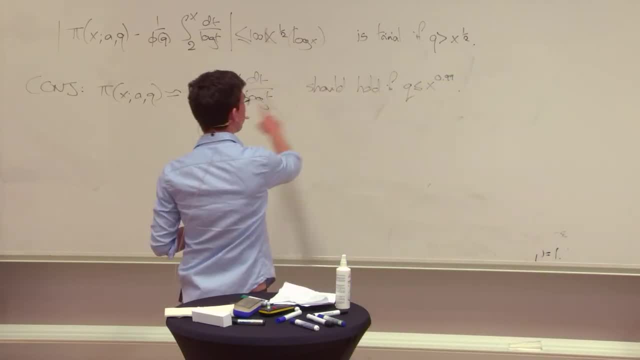 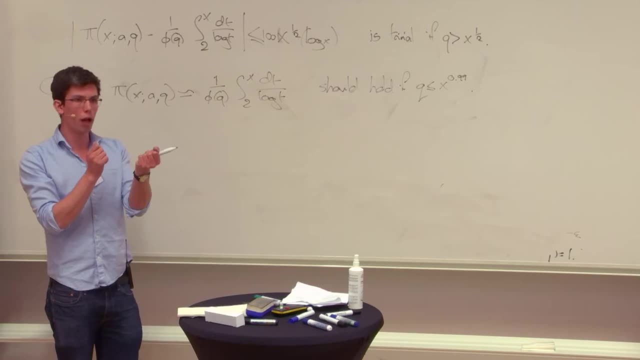 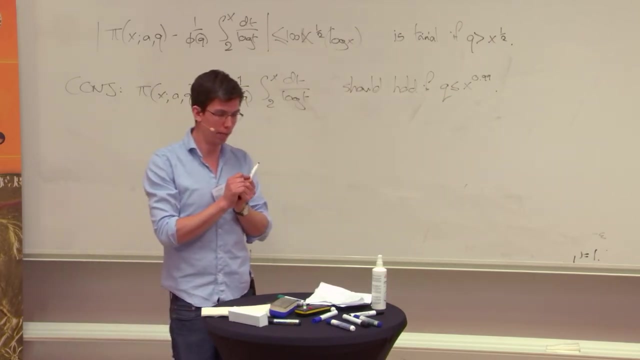 if q is close to x, And so this is somehow well outside of the reach of the generalized stream hypothesis. Morally, it would imply that there's equidistribution of zeros on the half line between different L functions, But this seems way beyond anything. 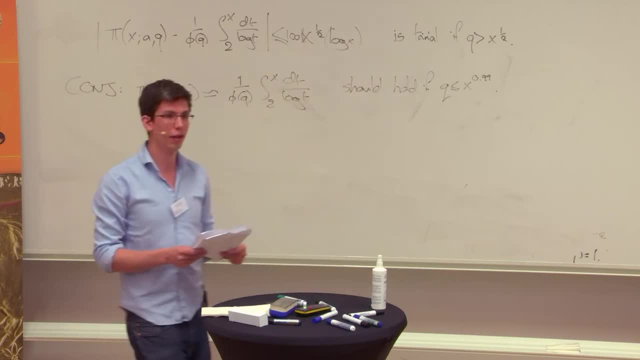 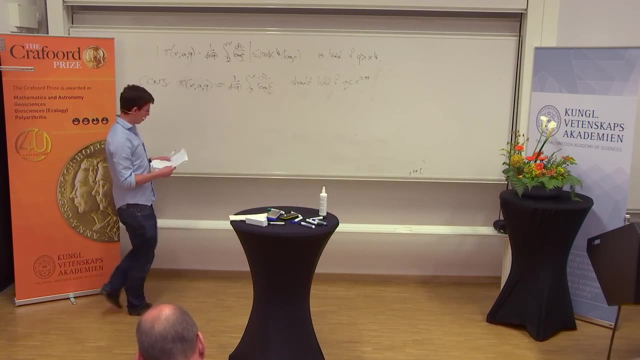 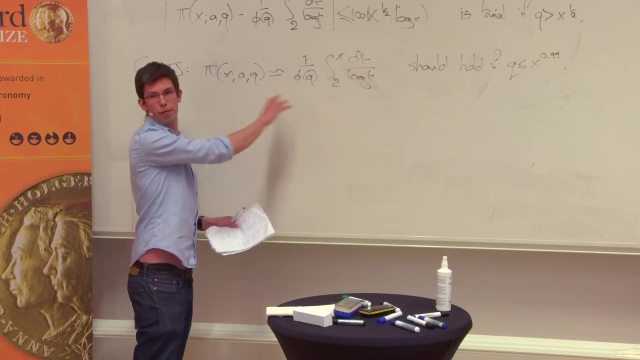 that we're even tempted to speculate on at the moment. So it seems well out of reach of things, even if you start assuming pair correlation of families of L functions and the distribution of zeros on the half line. But nonetheless we still expect this fairly natural conjecture. 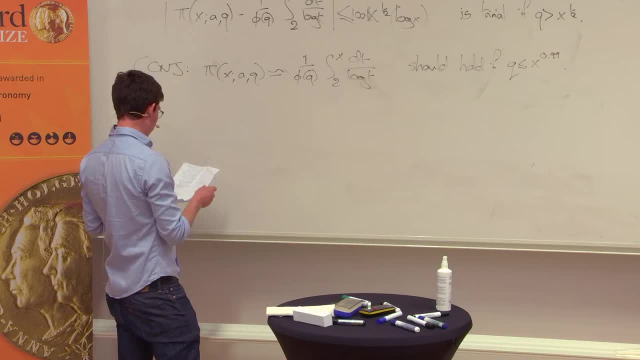 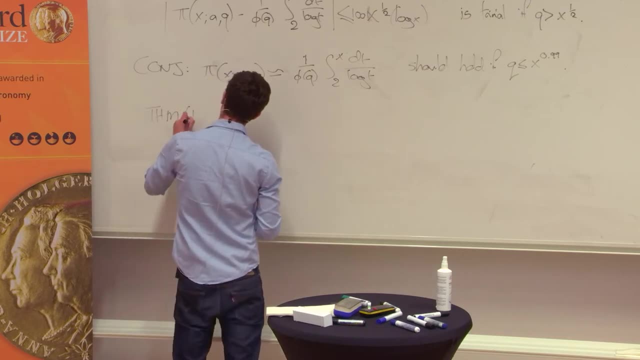 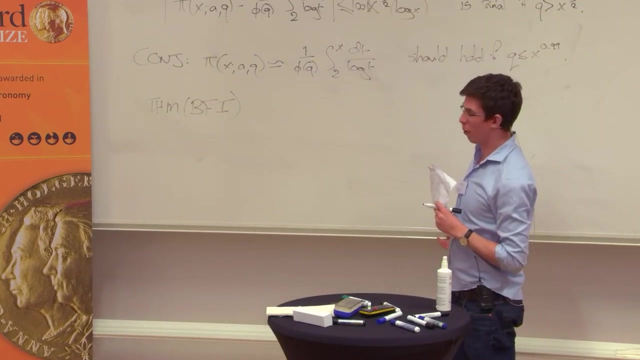 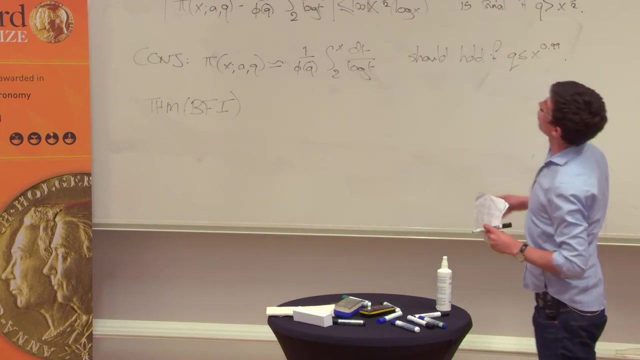 to hold And Maybe one result due to Bombieri-Freelander-Ranietsch- I'll write them, just as BFI- because that's how everyone refers to these results- says that you can get a version of the Bombieri-Vinogrado theorem, that's. 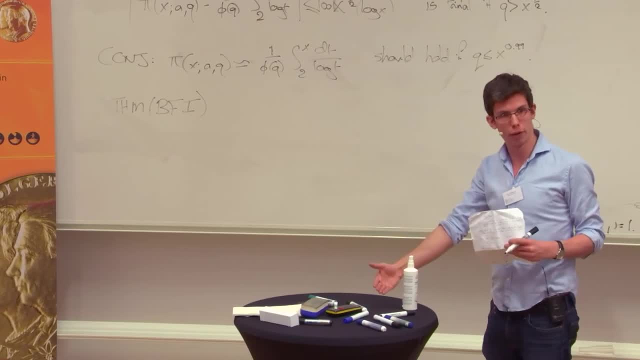 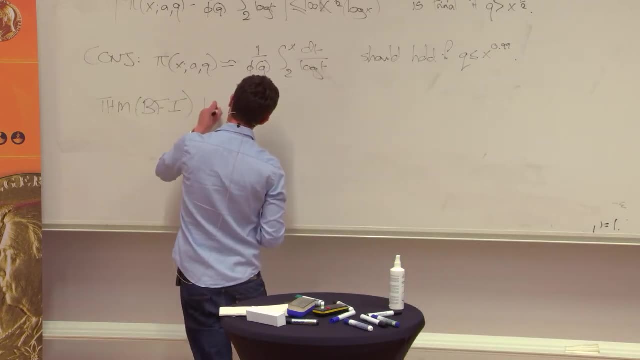 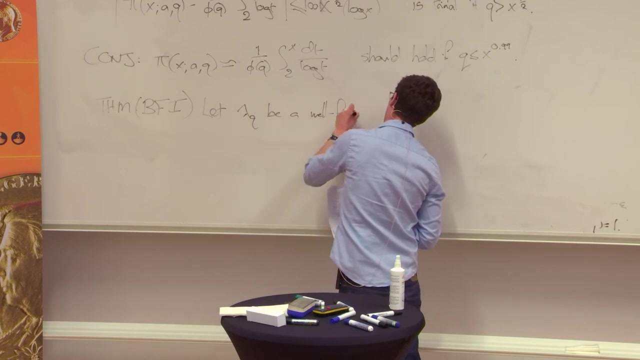 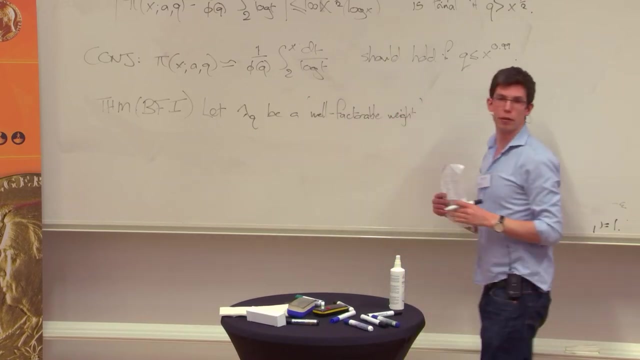 unconditional. that goes beyond this Riemann hypothesis, range of q being smaller than the square root of x. So Let lambda q be a well-factable weight, which is some technical condition that I don't really want to get involved in too much. 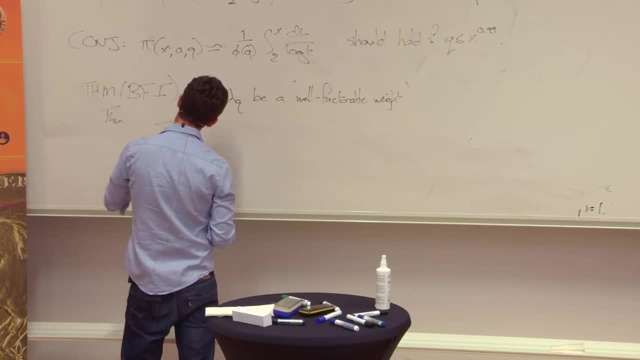 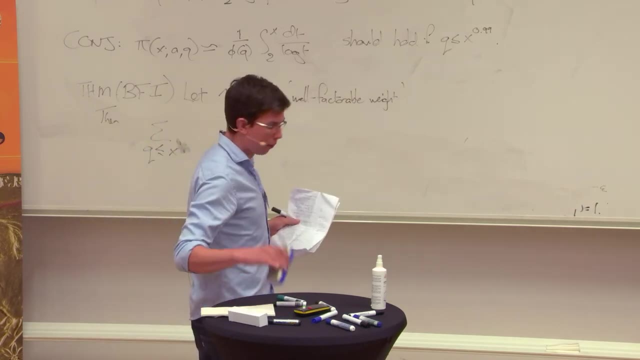 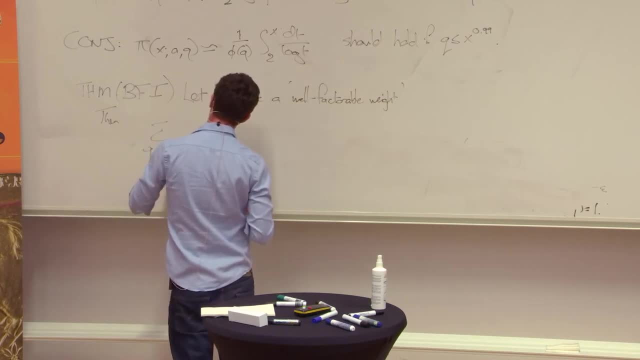 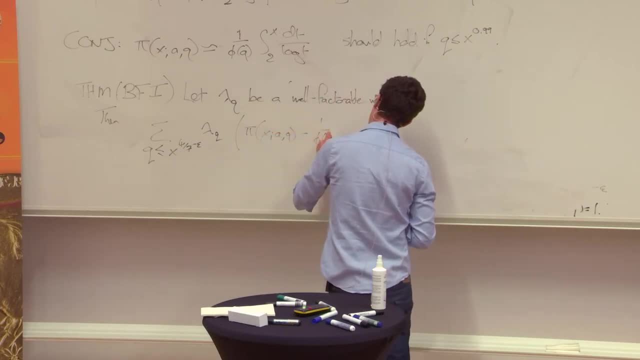 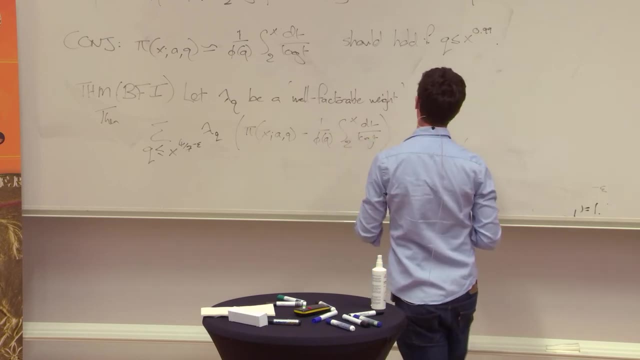 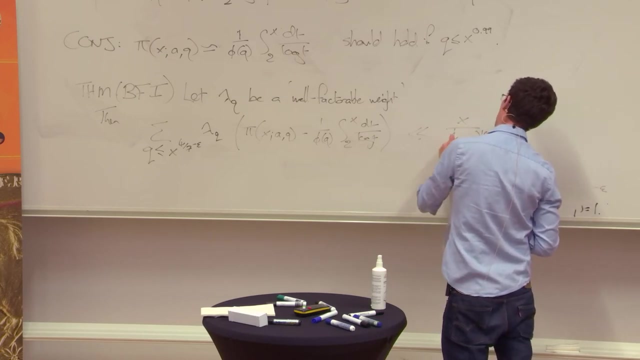 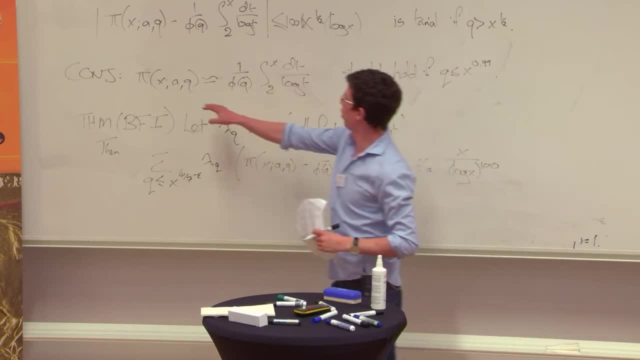 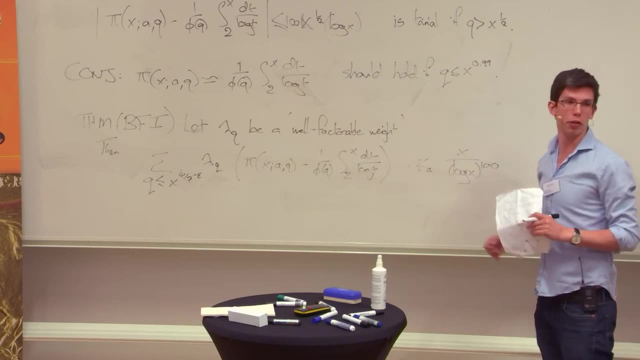 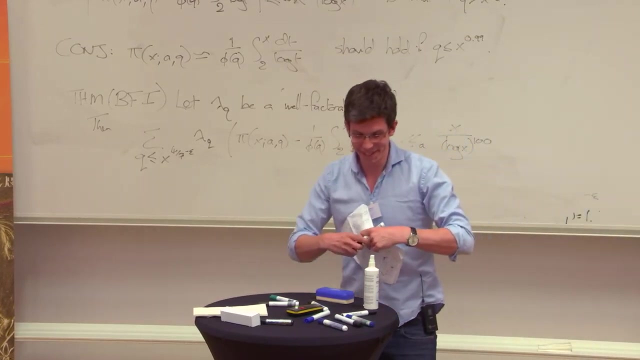 Morally. this is sort of saying that this conjecture Holds, in a slightly technical sense, Even when Q goes up to the. when Q goes up to the range X, the power for sevens it holds on average. I Trying to remember which pens I've used and which ones I have it, Maybe I'll move to a blue pen and see if that's clear. 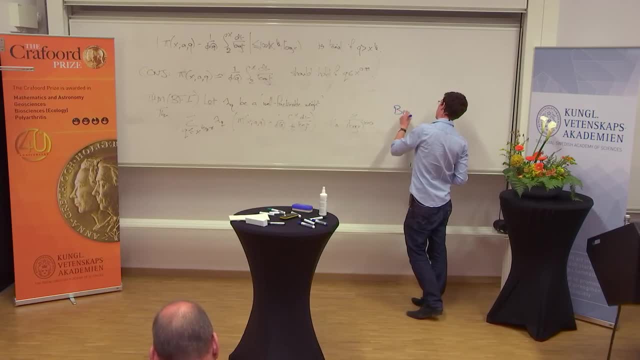 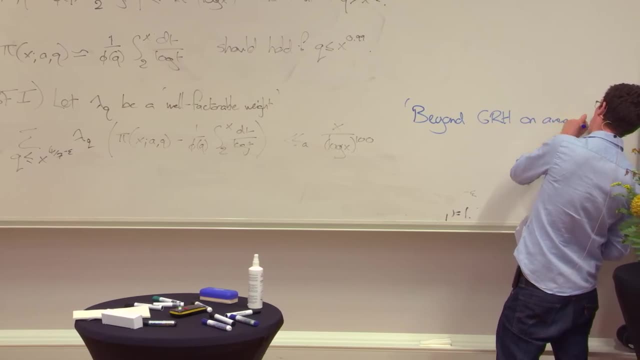 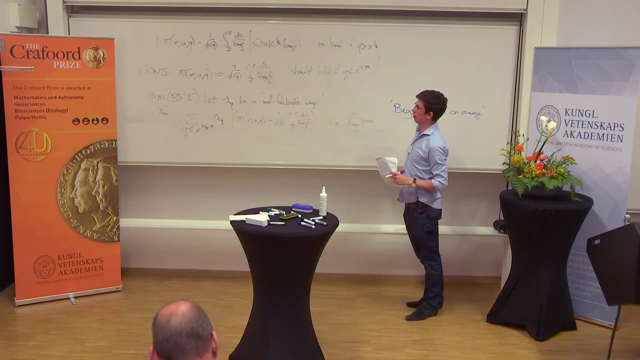 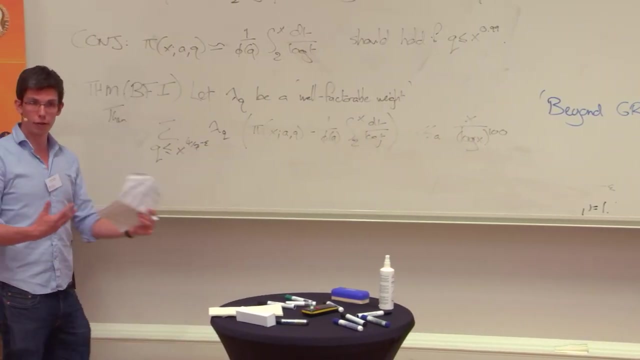 So this is sort of: oh, that looks much better Beyond grh on average. So the key point here is that for sevens is bigger than one-half, and It turns out for various results that this going beyond the square root barrier, so beyond the range of grh, is crossing some important qualitative threshold and 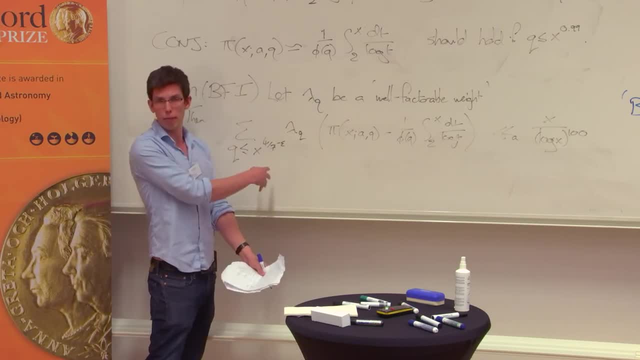 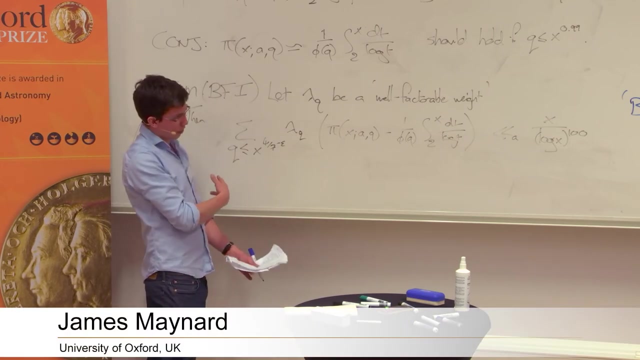 there's certain applications to the distribution of times and of other results of arithmetic significance Which finally rely on you going past this, just past this range of applicability of grh. so, as well as being a sort of proof of concept that unconditionally we can do things that go beyond the immediate, 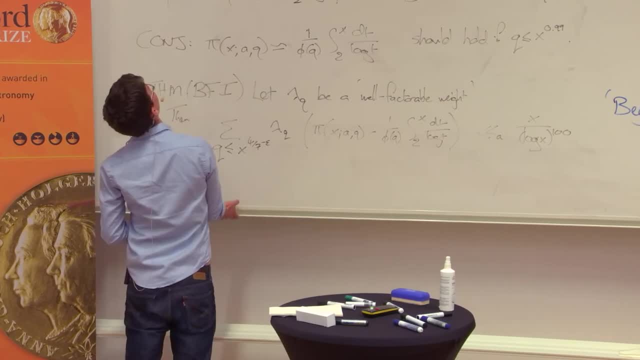 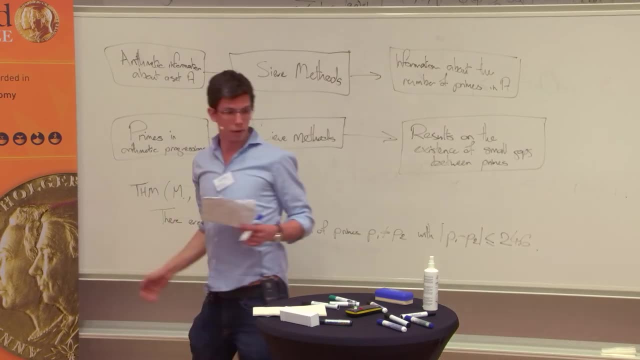 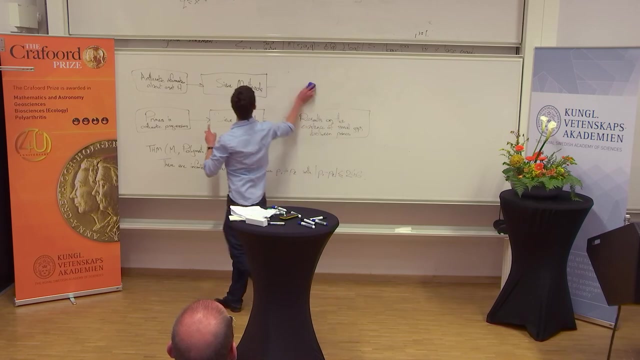 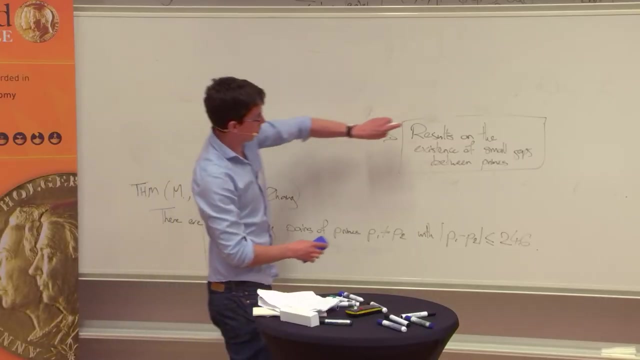 range of the Riemann hypothesis. This also has important arithmetic applications. Maybe I will just highlight a couple of those now. So I guess one thing is, as I mentioned, sieve methods, just as I'm raising here, often take results about primes in mathematic progressions. 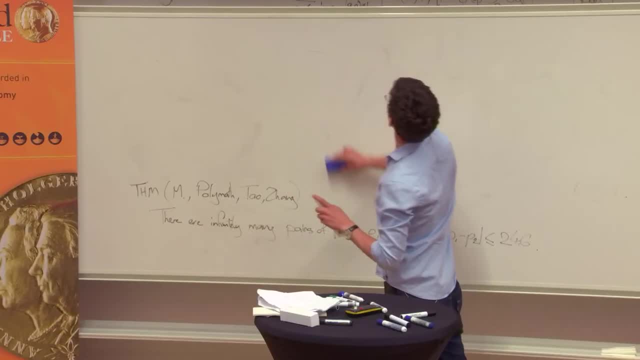 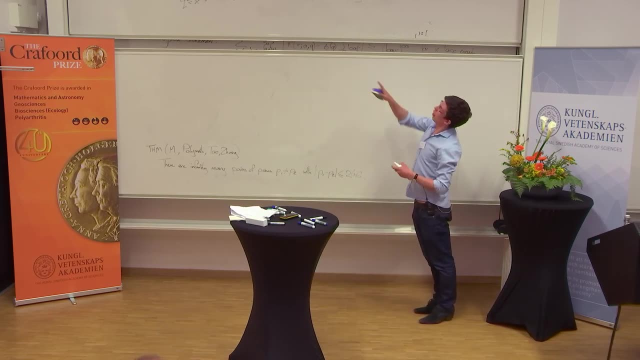 There's a a sort of black box arithmetic input, And so this is a technical result about times and arithmetic progressions that goes beyond the Bombier-Van der Garda theorem, And so just overnight this automatically improves a whole load of different results. 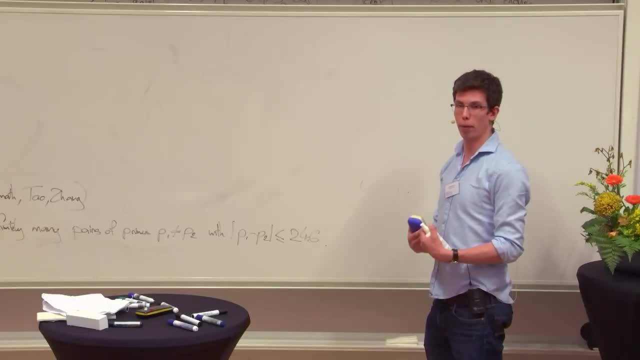 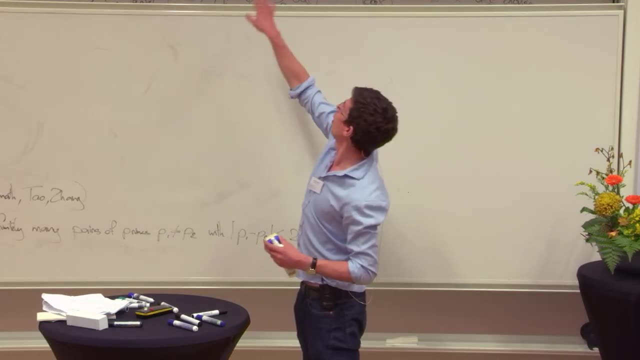 about coming out of SIV methods, because you can put stronger arithmetic information into the SIV methods and so you get stronger arithmetic information out. Because there's a slight technicality about well-factual weights and things you have to be careful about precisely which applications get improved. 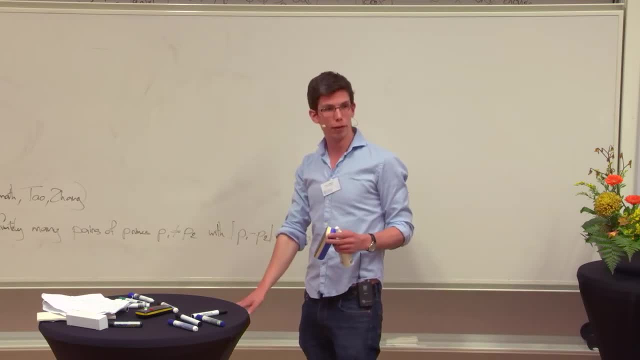 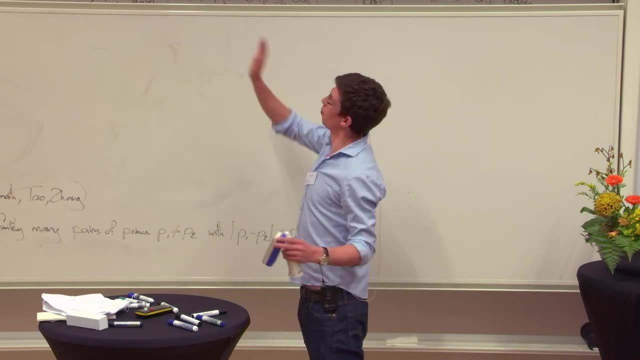 and don't get improved. but there's a huge number of results in SIV methods that just get improved overnight as soon as you have this statement, And there's lots of places where the constant one-half can just be replaced by a constant four-sevenths. 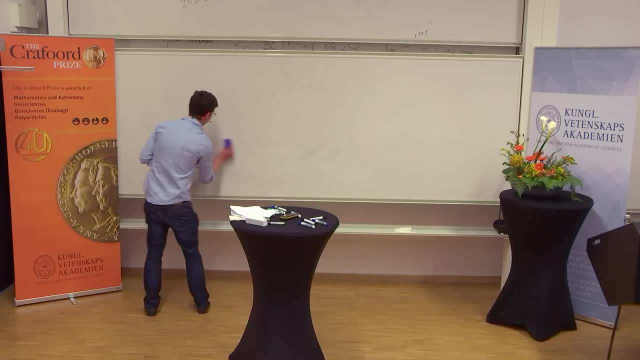 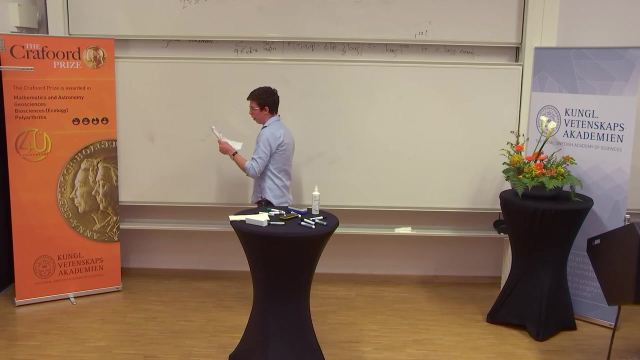 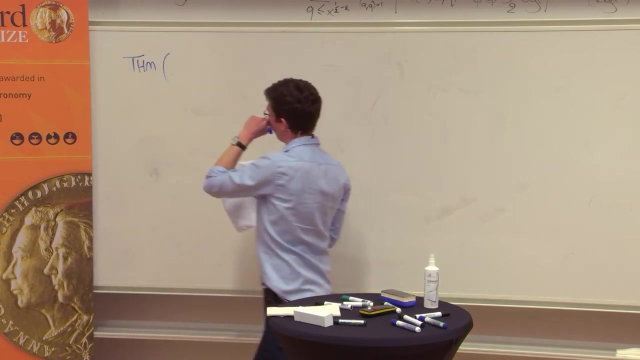 But maybe that just gives quantitative improvements and so it's an important psychological barrier that's been overcome, but less sort of fundamentally mathematically significant, But two results that really rely on going beyond this square root barrier. So maybe one result, the first one that I'll mention- 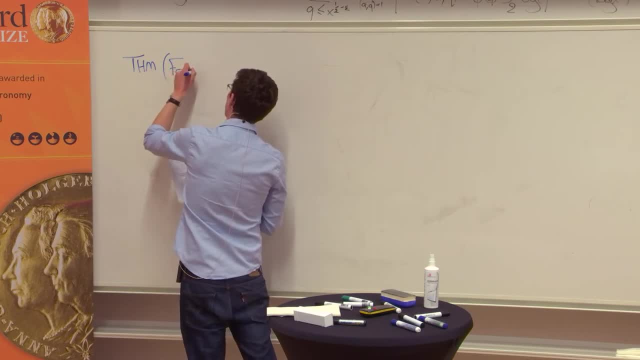 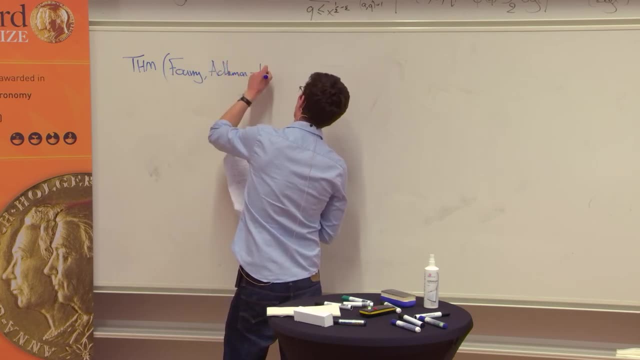 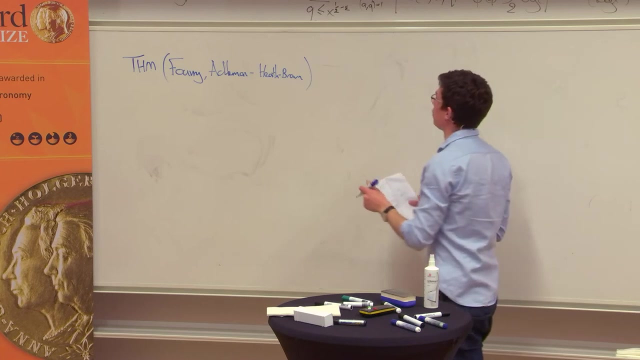 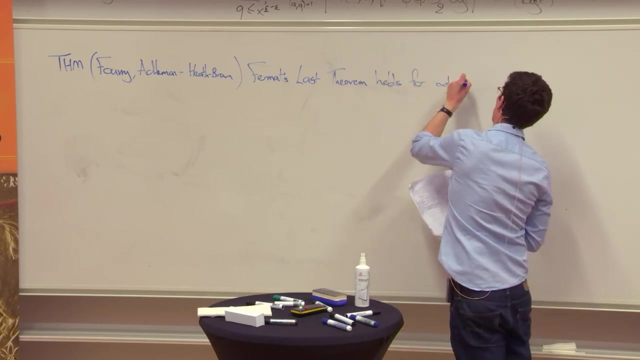 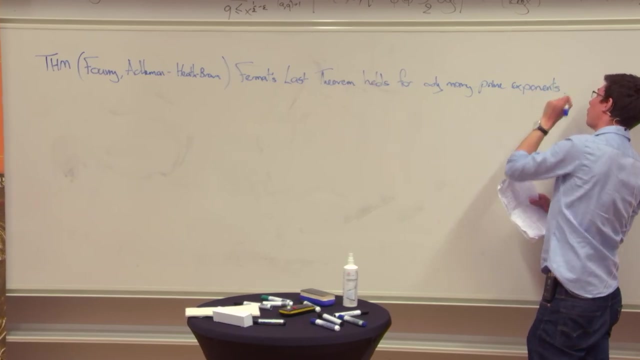 is a result of Fruvery and then independently Adelman and Heath-Brown, which says that Fermat's Last Theorem holds for infinitely many prime exponents. So obviously this isn't such an impressive result once you know Andrew Wiles' result. 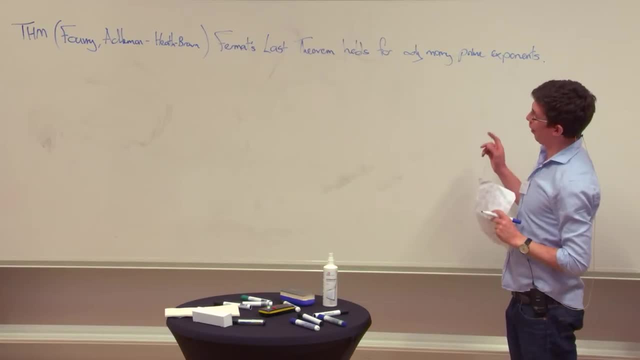 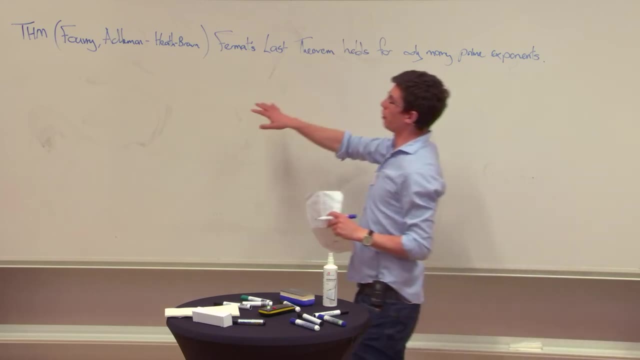 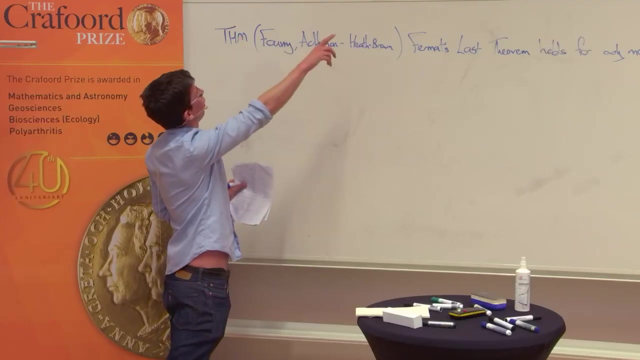 that Fermat's Last Theorem holds for every exponent, But this predated Andrew Wiles' result by more than a decade And the key technical information that went into this result of Adelman, Heath-Brown and Fruvery was a result on primes and arithmetic progressions. 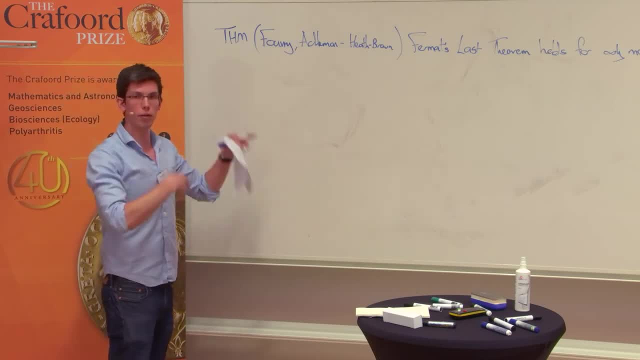 sort of morally of the shape of this BFI result. So there's quite a slightly different formulation, but it was these ideas about primes and arithmetic progressions to modulate beyond X one-half and beyond this square root barrier, that was the key. So that's the arithmetic input. 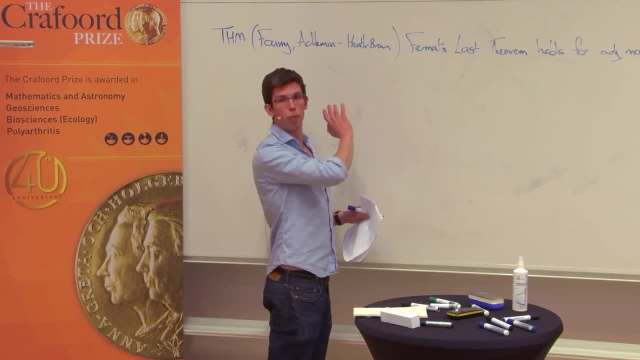 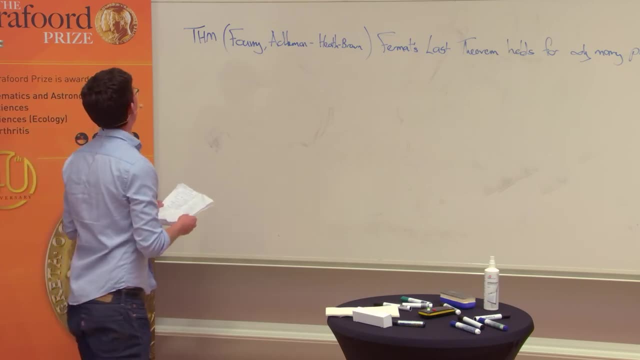 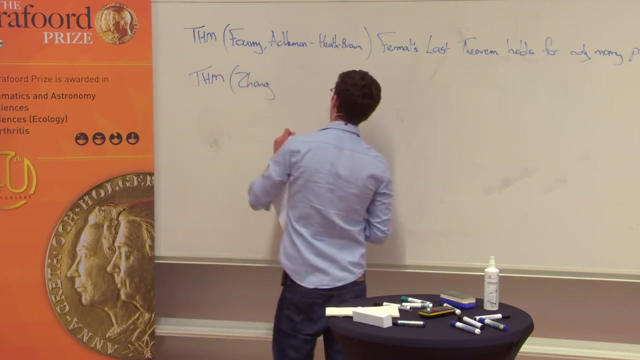 And, at least at the time, that was maybe the strongest result in the direction of Fermat's Last Theorem by some metric- Maybe I've already mentioned the results of Yiteng Zhang from 2013,- that there exists boundary gaps between them. 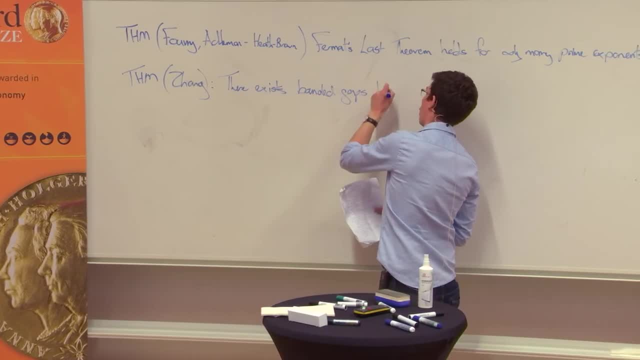 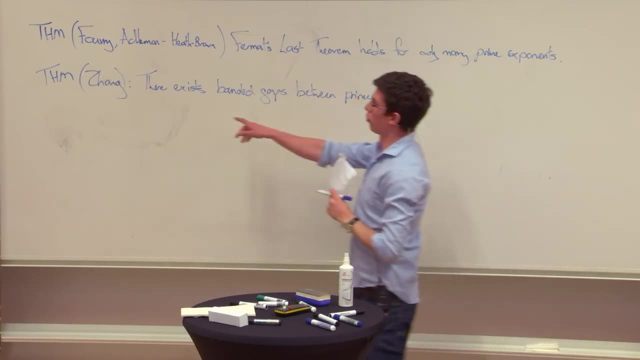 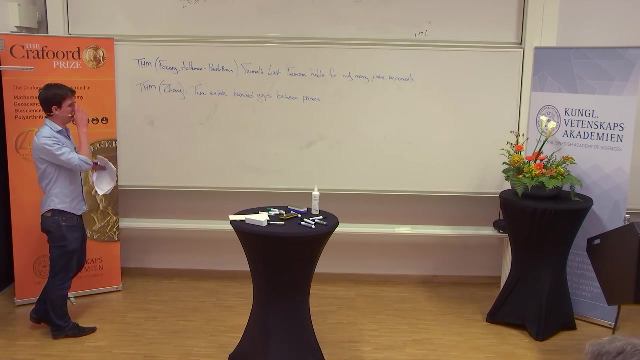 So there's a lot of information about boundary gaps between primes, And Zhang's result was very much inspired and followed much of the spirit of this result of Bombier-Friedland-Rovanić. Obviously, he had to come up with several impressive innovations on his own. 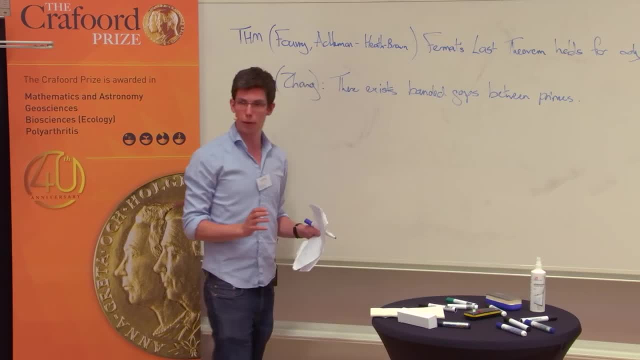 But the key input for Zhang's result about boundary gaps between primes was not a result in Siv Mathis at all, but it was a result of the fact that in fact, he was able to find a solution to the boundary gap between primes. 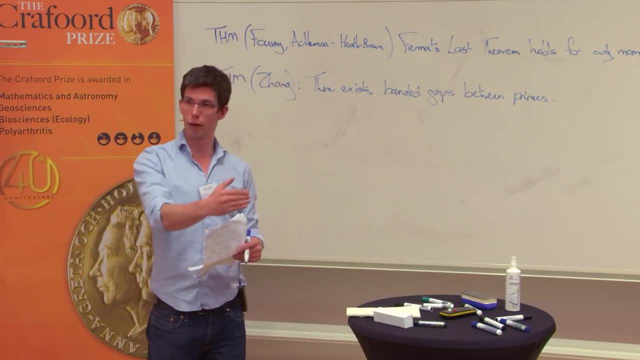 and the square root of X, And that's what I'm going to talk about in a little bit. But the key input for Zhang's result is all about a technical extension of the Bombier-Vinogradov Theorem to moduli which was slightly bigger. 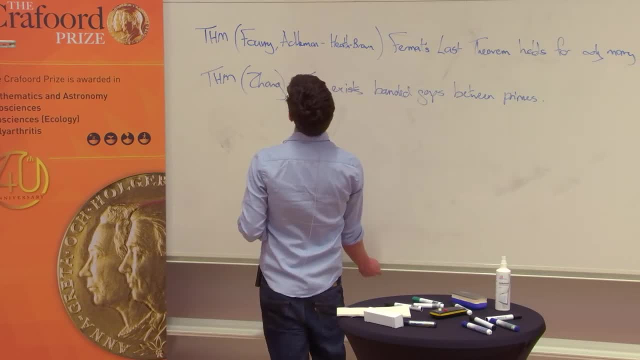 than the square root of X and slightly beyond the stream hypothesis range, And so, just as so, this result is kind of for someone who likes primes and likes Siv Mathis and things, I find this a very pleasing result, as both as a practical tool- 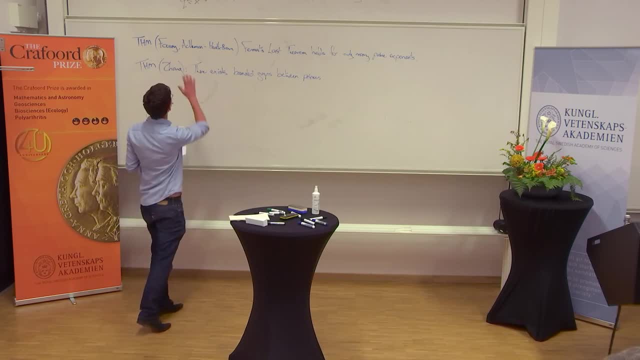 and also as a psychological tool to be able to find a solution to this problem. So that's what I'm going to talk about at the end of this talk. Thank you very much. You will find that this is not the case. It's actually a really good 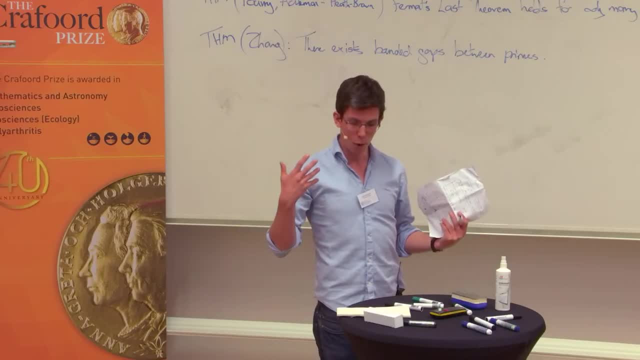 example of what you can do in this sense, of how you can make these kinds of transformations with the Bombier-Vinogradov Theorem by using a very practical tool and also as a psychological tool that we can actually prove results that from the point of view, 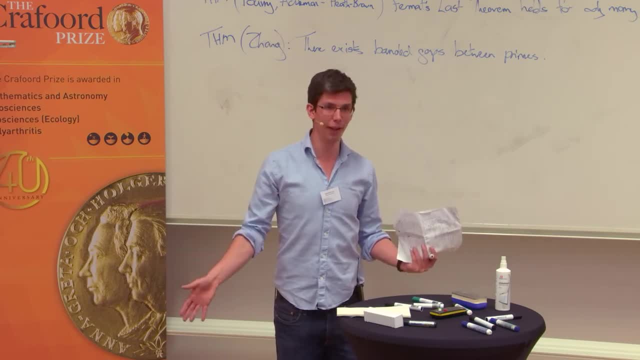 of Siv Mathis, the Bombier-Vinogradov Theorem is as good as the generalised dream hypothesis and there's very little to be gained if you assume that the generalised dream hypothesis from the point of view of Siv Mathis only. 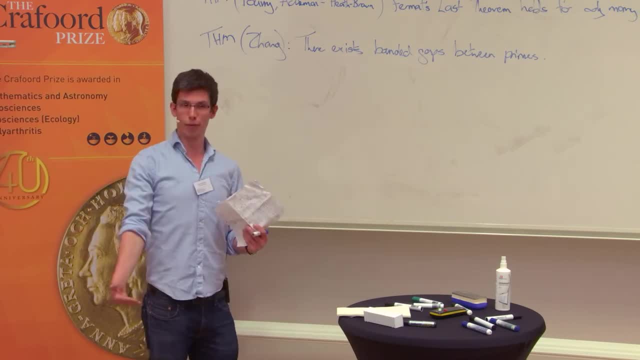 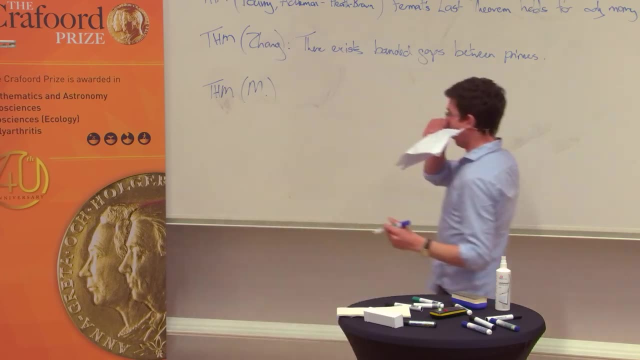 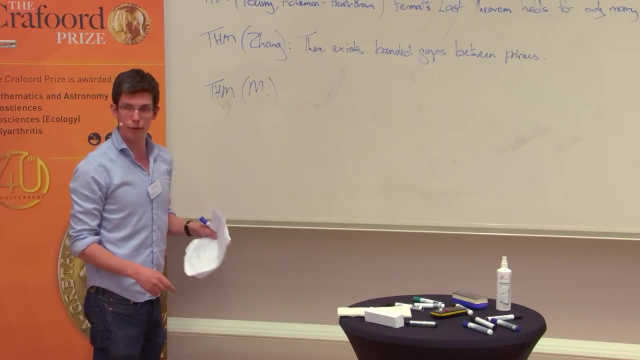 But actually with these sorts of results you can actually go beyond the generalised dream hypothesis and you can prove stronger results. finish with just a very recent project that I completed, maybe last year, which was trying to improve upon these sorts of technical results about primes and arithmetic regressions, largely. 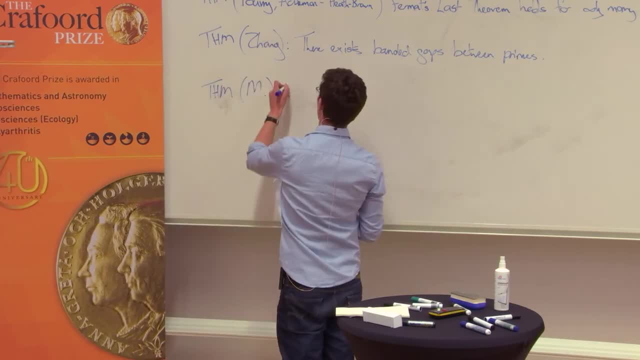 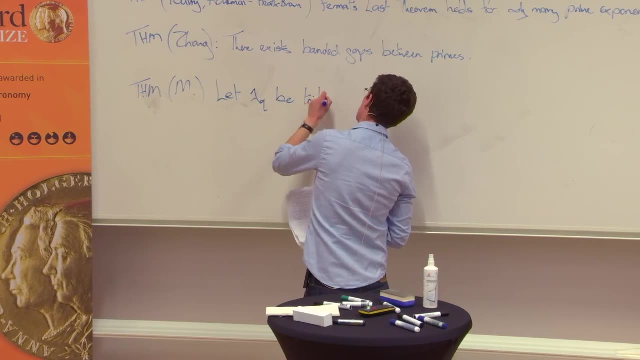 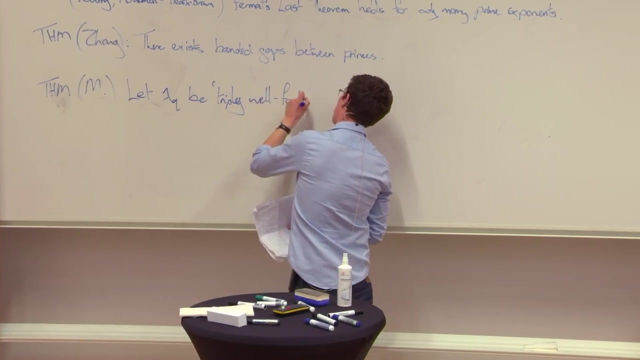 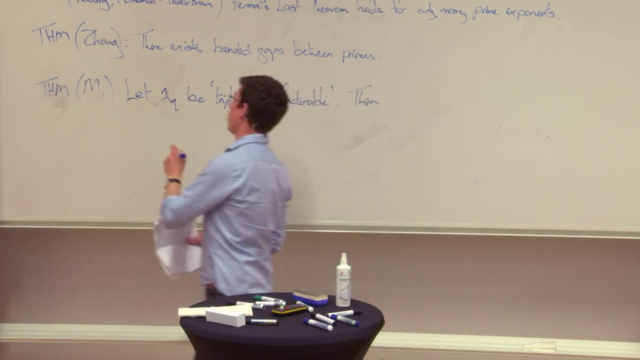 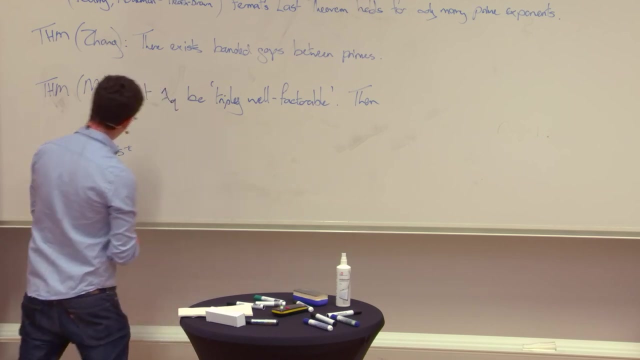 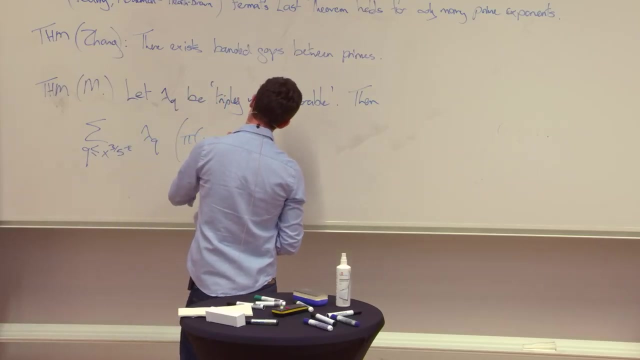 beyond x one-half. I have some slightly different technical condition which I am going to call triply well factorable. Then we can get a similar result, but now improving on the four-sevenths to a three-fifths. Okay. 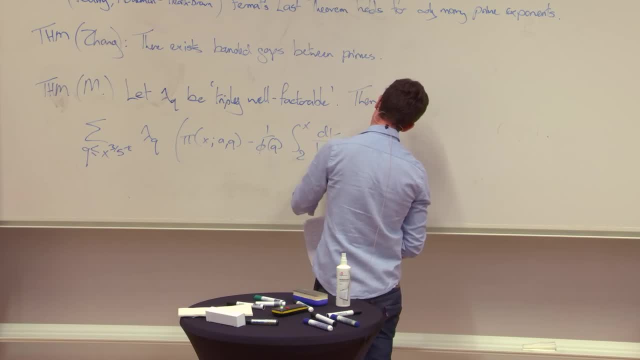 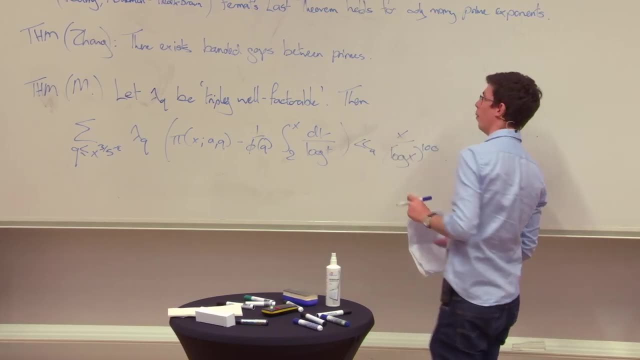 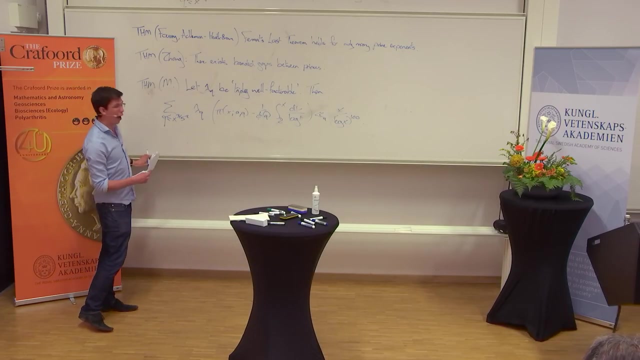 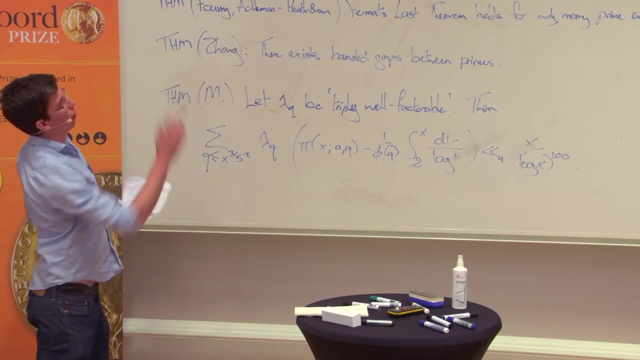 Okay, Okay, Okay, Um Again, if we are playing this quantitative game as to how far beyond the generalised dream hypothesis can you go, then hope in your dreams, if you believe this conjecture, you should be able to get a constant, arbitrarily closed to one: The generalised dream hypothesis. 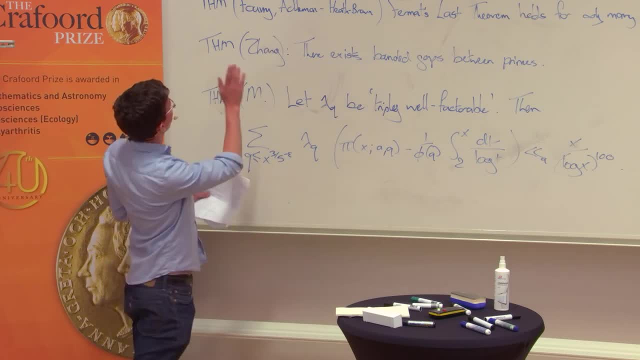 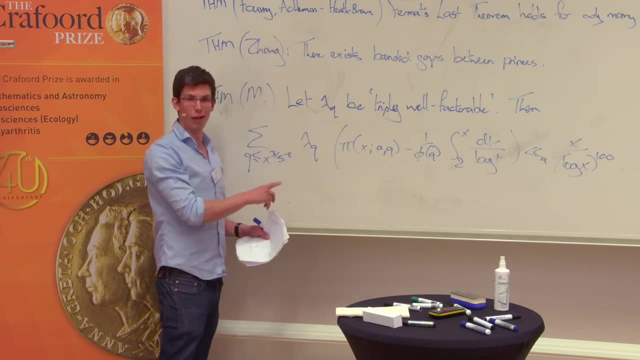 Bombier-Vinogrado theorem corresponds to one-half. There's this proof of concept, getting four-sevenths, and my result now gets us up to three-fifths, which is the current world record. So I don't know if this means we're 20% beyond.